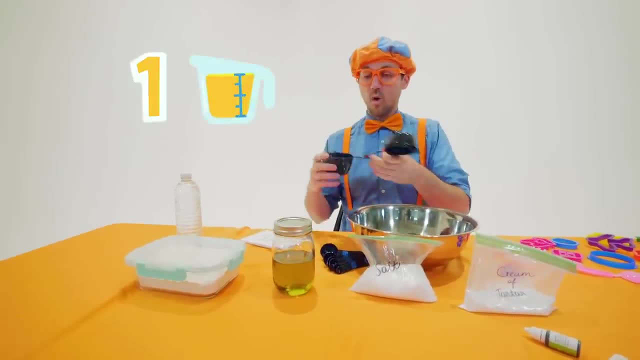 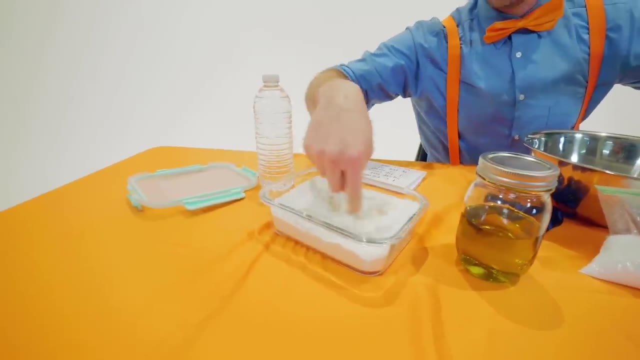 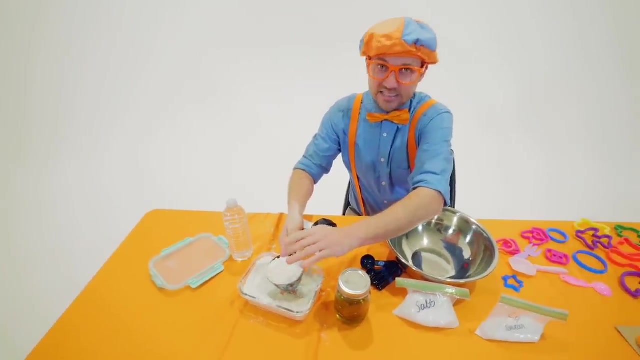 Yeah, all right. So first we need to start with one cup of flour. Whoa, okay, Let's open this up. There we go, And it doesn't need to be exact. Yeah, that is one cup of flour. 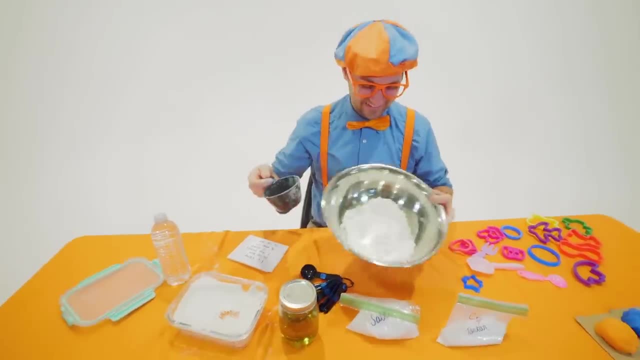 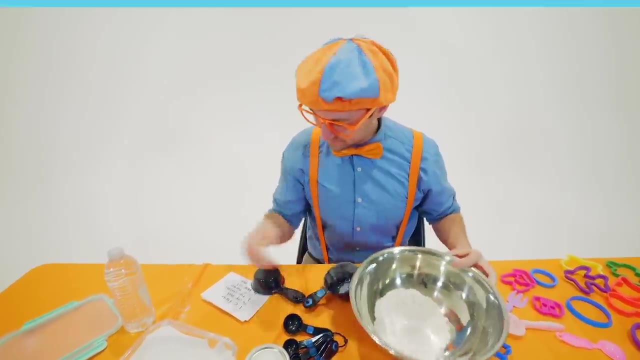 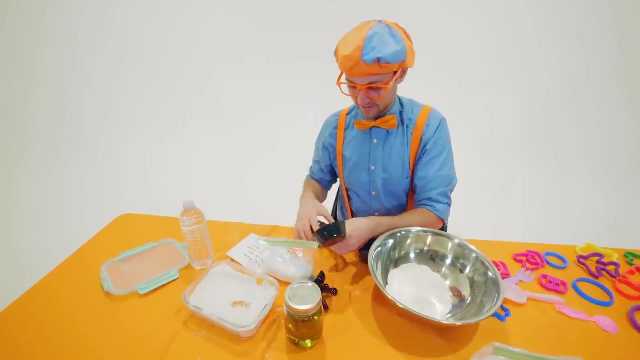 Here we go. Whoa, wow, That is. That is a great base for the clay we're making. Okay, all right, Let's see One quarter cup of salt. All right, It is definitely already getting really messy. Okay, one quarter cup. 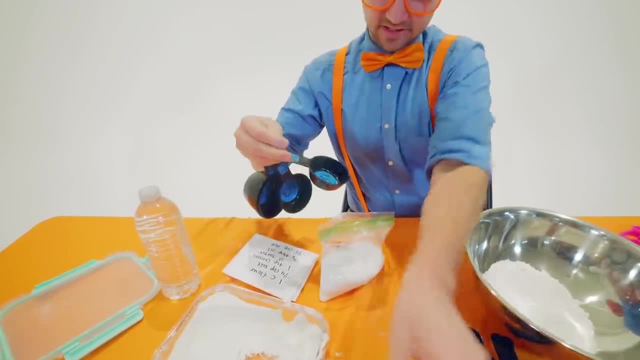 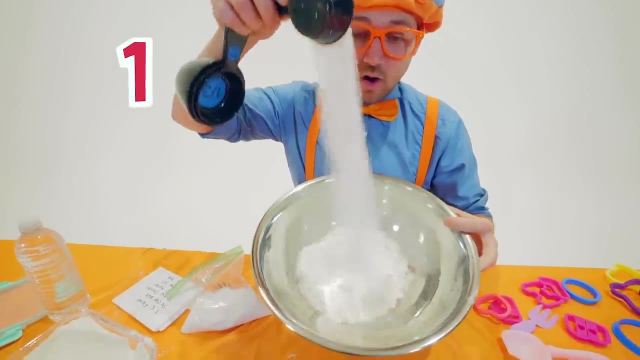 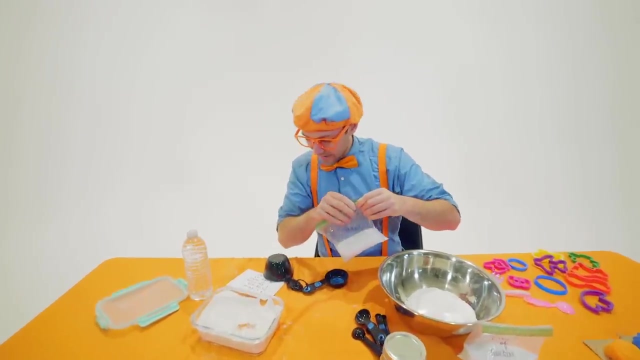 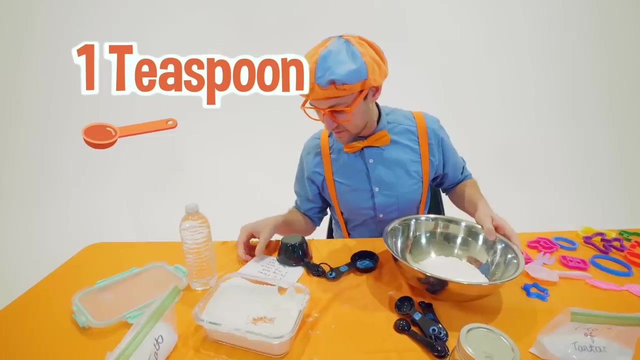 And then we need to grab some salt. Here we go: Perfect Ready, Three, two, one, Whoa Perfect. All right, Okay, let me zip this back up, Yeah, And then we need one teaspoon of cream of tartar. 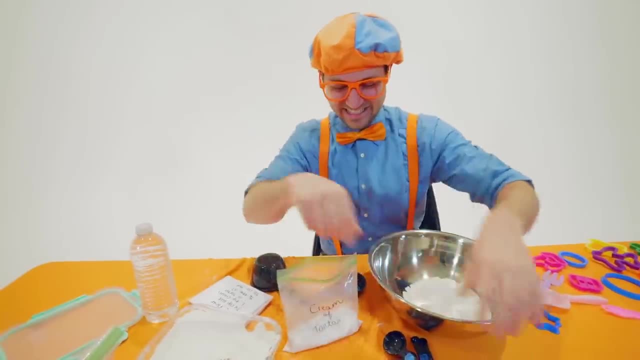 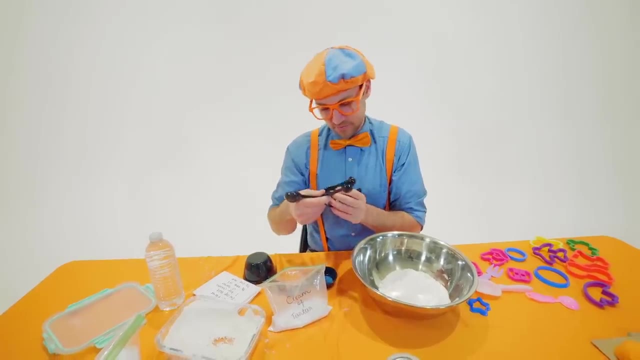 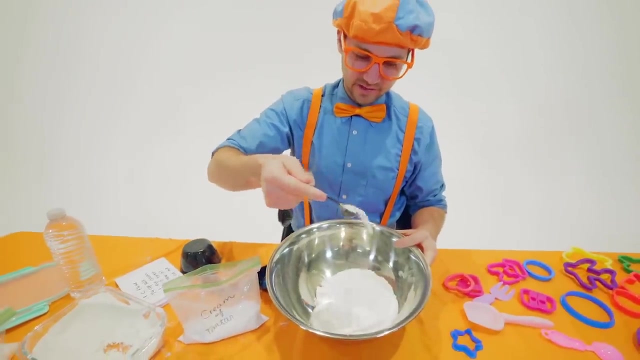 What a silly name. That's so fun. Cream of tartar: One teaspoon- Oh, there's so many. Okay, Here we go. Here's one, Here we go, And we're going to mix all this up in a little bit. 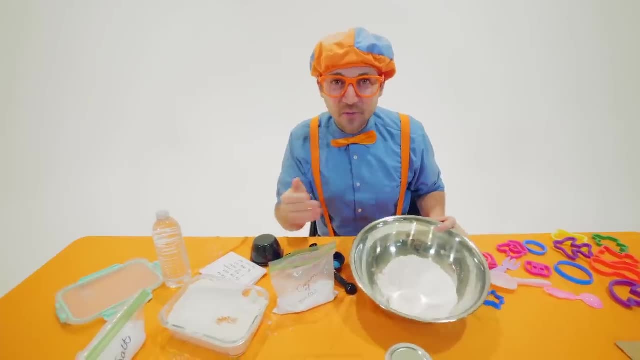 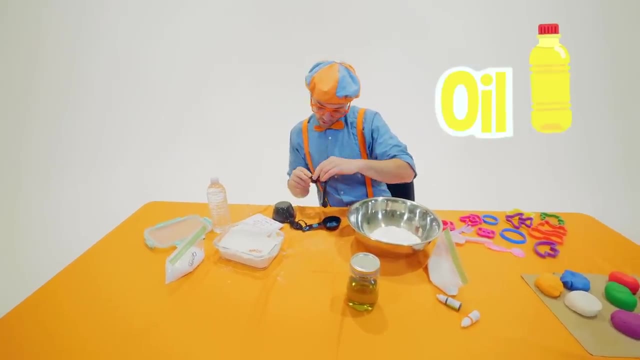 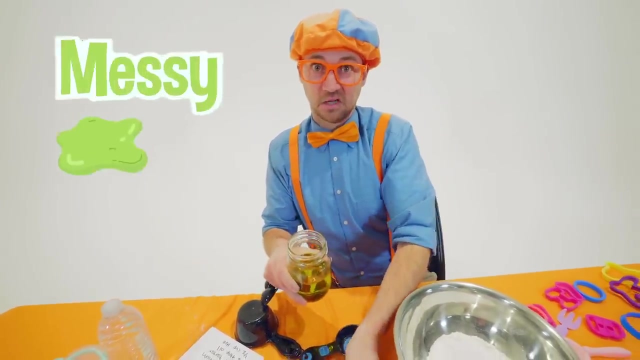 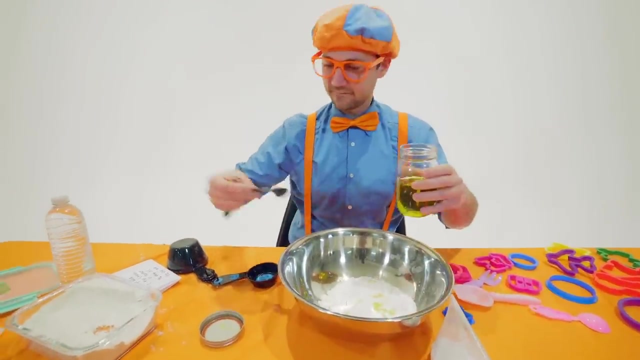 But for now, let's pour all the ingredients in here. Then we have a half a tablespoon of oil. Okay, Whoa, This is where it might get a little messy. Okay, Perfect, All right, Put the lid back on, just so it does not spill. 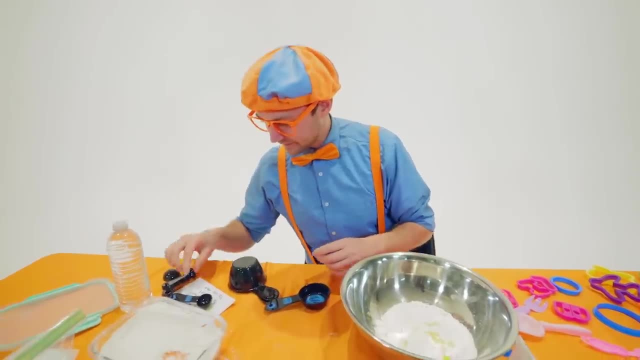 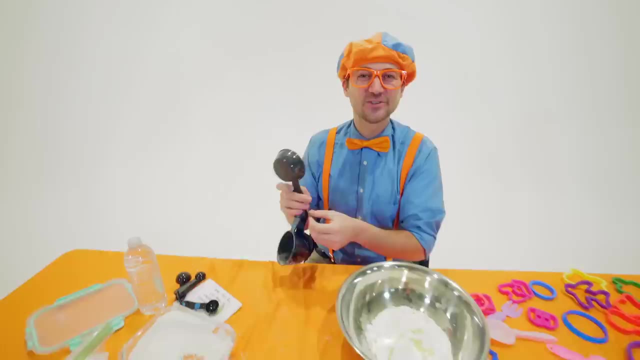 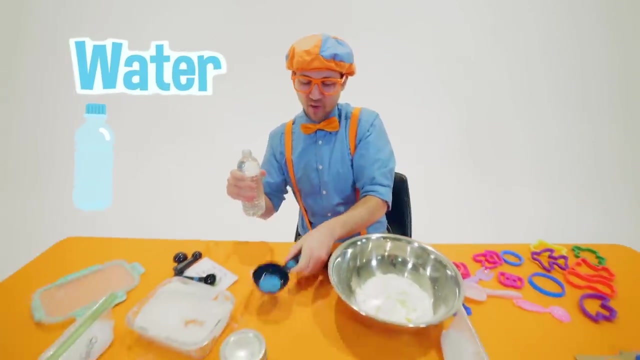 That would be bad news. berry, Okay. And then we have a half cup of H2O. Do you know what H2O stands for? Yeah, Water, I love water. All right, And then we have a half of a cup. 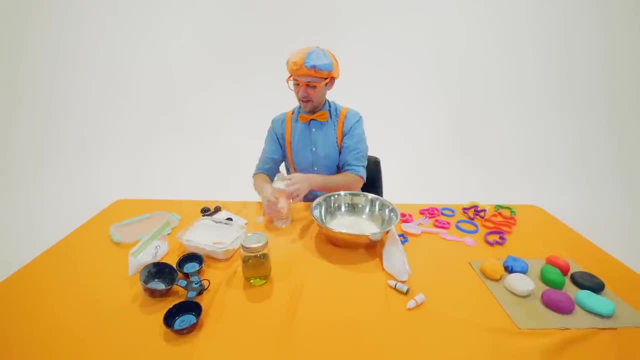 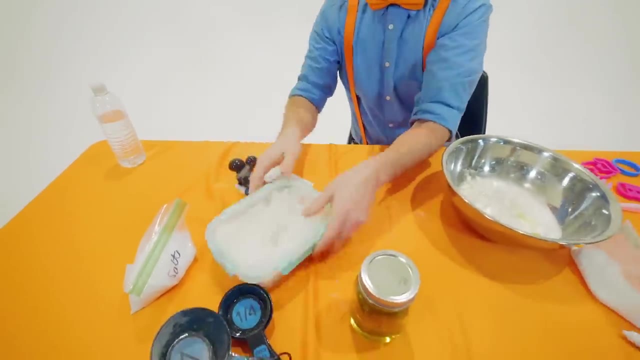 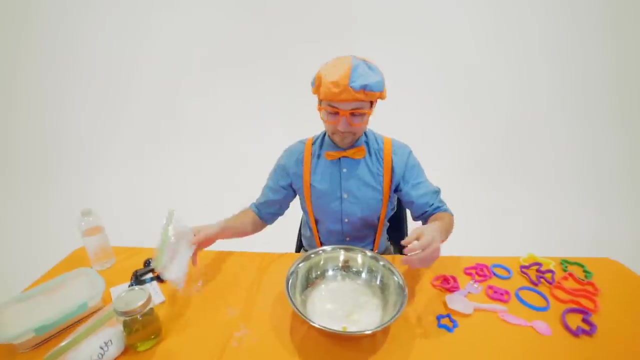 Perfect, All right. Oh, hey look, I forgot to close up the flour. You should probably do that. All right, Let's push all that stuff to the side, because now we're ready to mix it up, But what we need to do is put in some color. 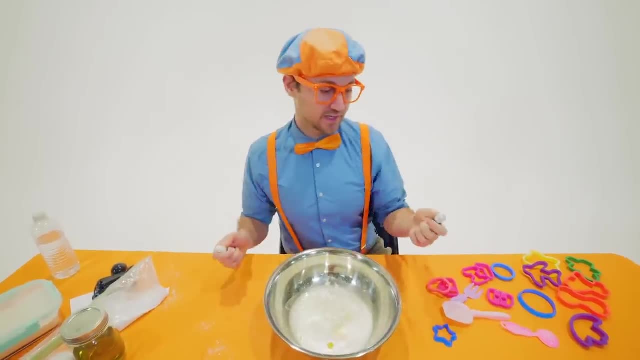 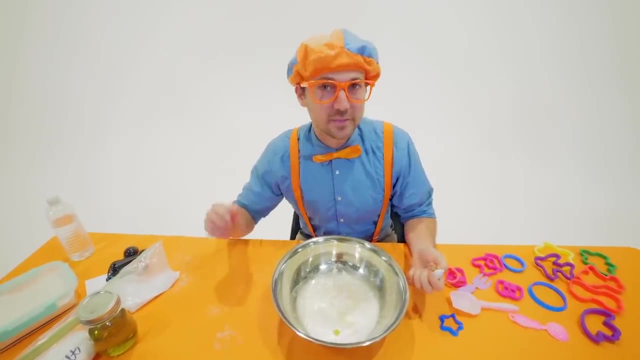 And you can make any color you want. But what we're going to do, although we already have a green color, I think we should make another green, But this one will be a little bit lighter. So let's open this up, Add some green. 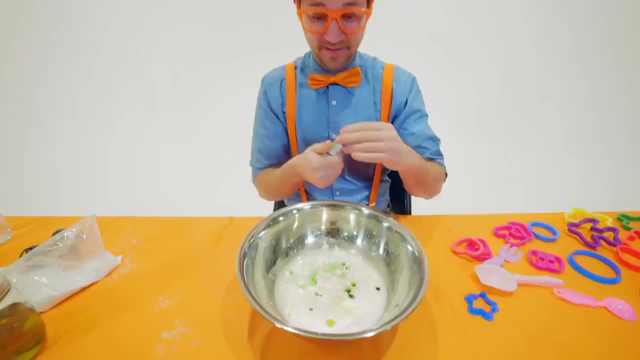 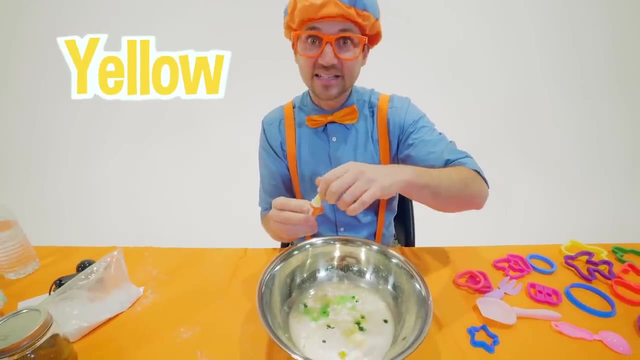 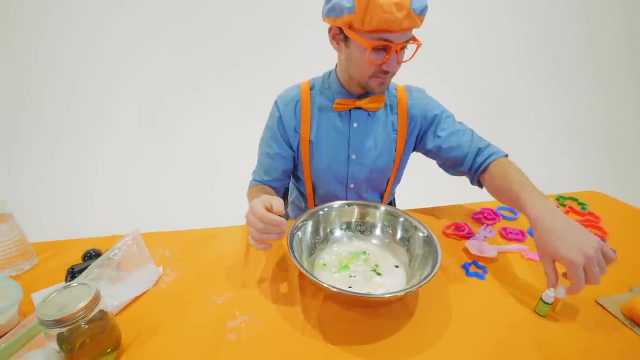 I don't know how much to add, but that seems like quite a bit. And then also I'm going to add a little bit of yellow. Yeah, It's going to make it more of a bright green. Let's close that up. 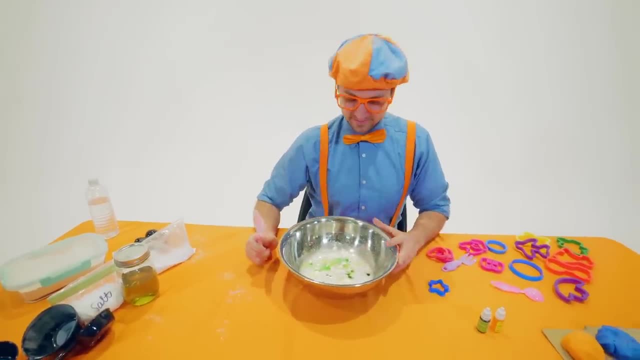 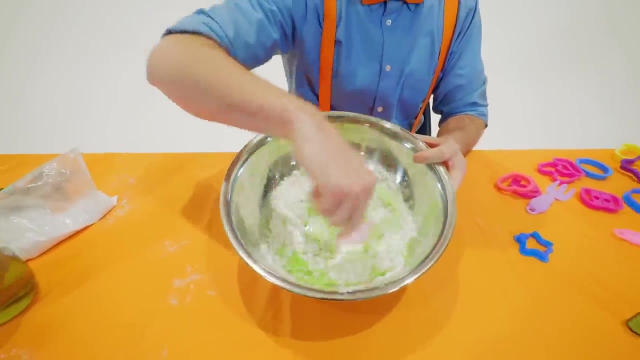 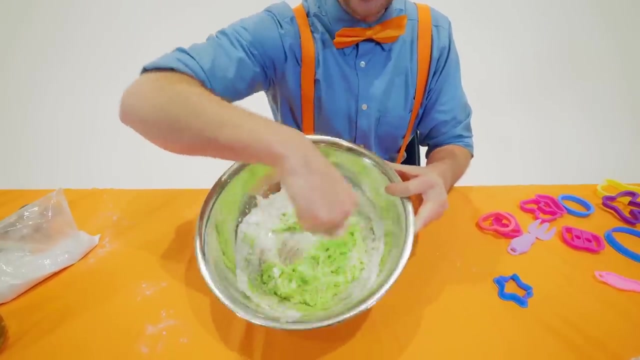 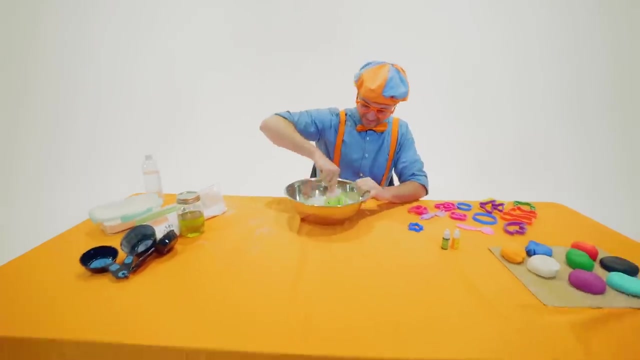 Whoa. That was a fun recipe to make, But now I got to mix it up. Whoa. It's looking so good. Wow, You see it. Whoa. All right, Let me keep mixing it up, Whoa. 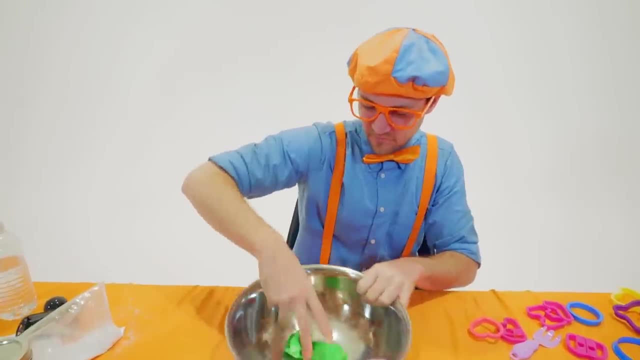 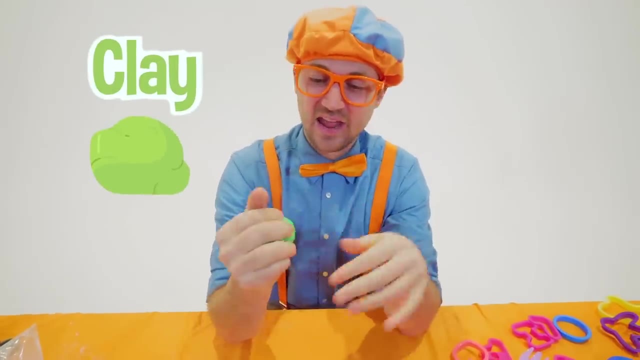 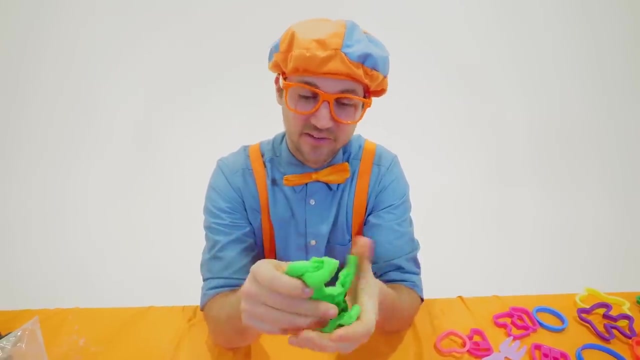 Yeah, We did it. Whoa, Check it out. Wow, Whoa, Homemade clay. Wow, What a pretty green color. we made Good job. I wonder what color you're going to make at home for your first color. So now, what you can do with this. it's so much fun. 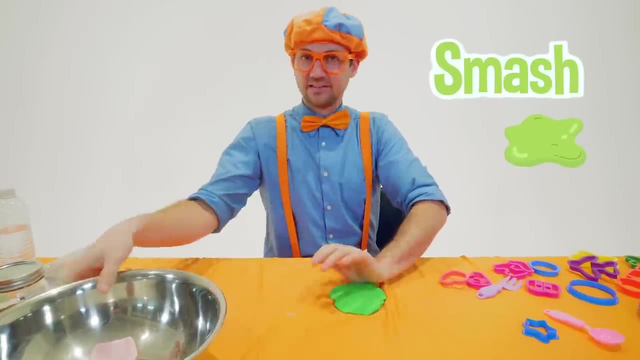 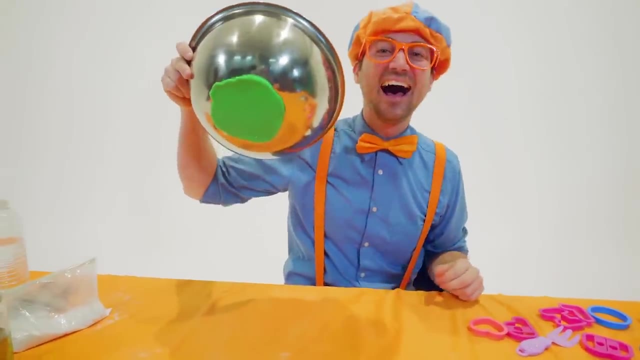 You can actually smash it flat. Watch this trick. Where'd it go? Oh, that's silly. Okay, Let's peel it off. Wow, Perfect. And then now you can use these. Yeah, They're like cookie cutters. 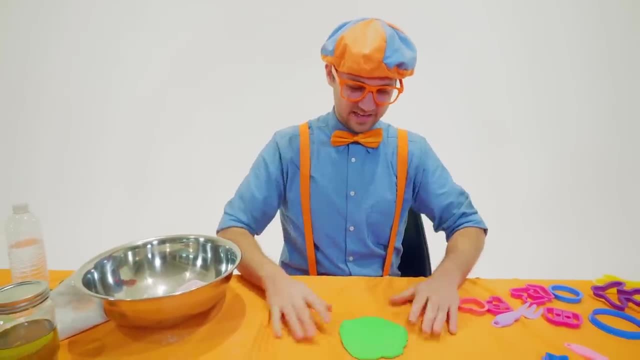 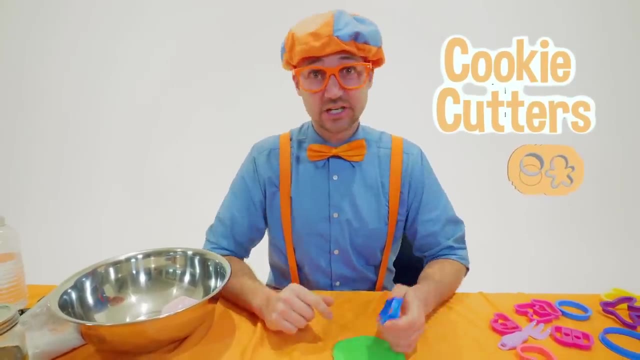 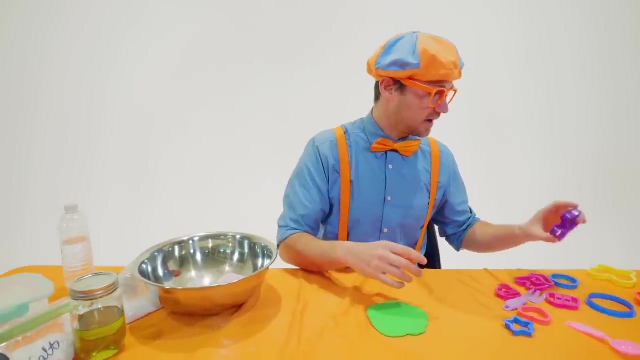 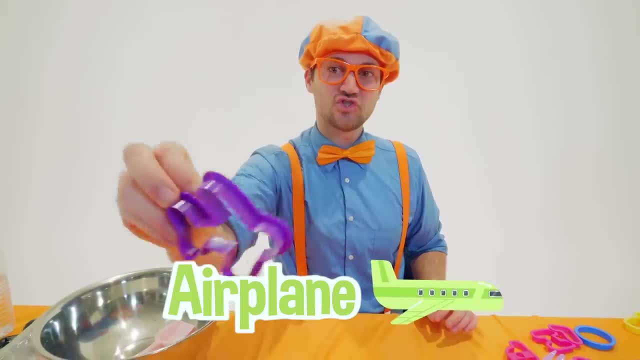 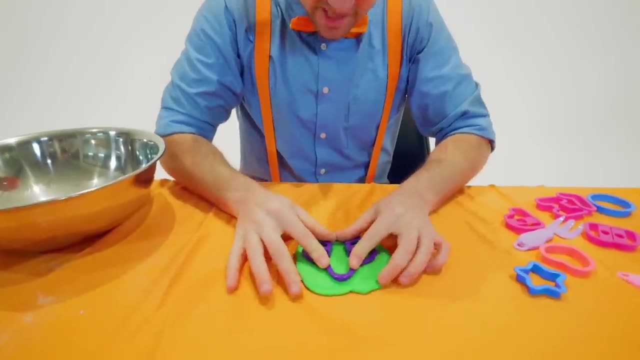 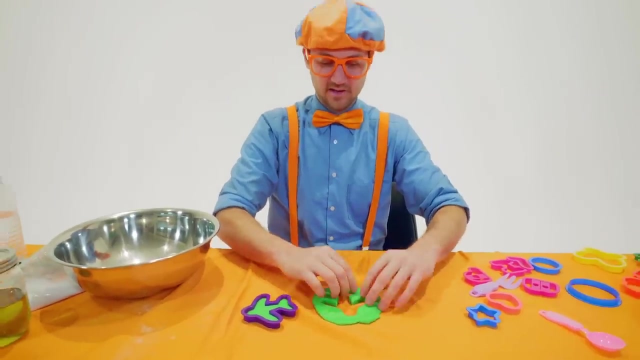 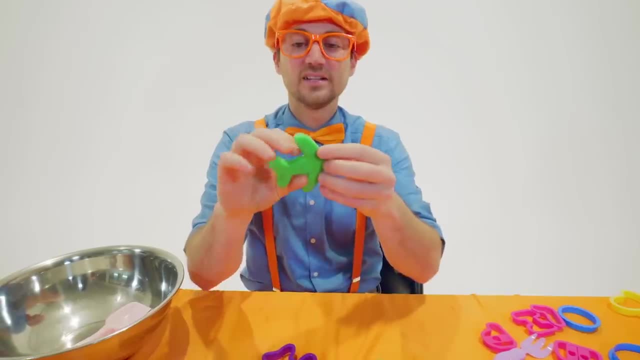 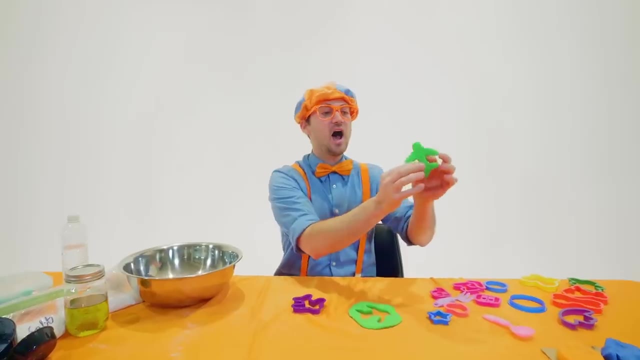 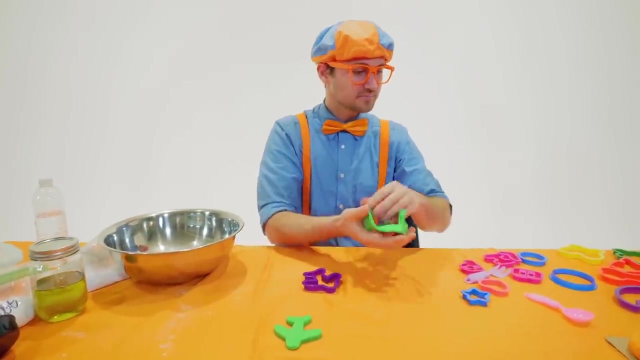 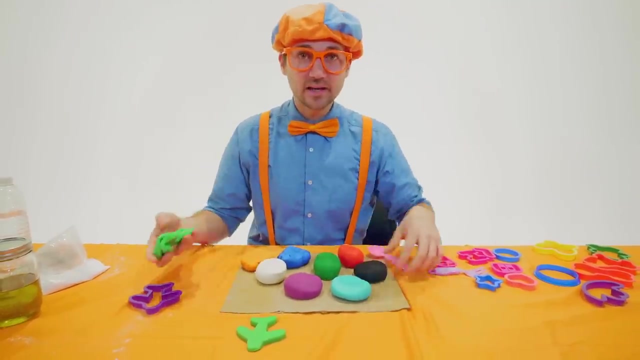 Wow, Look, Cut an airplane out, But first let's push it out of here. Wow, Yeah, Wow, okay, I'll put that airplane right there. Now let's bring all the colors that we have out, and then let's see what we can make together. 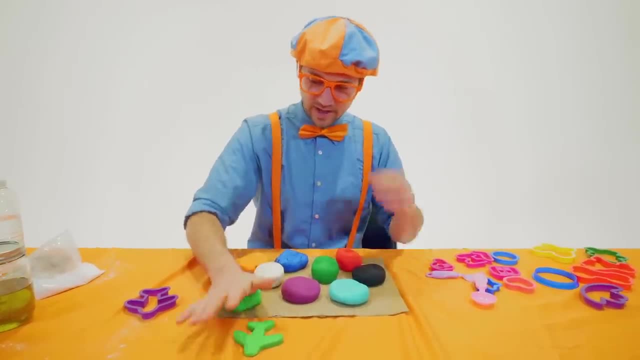 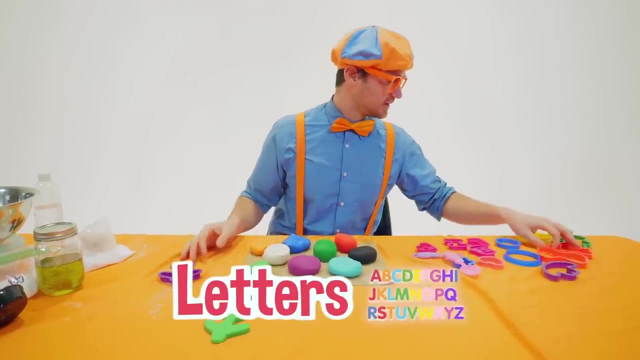 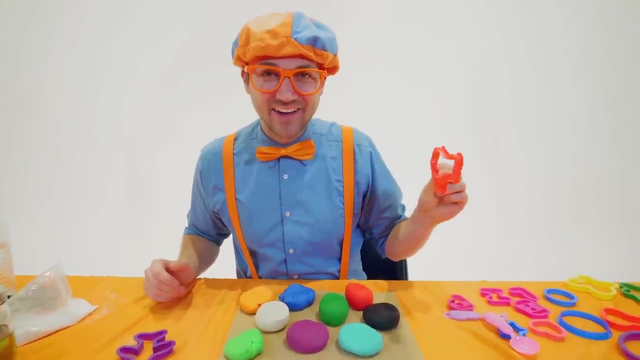 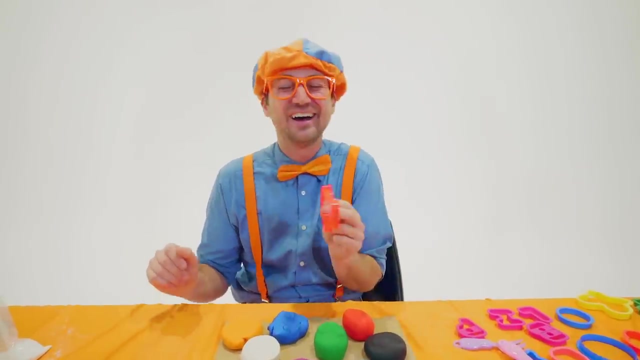 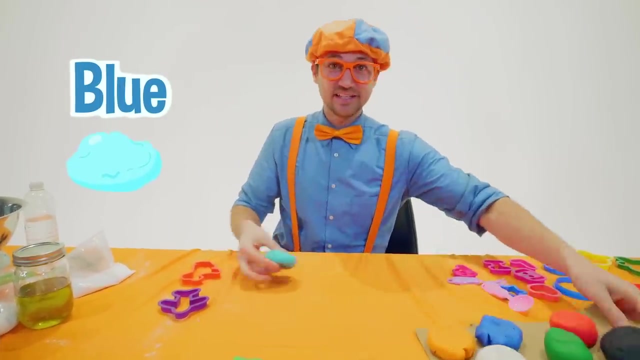 Okay, So let's put that green back and we have the airplane right there. What else? Oh, We have some letters. We have, whoo, a dog. Will you act like a dog with me ready? Dogs are so cute. Okay, let's make a blue dog. That sounds pretty silly, doesn't it? Okay, you know what to do. 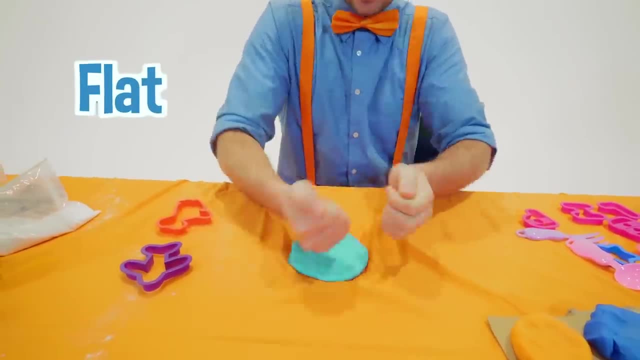 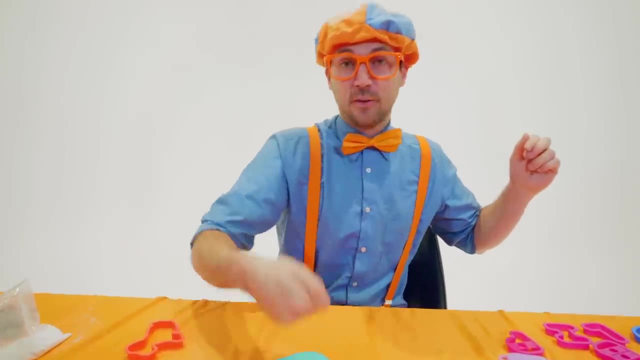 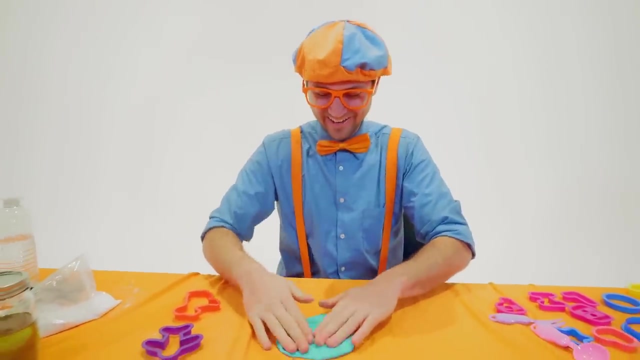 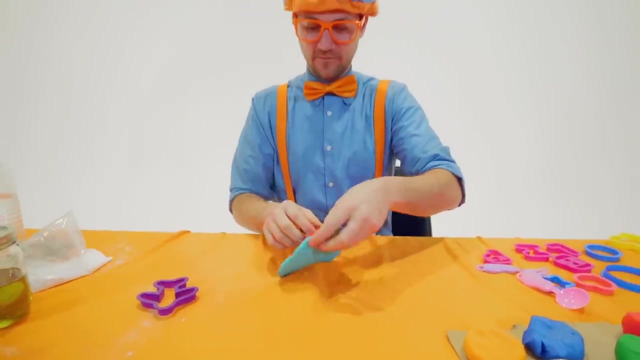 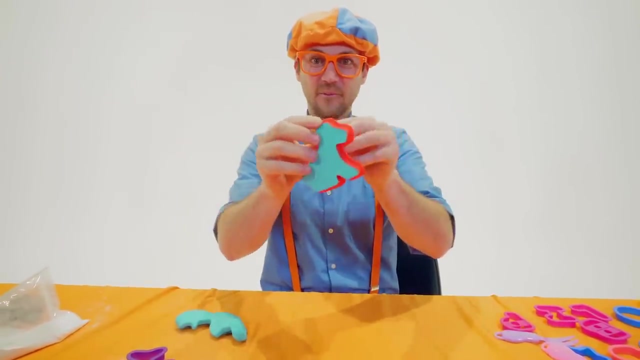 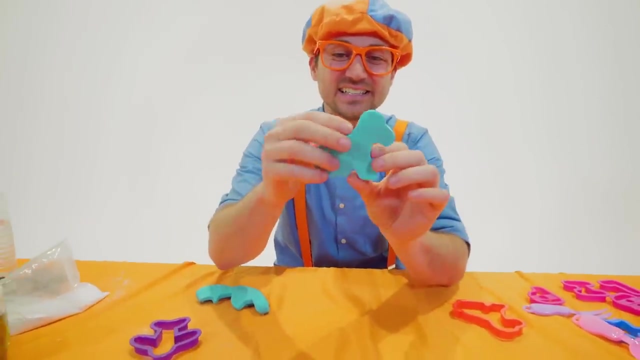 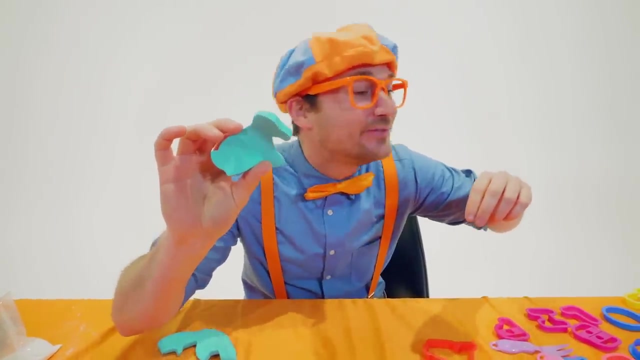 Smash out your clay nice and flat. Oh, Okay, here we go. all right, push it down, right. Whoa, look at that. Oh, Pull the sides away, Wow. and now? oh, Oh, What is that? Yeah, it's a little poochie. Okay, we'll save you, we'll put you right there, perfect. 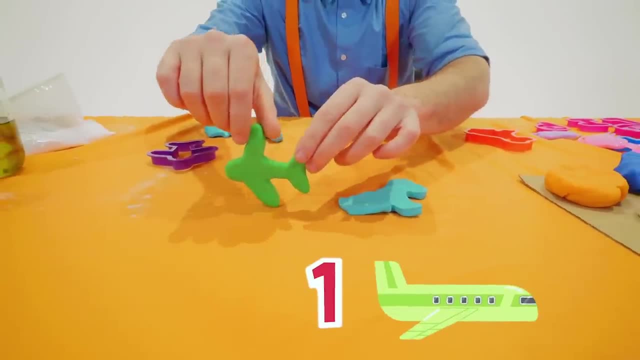 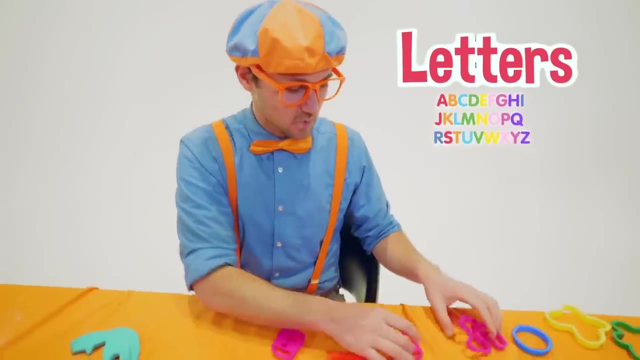 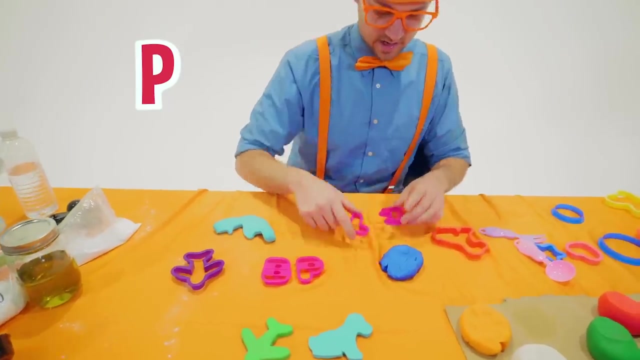 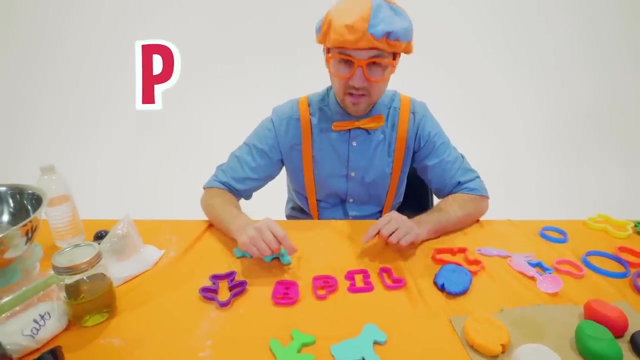 All right, one pooch and one airplane, huh Perfect. Oh Hey, I think we have some letters over here. We can spell something out. Okay, It looks like we have a B, a P, an I and L. Huh, a B, a P, an I and an L. 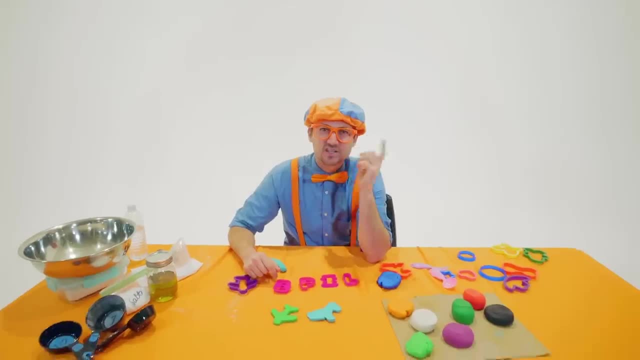 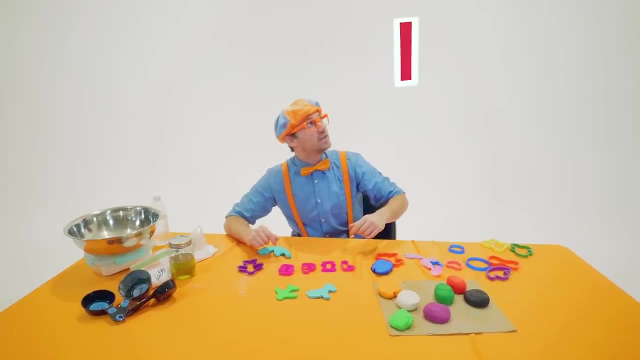 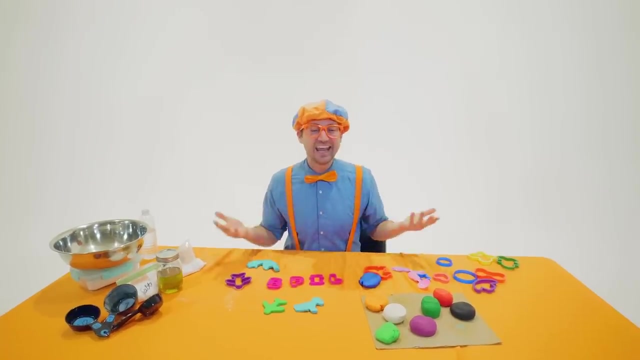 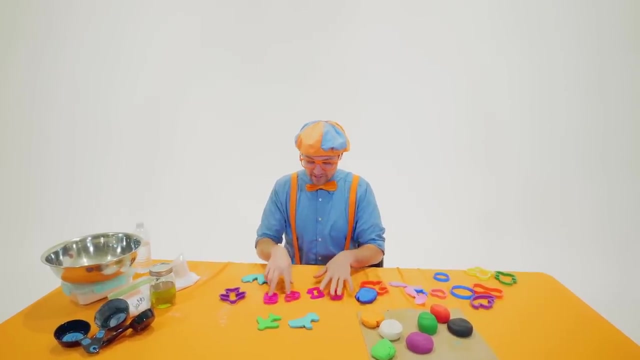 What word can you think that uses those letters of B, a, P, an, I and an L? hmm, oh, I know, Yeah, my name Blippi. Yeah, we can actually spell my whole name out, just with these four letters. See, we would go like this: We would use a, B, an, L and I. 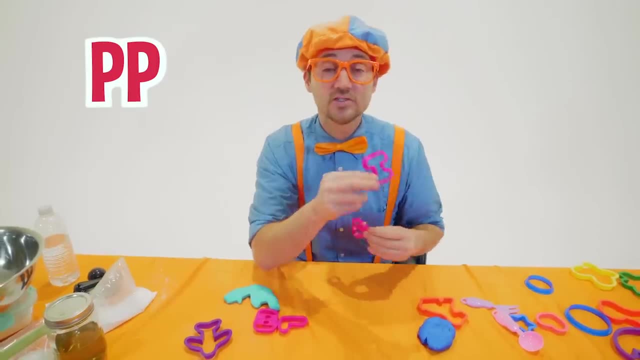 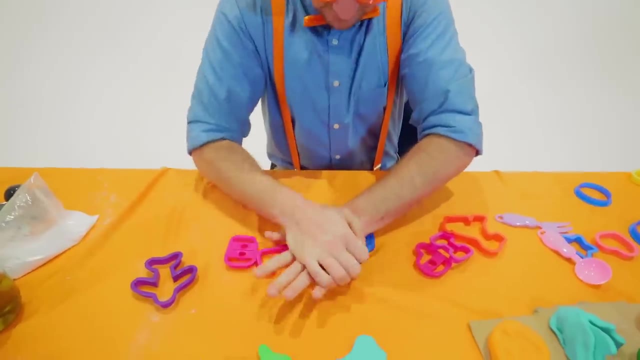 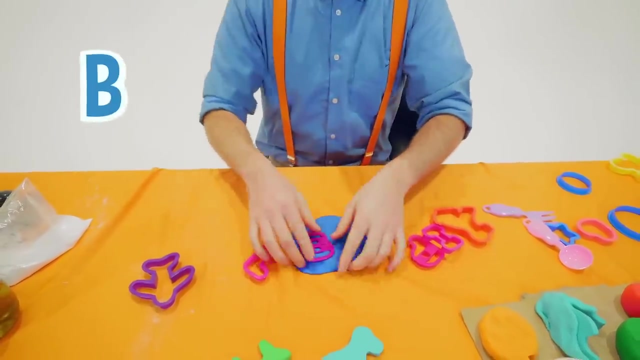 We would do two P's and then we would use another. I Perfect, All right, let's do that. All right, first we need some colors, So let's use- Let's use this blue color. Yeah, there we go. Let's do a B, right there. 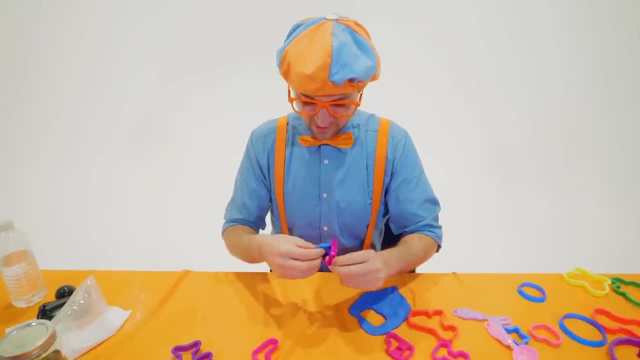 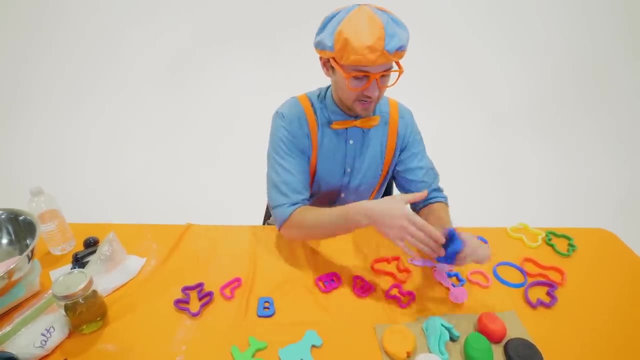 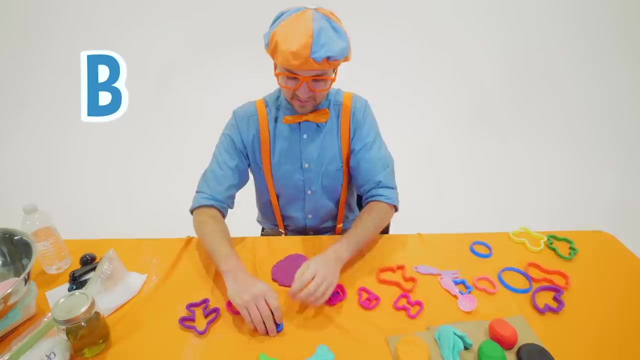 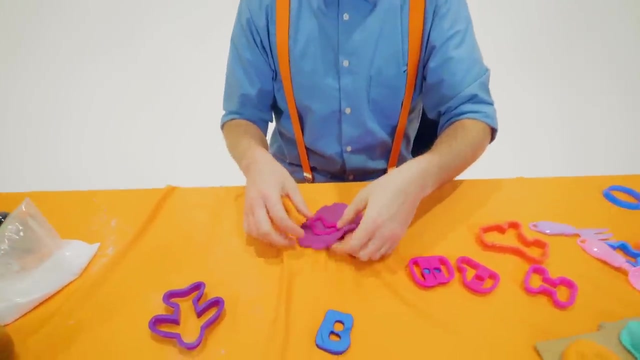 Perfect. Well, this is gonna be so cool. Yeah, and if you use some of this at home, maybe you could spell your name. Okay, let's use some purple, Alright, so we've got a blue B right here. Yeah, oh Okay. and then we have an L. 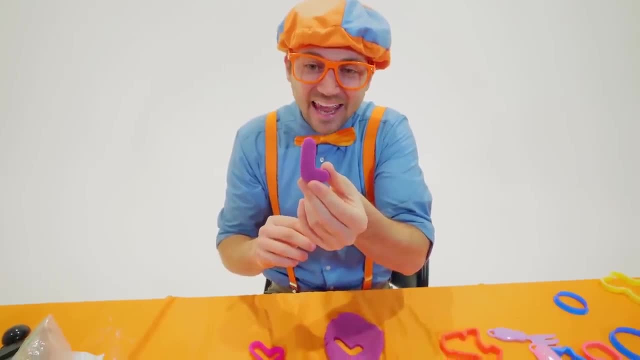 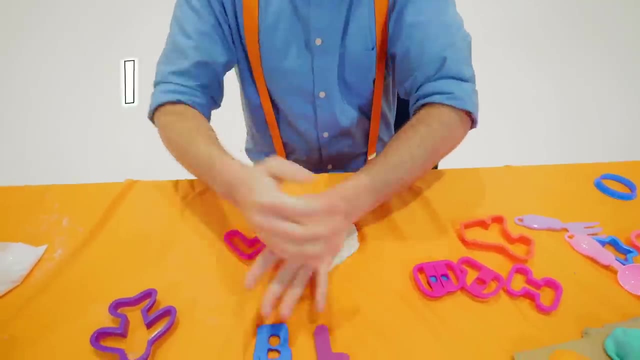 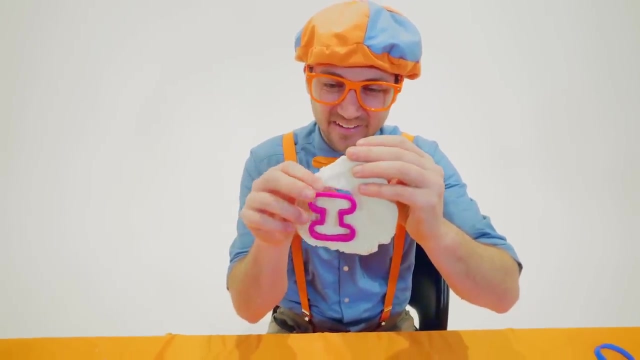 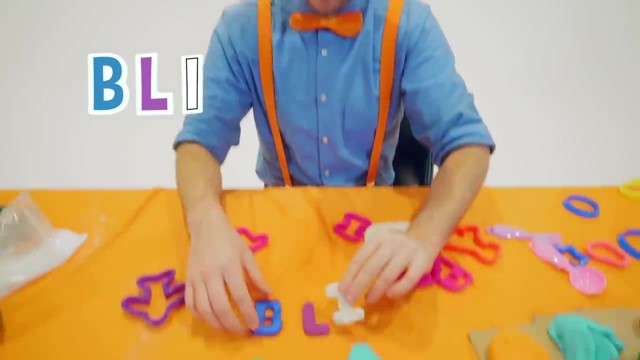 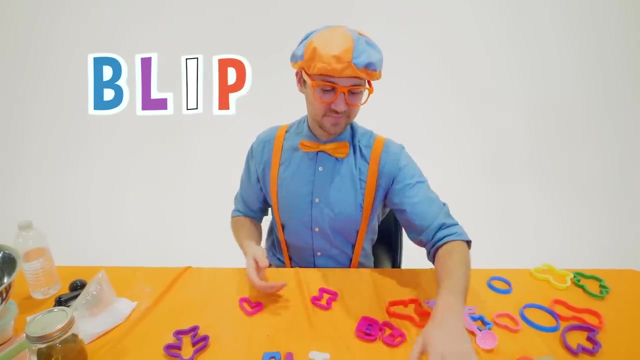 Alright, nice little L right there. Yeah, it's a B L, then we need an I. How does that look? yeah, whoa. Okay, B L I. Yeah, B L I. What's the next letter? Yeah, P, and there's two of them. Let's use one of my favorite two colors. 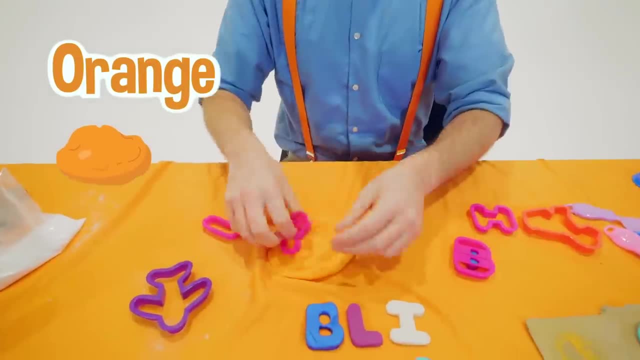 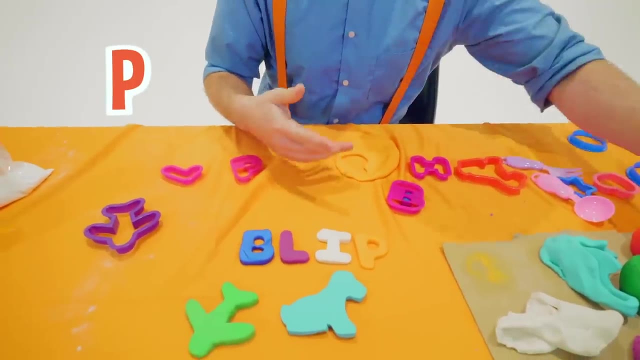 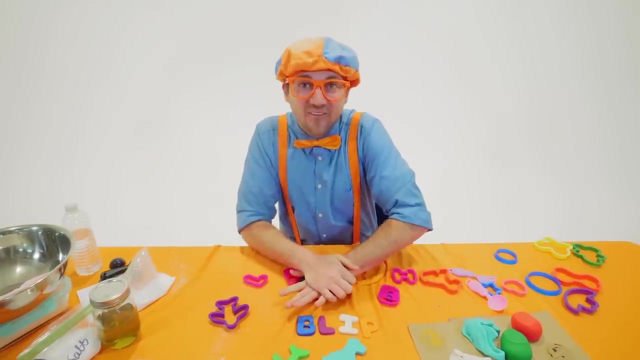 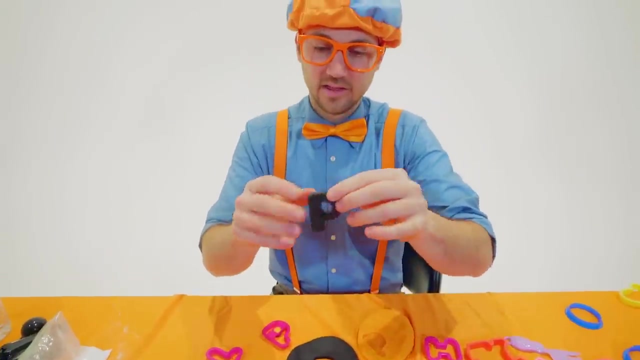 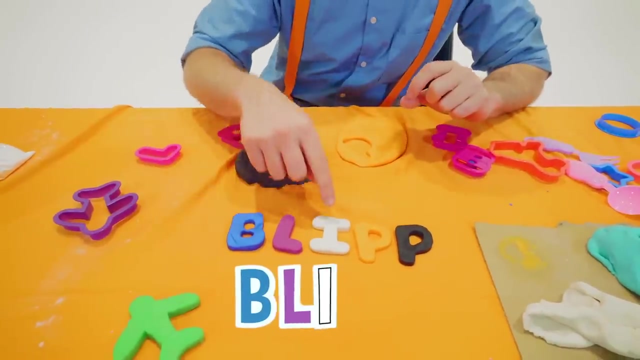 Yeah, the color orange. B L I P. we need another P, We'll use the color black. This is so much fun. It feels so cool on my hand. Ooh, another P, Yeah, so we got Here, we go, We got B L I P, P. 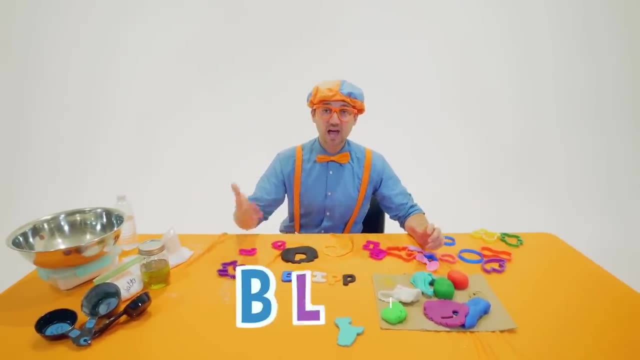 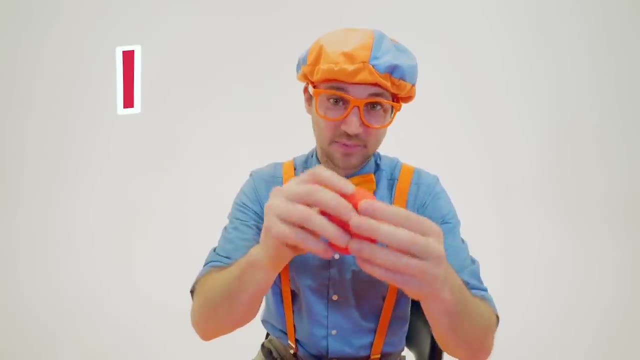 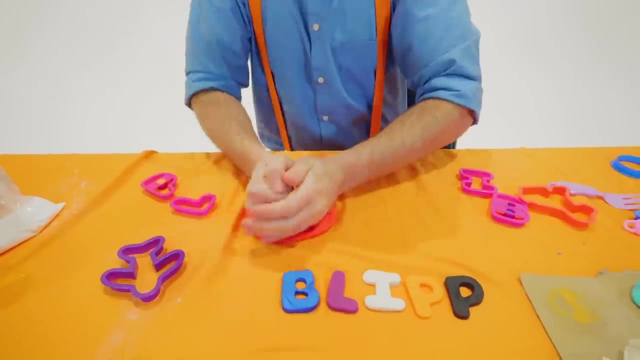 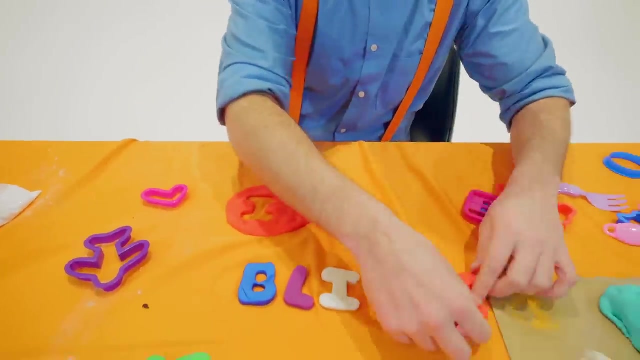 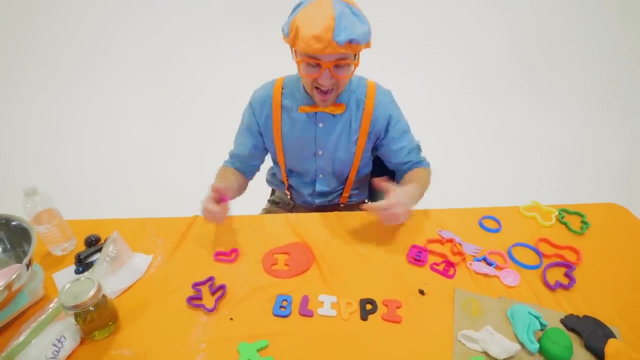 What's the next letter? B L I P P. Yeah, I, And let's use this bright red color. All right, here we go. B L I P P I. Here we go. Oh, How does that look? B L I P P I- Yeah, good job, All right. Okay, let's put these down here with the dog and the airplane. 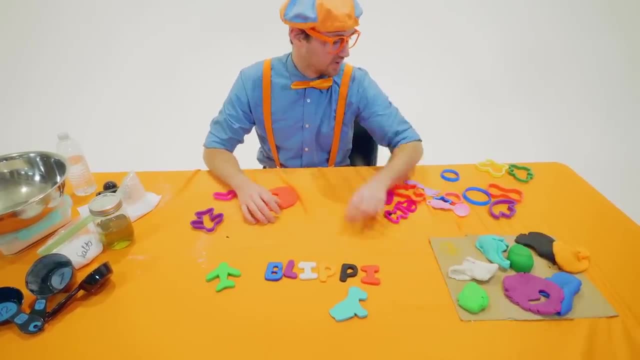 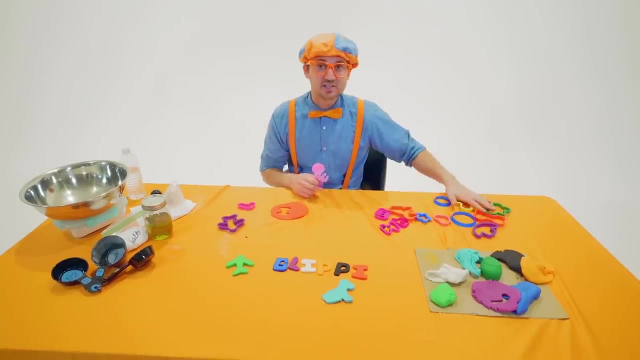 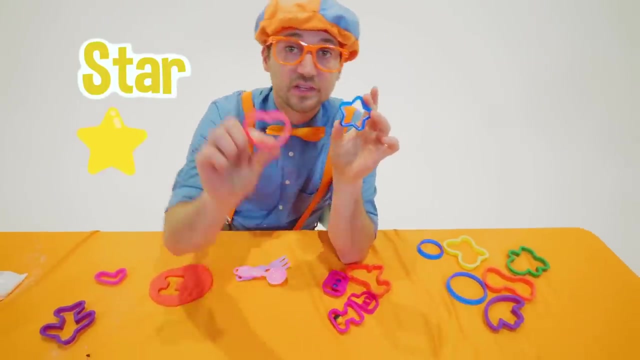 There we go, All right now. Now, let's make one more thing, Huh, Hey. well, since we have all these stencils and these cookie cutters, Yeah, you could actually use a lot of them. You can make a star, You can make a heart. 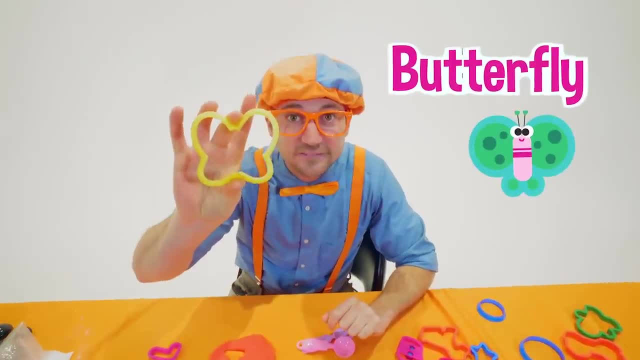 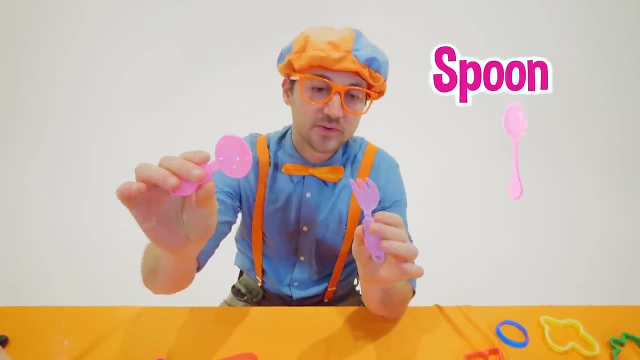 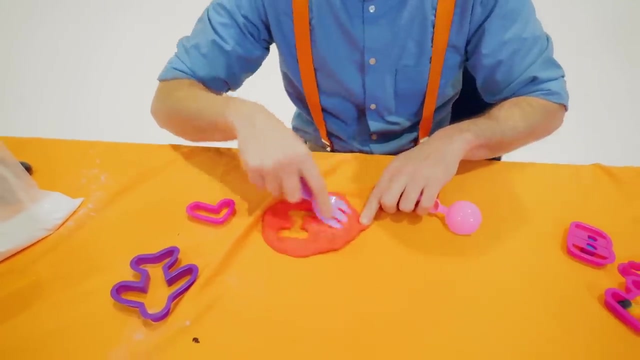 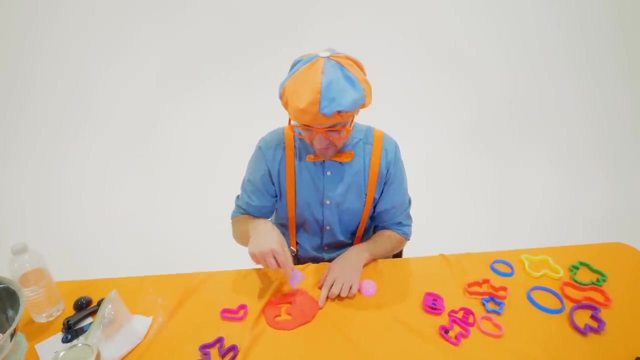 You could make a butterfly, Yeah. or you could use some other tools, Yeah, like the spoon or this fork and see, look at this, see, You can use the fork and, Yeah. act like you're in the garden. Yep, gotta make the soil nice and soft, so then you can plant some plants. 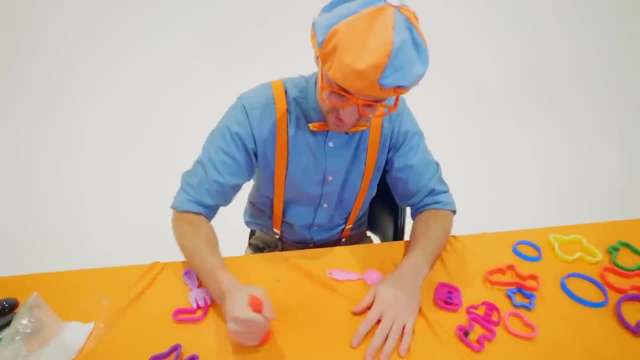 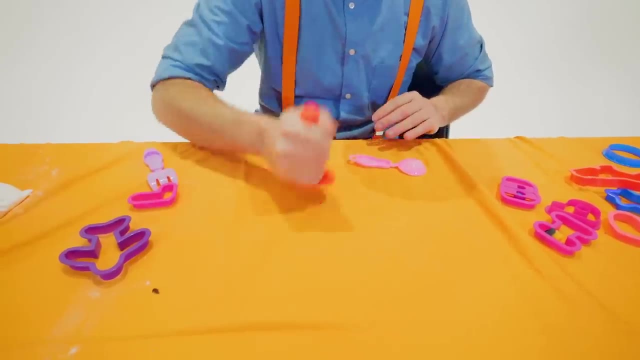 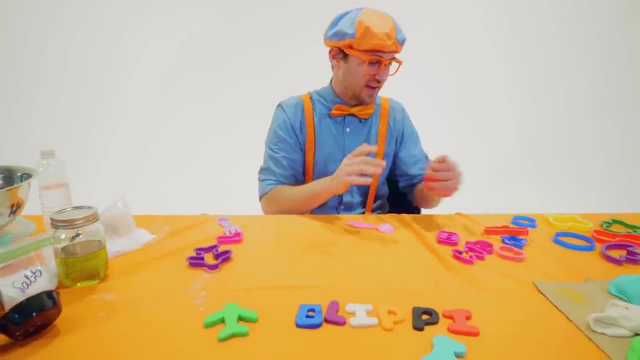 but I am definitely making a mess with all these small pieces. so this is a cool trick that I learned. see, you can actually pick up a lot of the pieces by Smashing it. Yeah, it's kind of fun, huh, oh, okay, but watch this. hey, we haven't used this color green yet, so if you take the 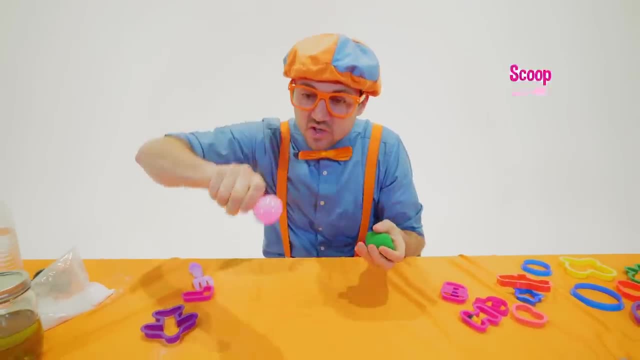 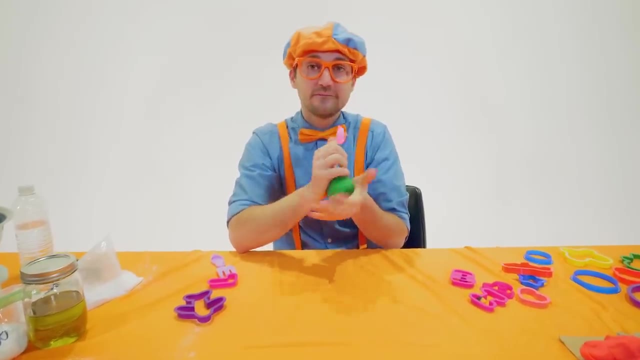 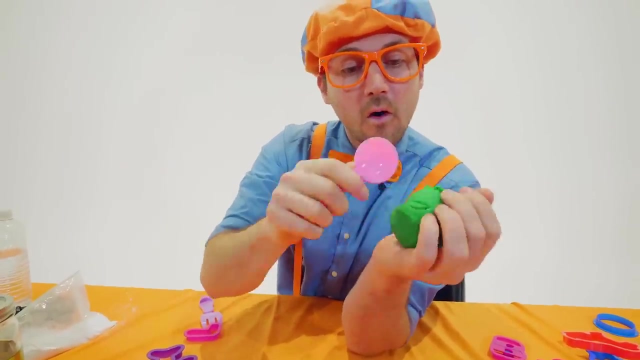 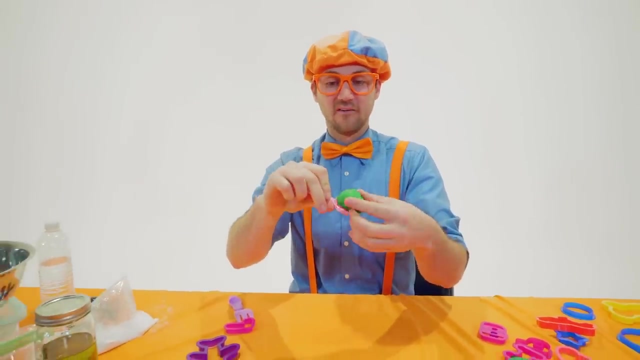 spoon and you scoop it. although it's a half of a circle, we go all the way around. you actually might be able to scoop a full circle. hey, let's try it ready. yeah, look, there we go. whoa, it's like a circle, Wow. and then you can put it in. 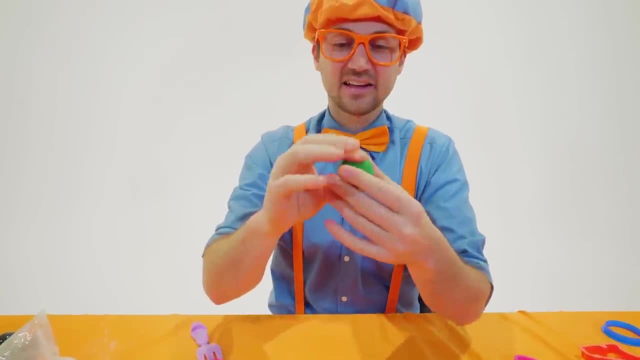 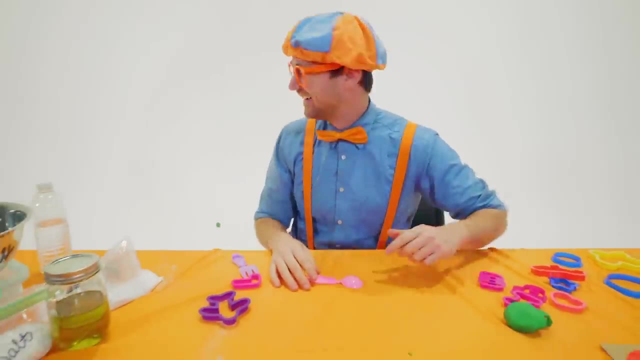 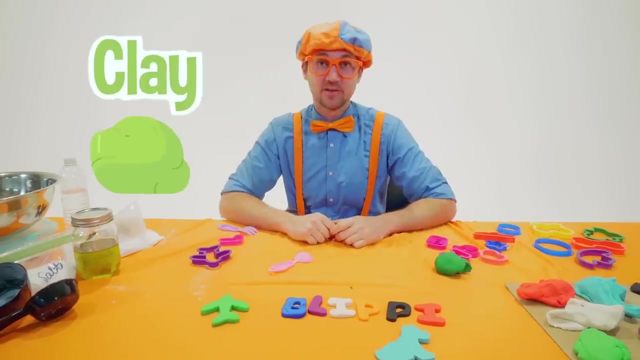 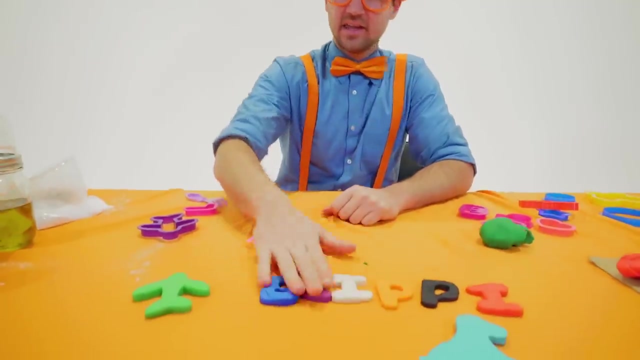 your hands roll it around. yeah, look, it's like a basketball. oh, that was silly. well, this has been so much fun. so much fun making this clay with you. did you have fun making clay with me? yeah, and it was really fun. yeah, using those cookie cutters to cut out some of the clay into an airplane. 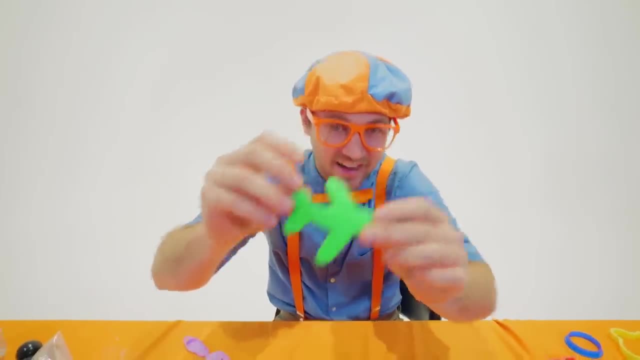 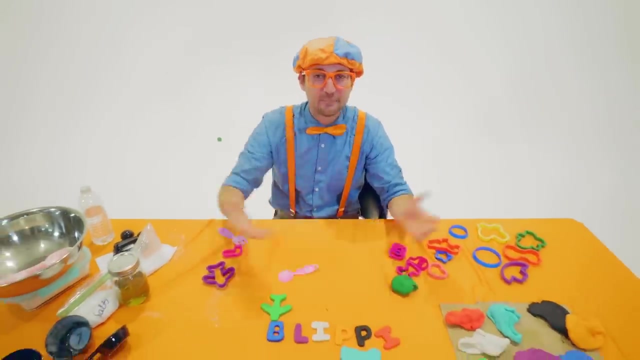 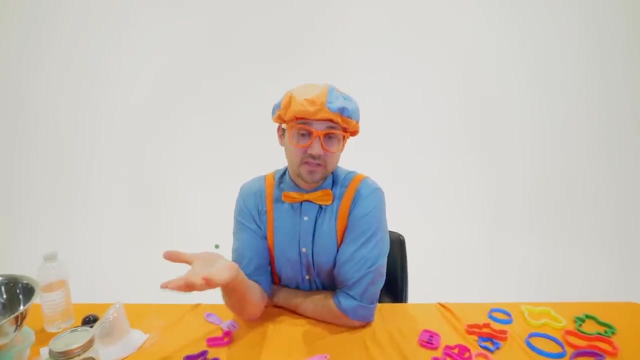 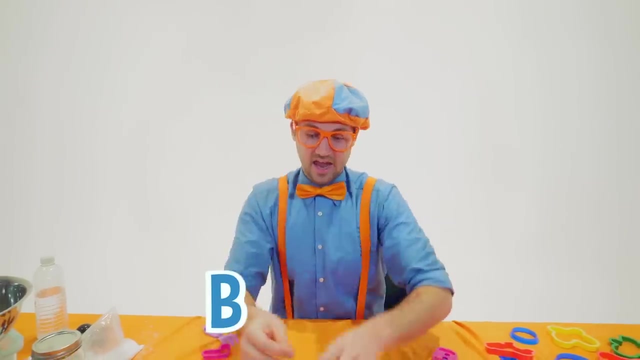 yeah, a doggy and my name flippy. well, this is the end of this video, but if you want to watch more of my videos, all you have to do is search for my name. will you spell my name with me ready? B Oh, L, I, P, P. 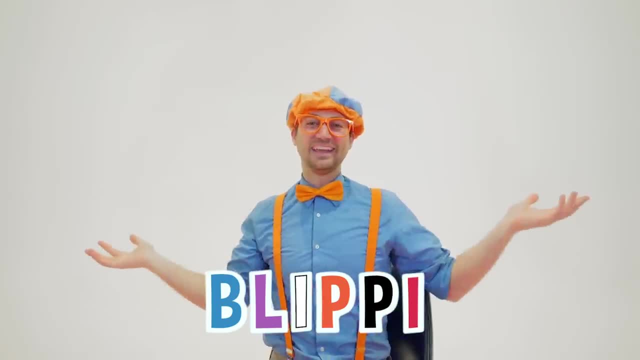 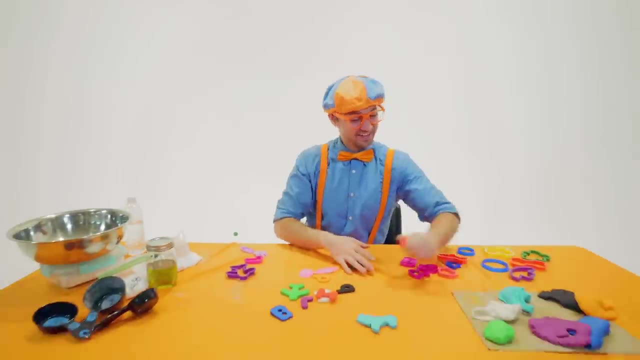 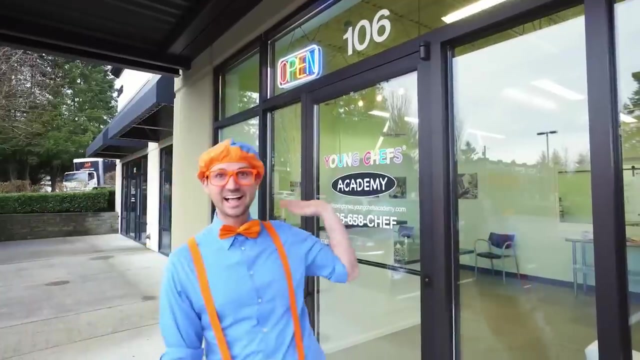 I Blippi. all right, thank you so much for being my friend. see you soon, bye, bye. So much to learn about. It'll make you want to shout Blippi's, Hello, Hey, It's me Blippi, And look at where I'm at. 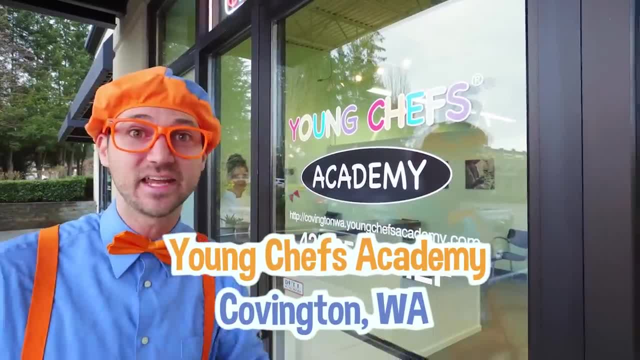 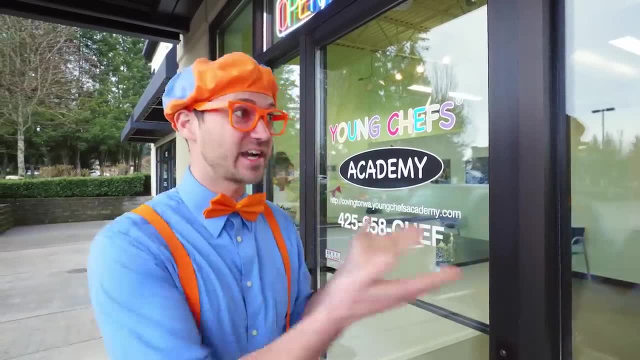 Well, today I'm at Young Chefs Academy in Covington, Washington. This place is so cool, Yeah, where. Well, today I'm at Young Chefs Academy in Covington, Washington. This place is so cool, Yeah, where young chefs- kids just like you- can come here and learn to cook some delicious. 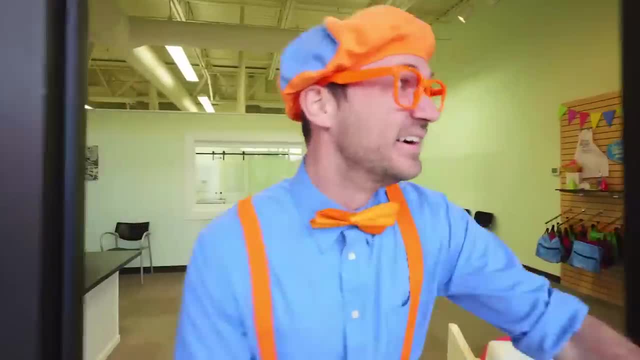 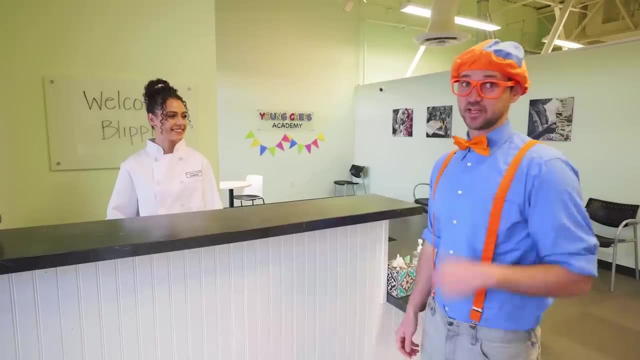 treats. Haha, Let's go. Hi Blippi. Hey, who are you? My name's Chef Riley. Oh nice to meet you, Chef Riley. Hey, do you mind if we go explore the kitchen? Go for it. I'll see you in a sec. 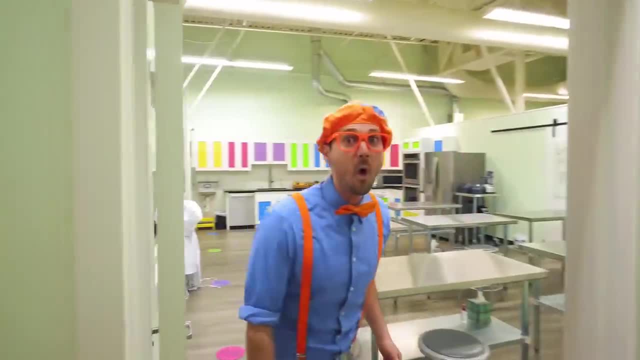 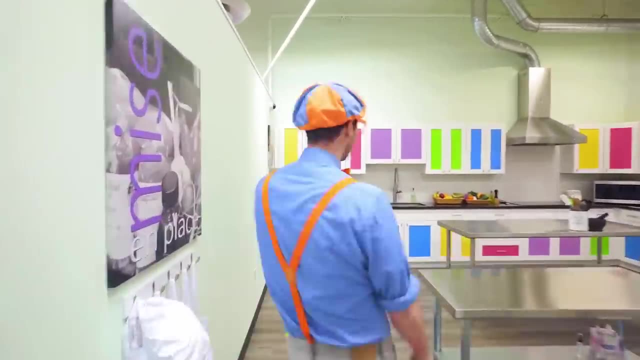 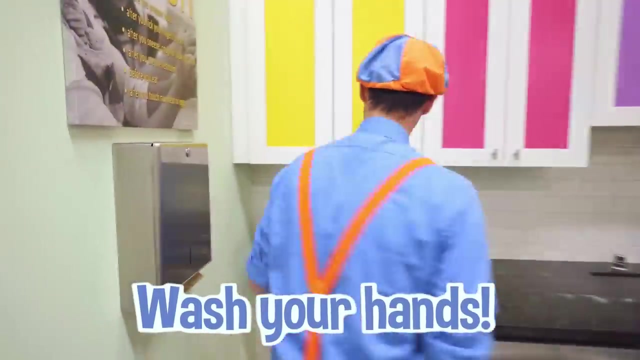 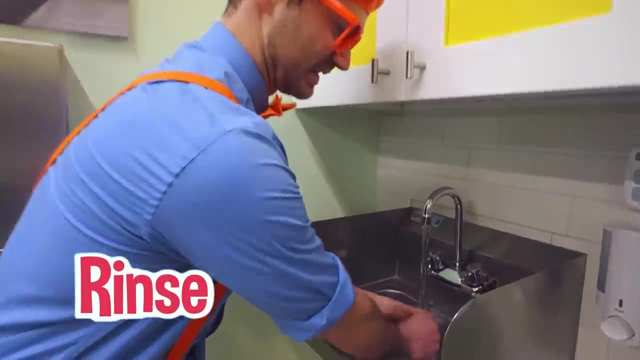 Okay, let's go. Wow, look at this kitchen. It is so bright and colorful. Whoa, come on. Okay, the very first thing that I need to do when we enter a kitchen is wash our hands. Okay, I'm going to turn on hot water and then I'm going to rinse them. Okay, get them. 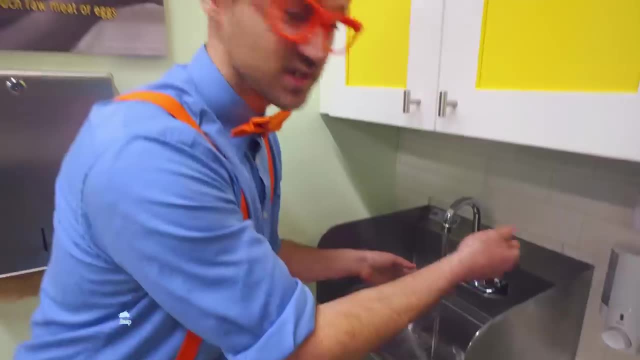 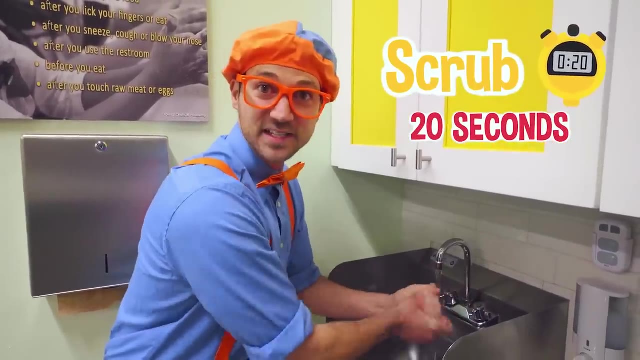 nice and moist, And then we need some soap, Okay, and we need to scrub for 20 seconds, And one way to do this is to sing the ABCs Ready: A, B, C, D, E, F, G. 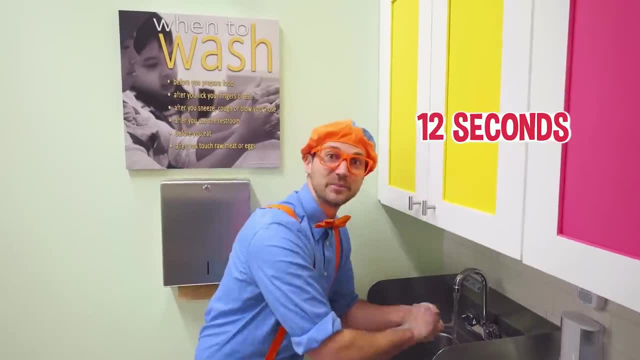 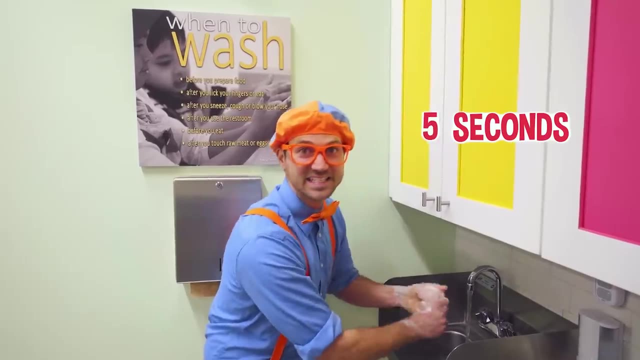 H, I, J, K, L, M, N, O, P, Q, R, S, T, U, V, W, X, Y and Z. Haha, Okay, now we can rinse off our hands. 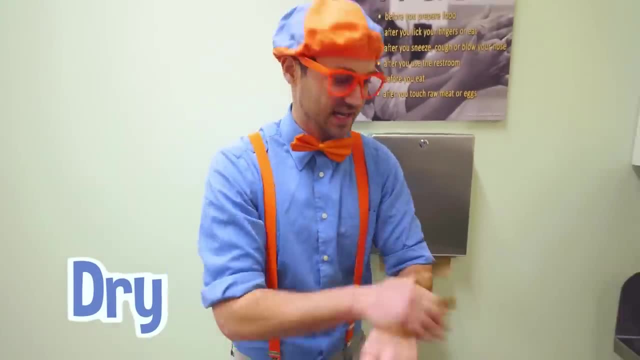 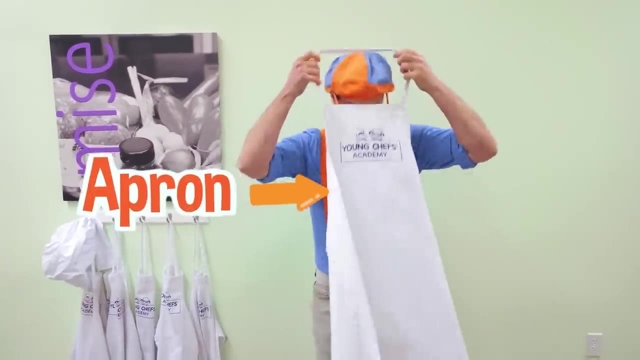 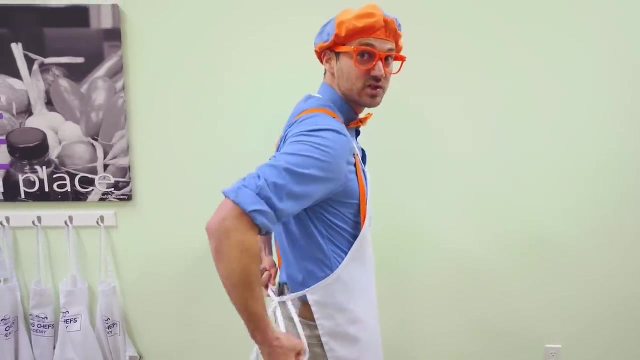 Let's get them nice and dry Now. once our hands are dry clean, Now we can put on our hands. We've got an apron- Yeah, an apron is used. so then clothes not get dirty when you're cooking with some food. 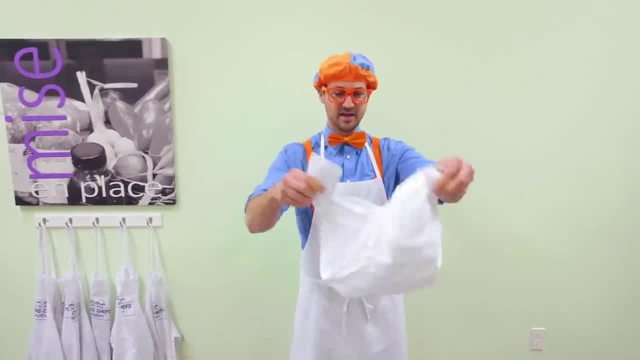 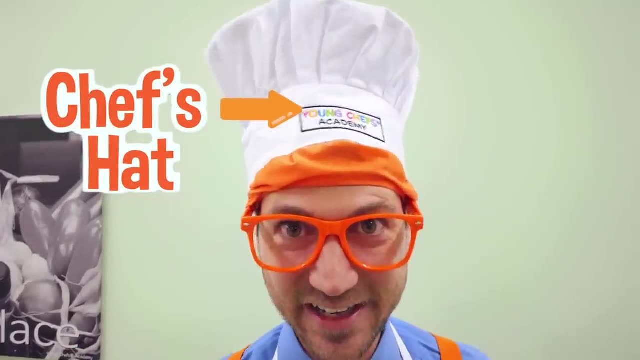 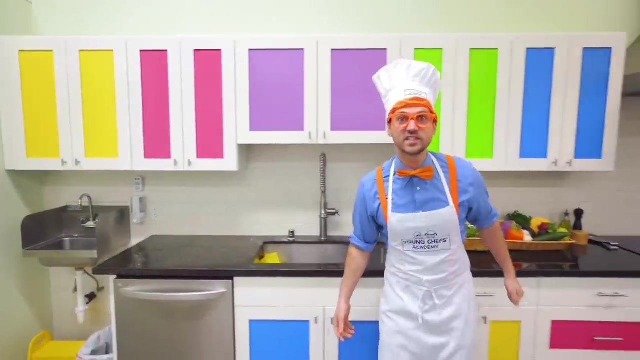 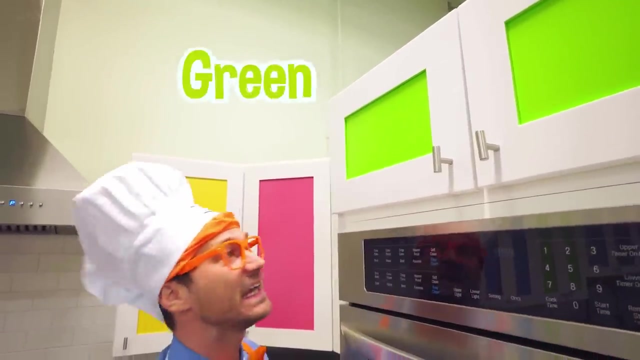 Alright, and can't forget my young chef's academy chef's hat. How do I look? Alright, check it out. This kitchen is so colorful. Do you see all these cabinets? Yeah, Whoa, These, yeah, are the color green. 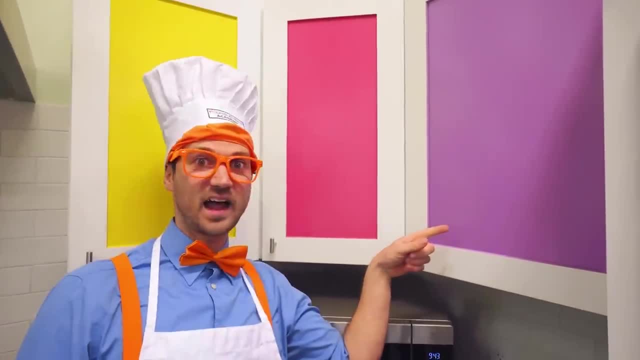 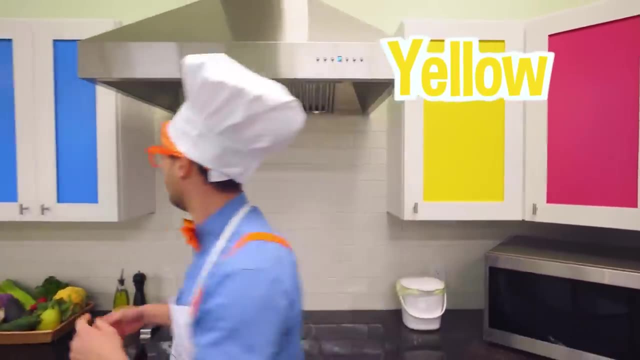 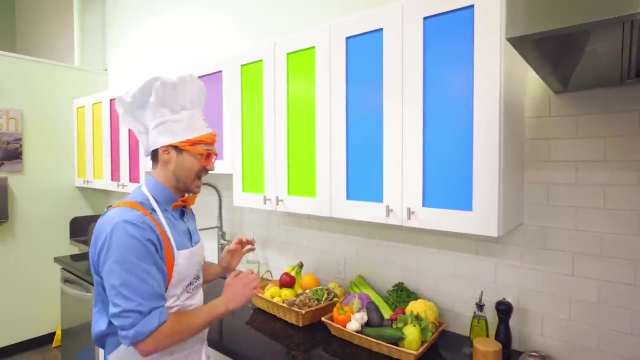 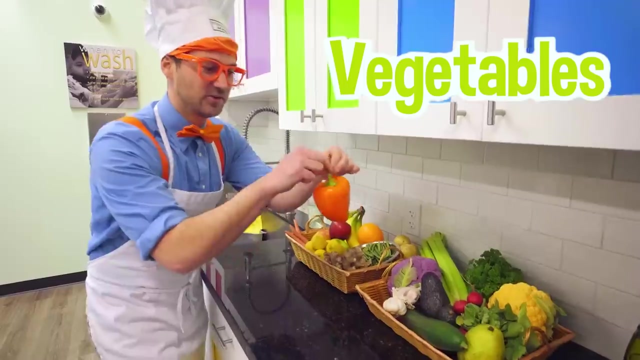 Ooh, this over here. yeah, that cabinet is purple, pink, yellow and blue. Whoa, I bet there's a lot of cool things in these cabinets. Whoa, Look at this, Some yummy vegetables. Hey, you know what kind of vegetable this is? 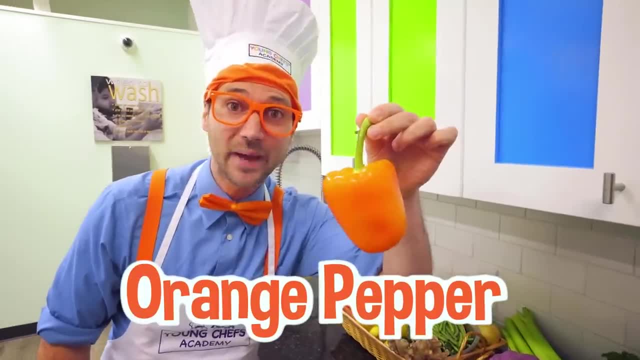 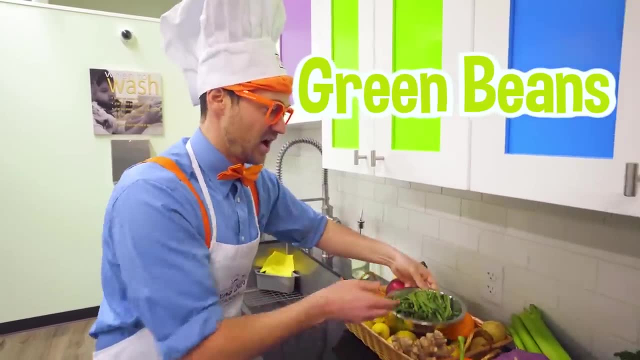 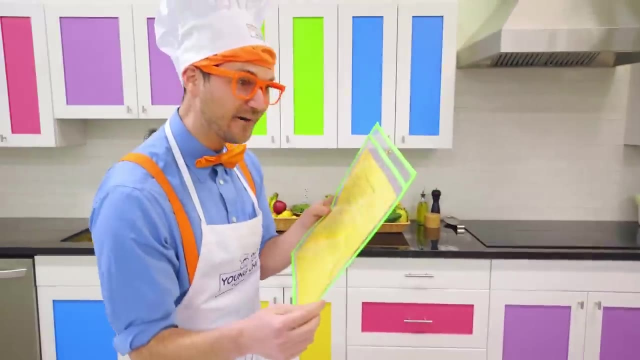 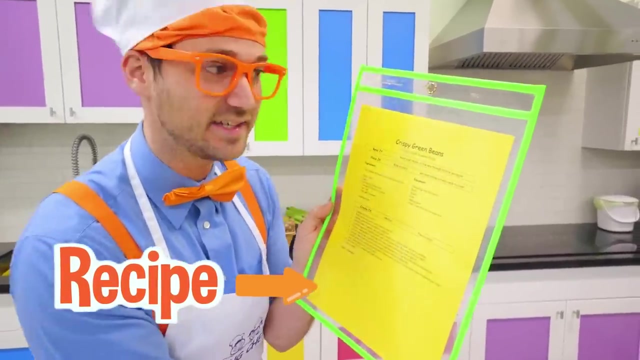 Yeah, this is an orange pepper. Haha, Look at these. Yeah, some green beans. I sure do love vegetables. Alright, I'm so excited. Whoa, I am so excited. This is gonna be tasty. I am looking at the recipe of what we're gonna be making today. 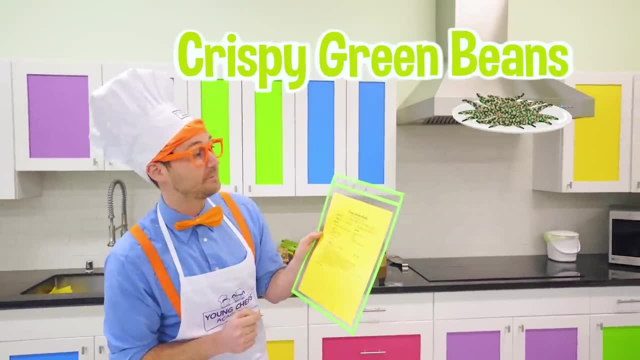 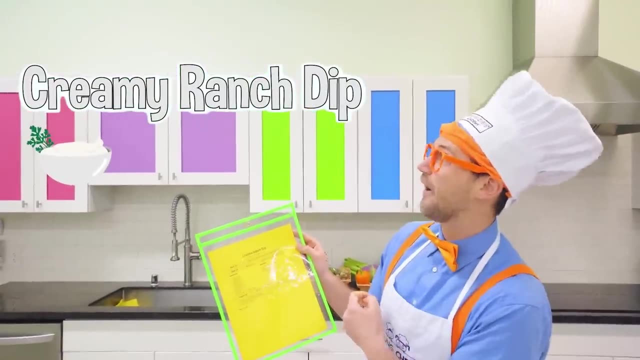 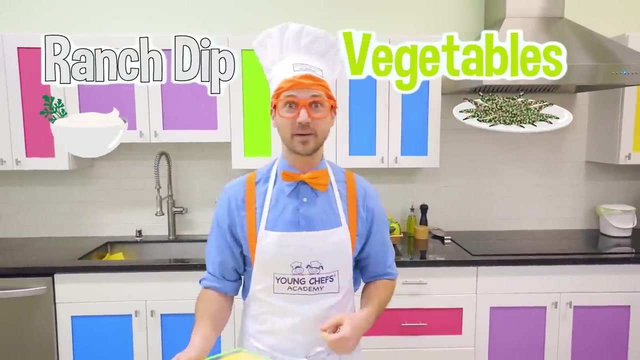 Looks like we're gonna be making crispy green beans- Whoa, Those look tasty- And creamy ranch dip- Oh, this is gonna be so yummy and healthy. I love vegetables and I love ranch dip. I wonder if we're gonna be able to dip the green beans into the ranch dip. 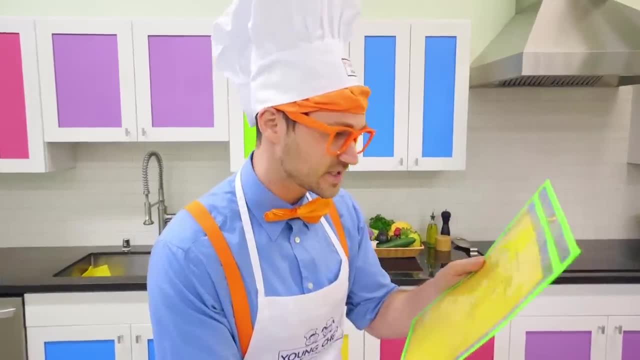 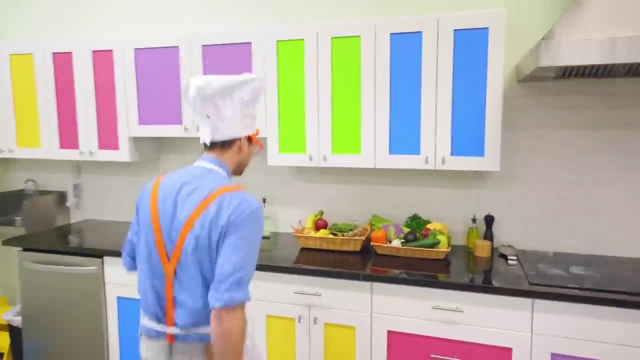 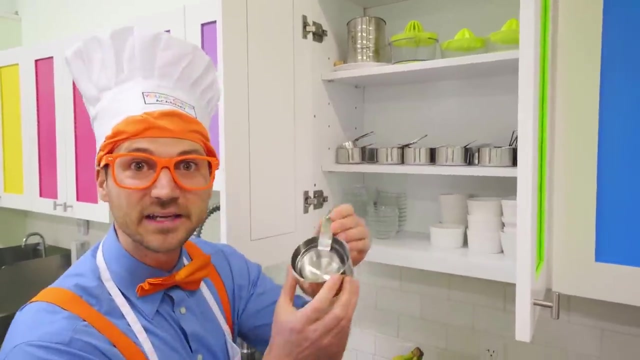 Yeah, Okay. so it seems like we need a lot of tools and a lot of ingredients. So, uh, let's get to it. Alright, let's see what's in here that we need. Okay, looks like we need some measuring cups. 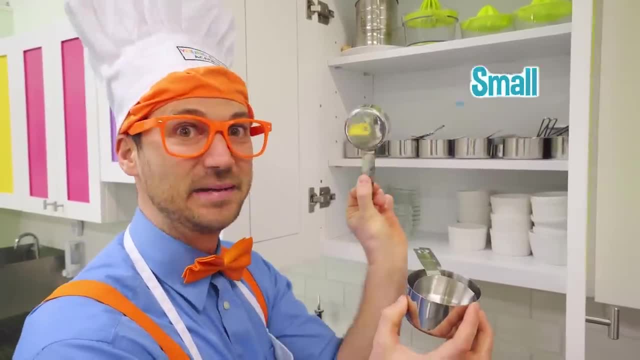 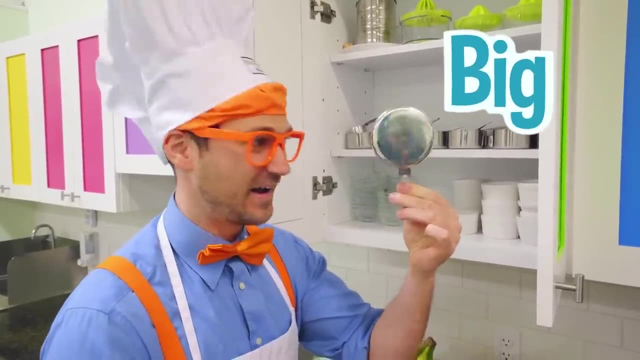 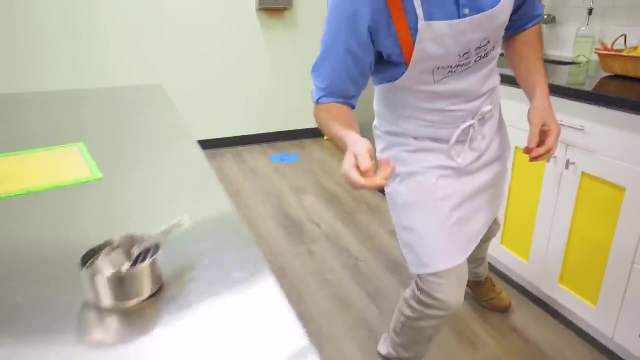 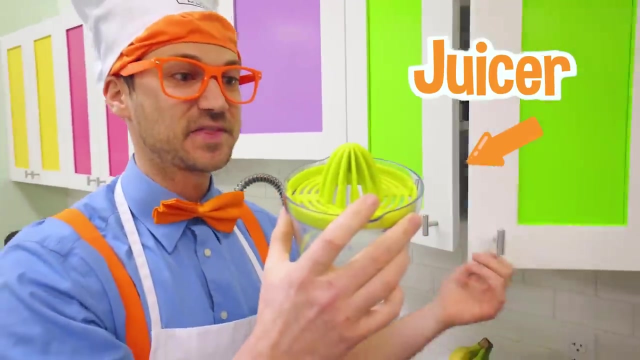 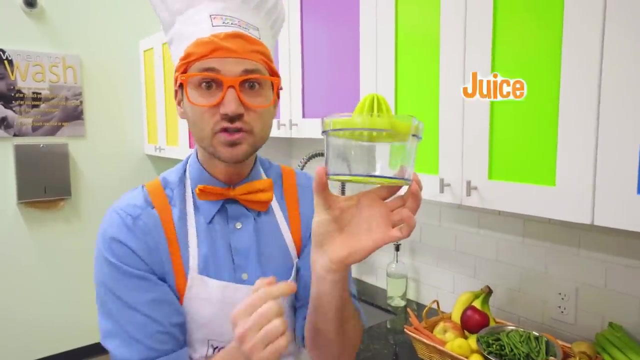 Ooh, a small one, A medium-sized one, Another medium-sized one And a big one. Okay, Put those right back here. Perfect. Then we need Whoa, A juicer. This is where you can put a lemon or an orange or a lime, squeeze it on top and then all the juice comes out the bottom. 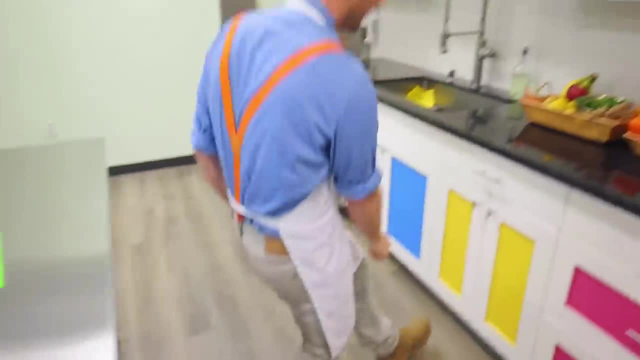 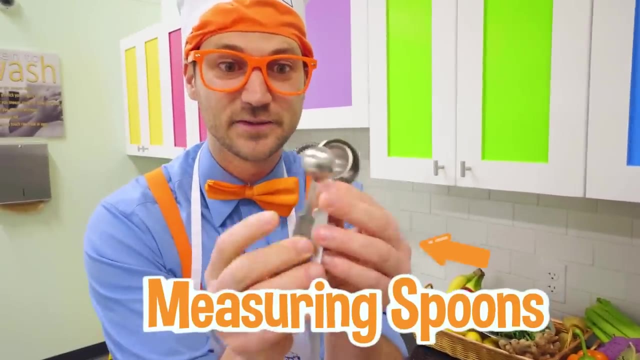 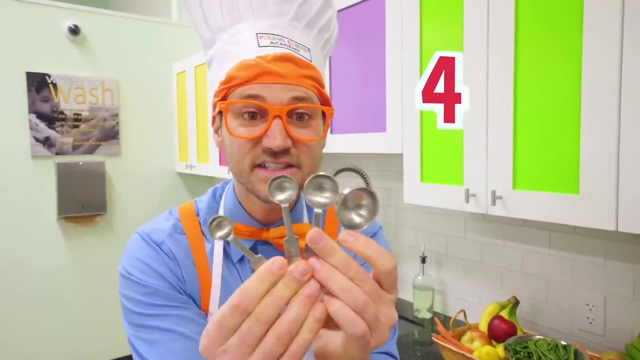 Okay, we'll set that down right there. Alrighty, let's see what's in here. Hmm, Oh, We definitely need some measuring spoons. Whoa, Yeah, same thing, just like the measuring cups: Measuring spoons of four different sizes. 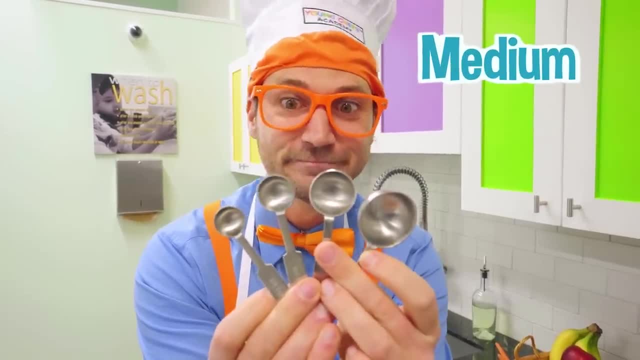 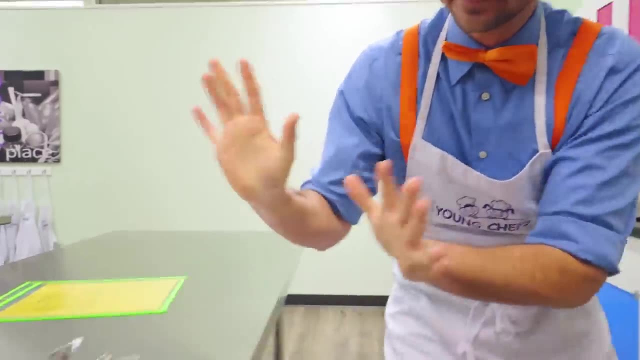 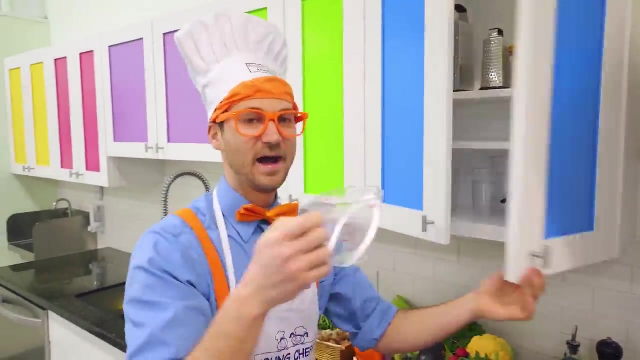 From small to medium to medium to large. Okay, Put them right About right in there. Perfect, Okay, uh, let's see How about. Uh, Oh, Wow, A measuring cup. This is what you put: liquids and. 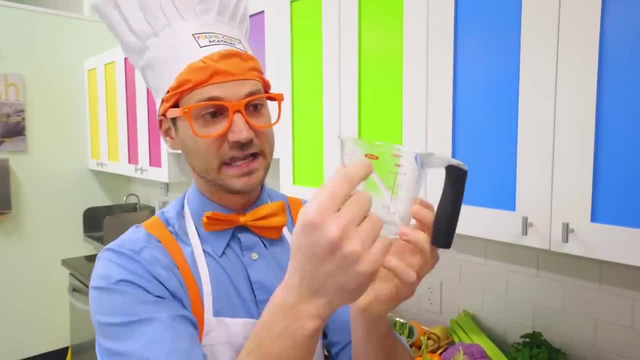 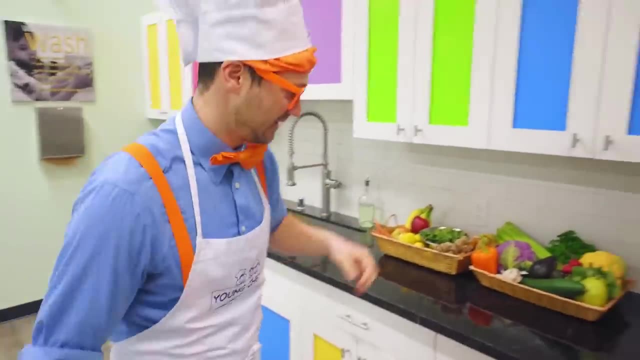 You could do solids, but this is primarily for liquids, And this is what you measure: to see how much you have. Okay, Put that down right there. Oh, let's see. Is there anything in here? Hmm, There's a lot of cool things in here. 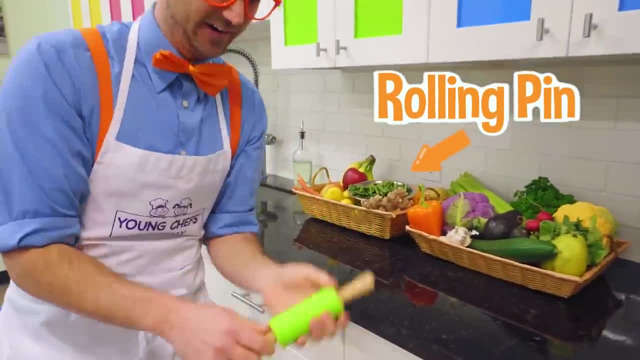 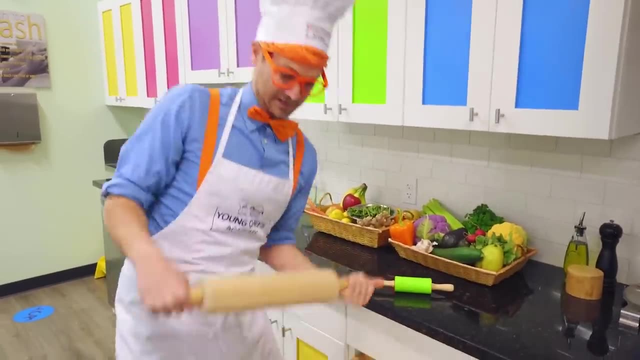 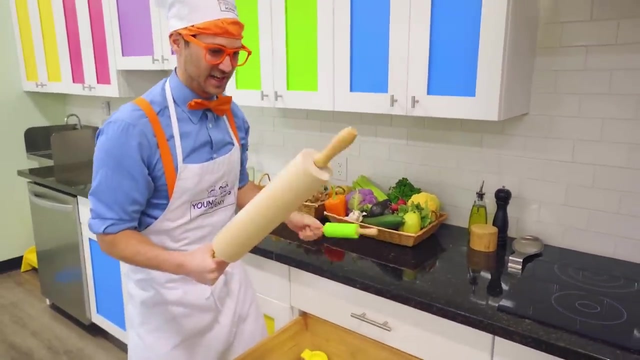 Whoa. Look at this, It's a rolling pin. Oh So cute. This is a small rolling pin Whoa. And this is a big rolling pin Whoa. They're used to flatten things out. I don't think we need those today. 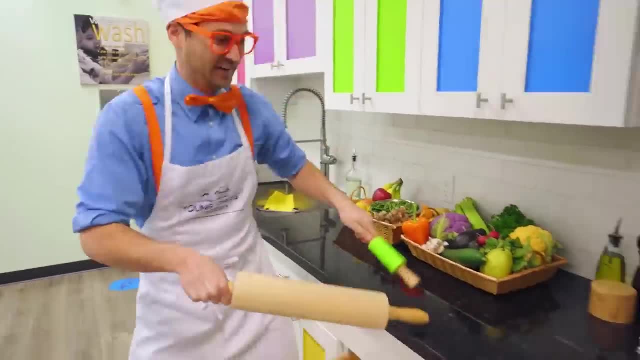 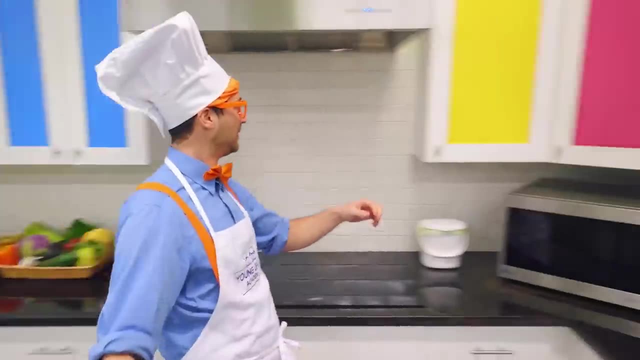 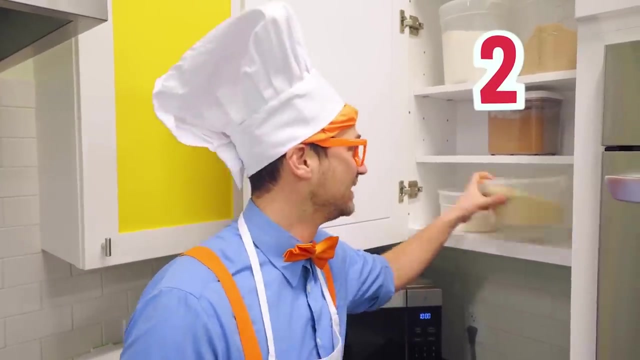 But they're pretty cool because we can use them for drums. Okay, Enough playing, Let's get to cooking. All right, Let's see, Um, probably right in here. Oh yeah, Two ingredients that we need: Breadcrumbs. 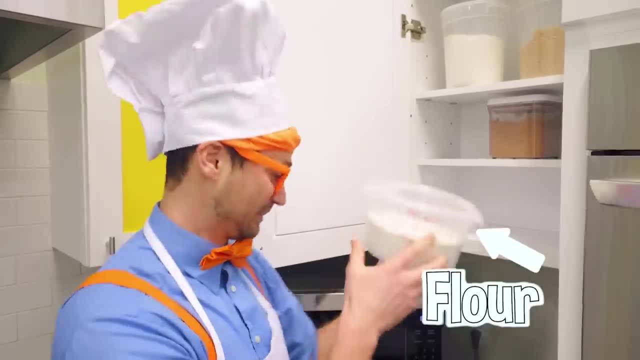 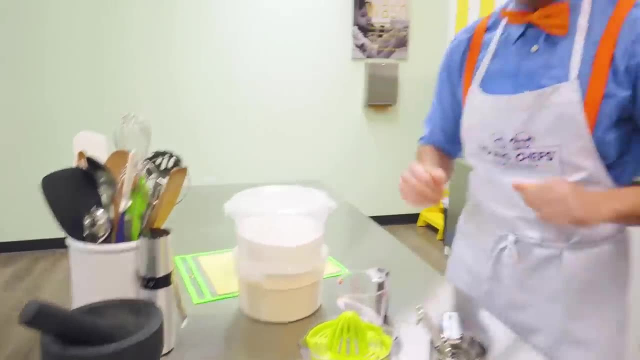 And flour, Perfect, Okay, We'll shut this. All right, There we go, And uh, let's see How about some cold ingredients? Wow, Look at this fridge, It's so organized. Huh, Okay, Looks like we have some cream. 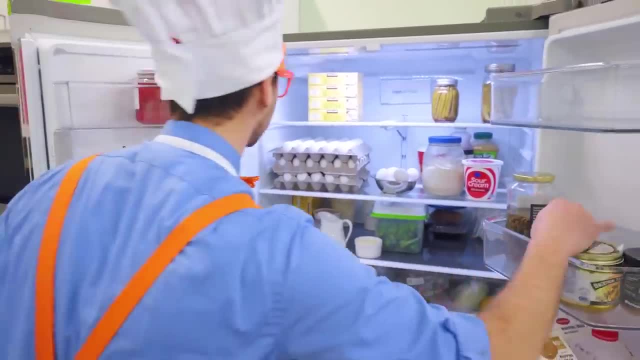 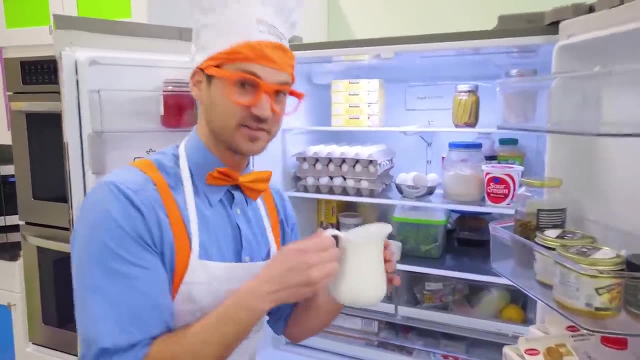 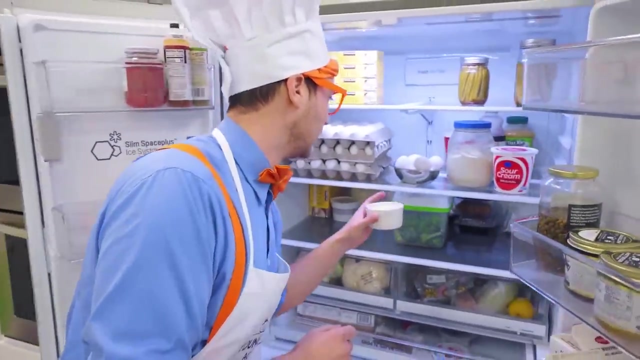 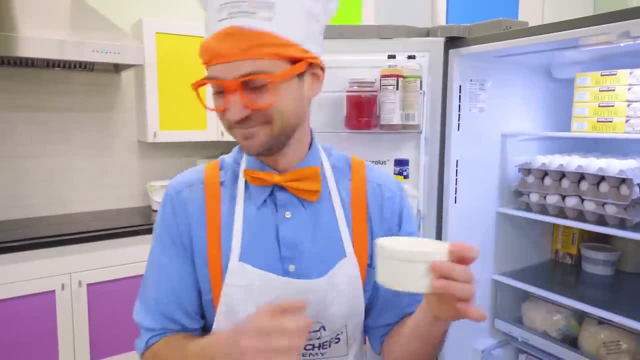 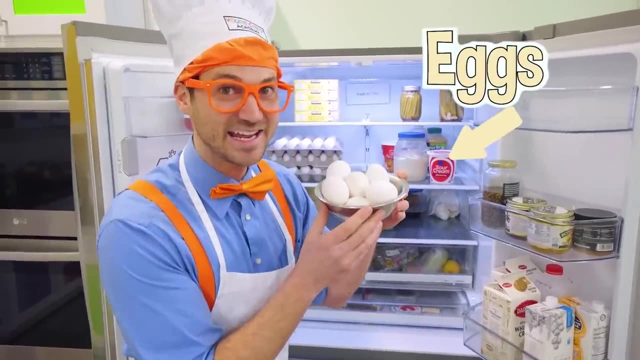 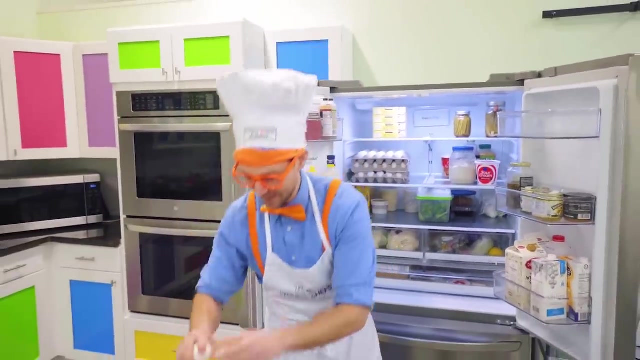 Parmesan cheese. Ha ha, Ha, ha. Okay, I'm going to put that down right there. And then we have some eggs. Yeah, Check this out. Whoa, Whoa. Okay, We'll put those down right there for later. 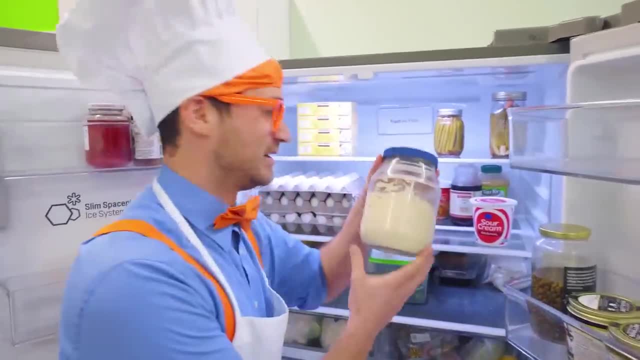 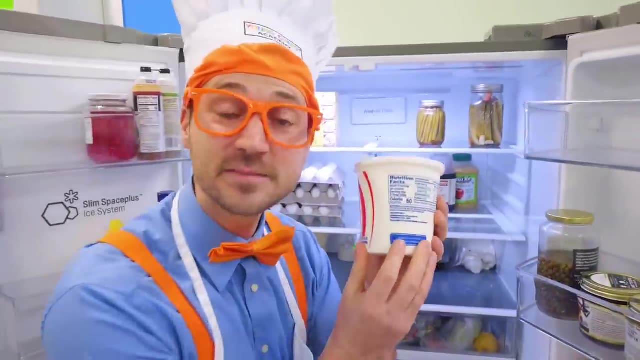 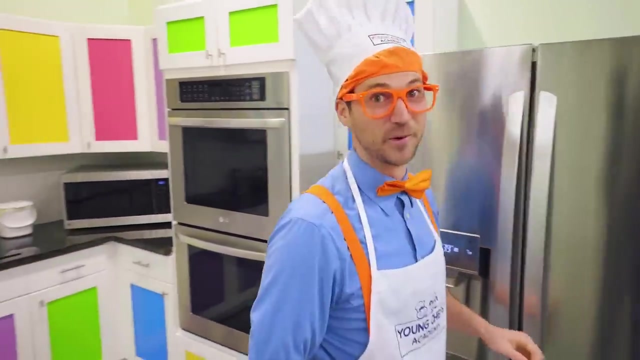 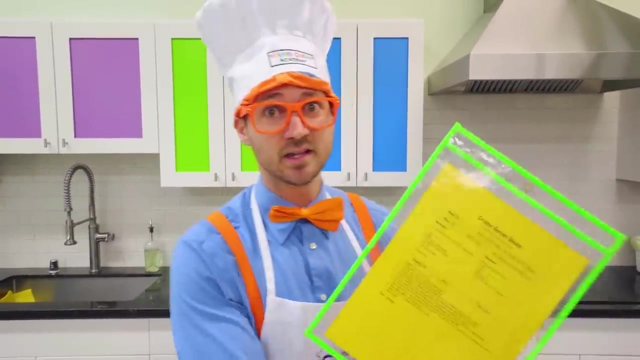 Probably shouldn't do that at home. and then we have some mayonnaise- put that down right here- and some sour cream- okay, put that down. and now I think we're ready. looks like we have most of the ingredients and tools, but this looks really hard. oh no, if only I had some. 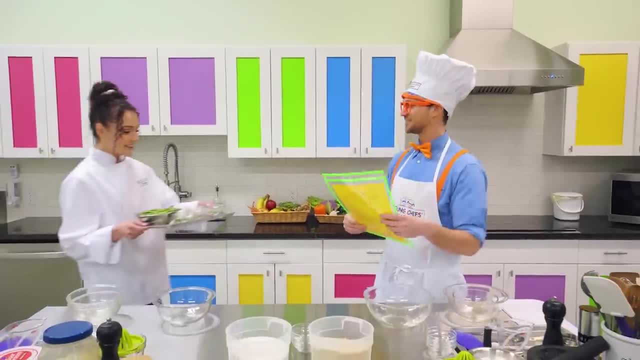 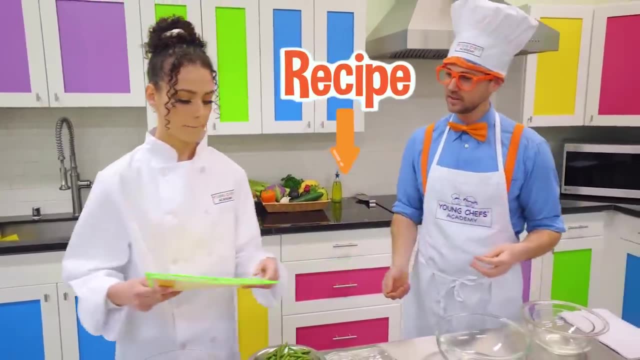 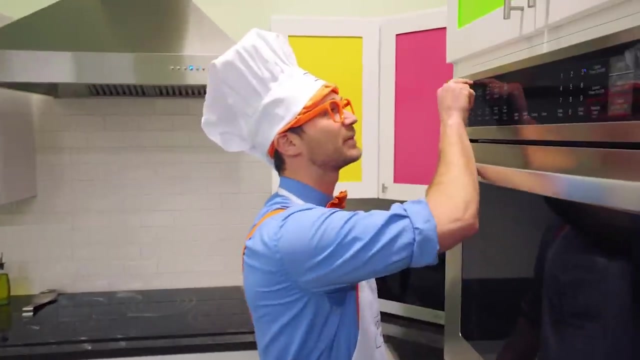 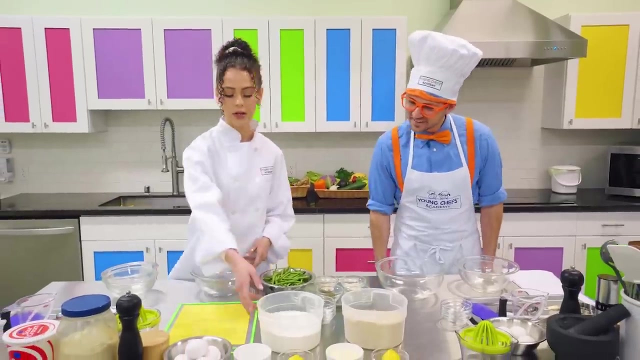 help. Oh, perfect, okay. well, here's the recipe. what do we do first? first, we're gonna want to preheat the oven to 425. okay, I know how to do that. ok, preheat the oven to 425, perfect, thank you right. first, we're gonna want to do a. 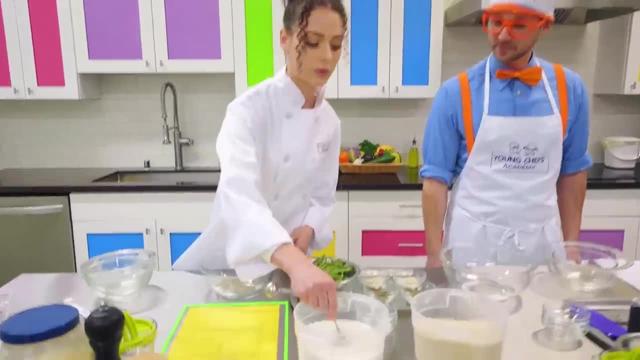 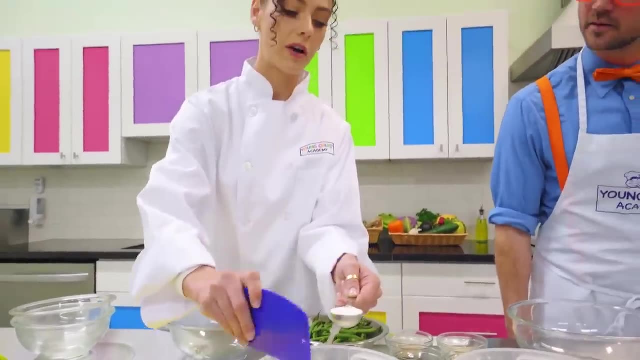 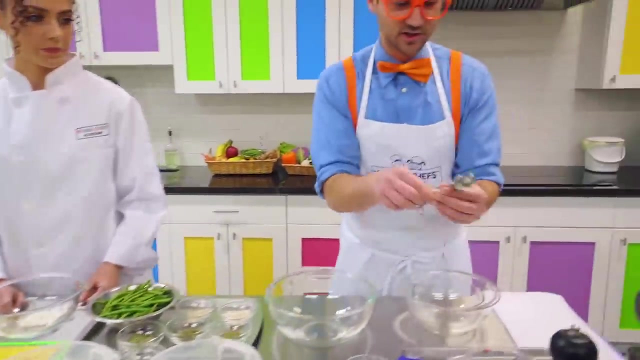 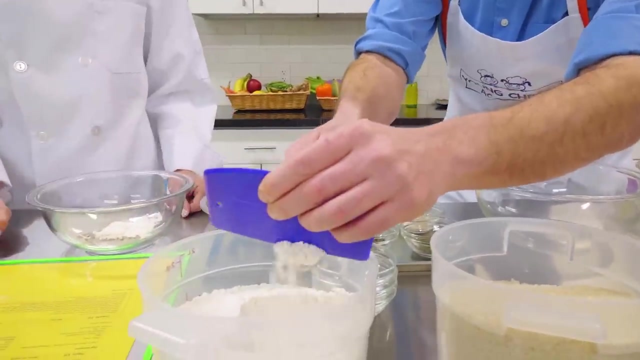 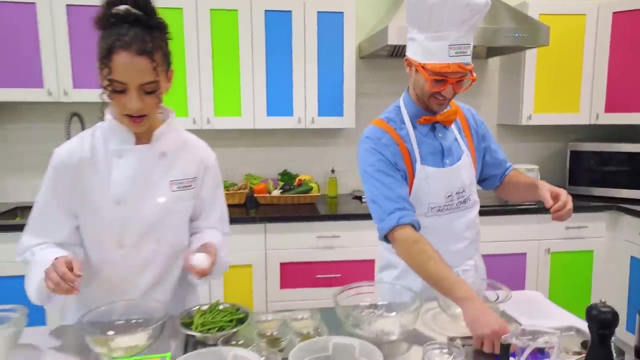 tablespoon of flour into our bowl. okay, want to make sure that we get a true tablespoon, because that is not accurate, so we want to scrape off the extra flour. okay, okay, can you do that? sure, okay, looks like we need some flour. let's do a little scoop and there we go and perfect, great job, looky, all right. next we're gonna want: 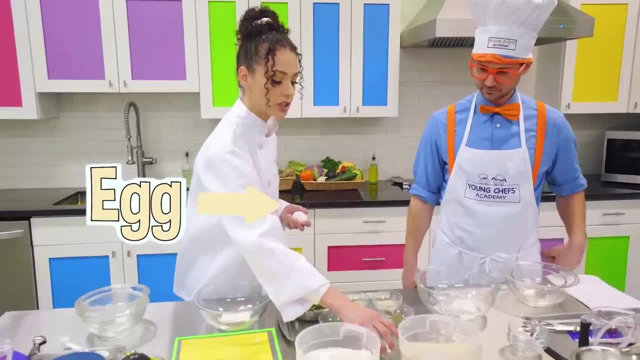 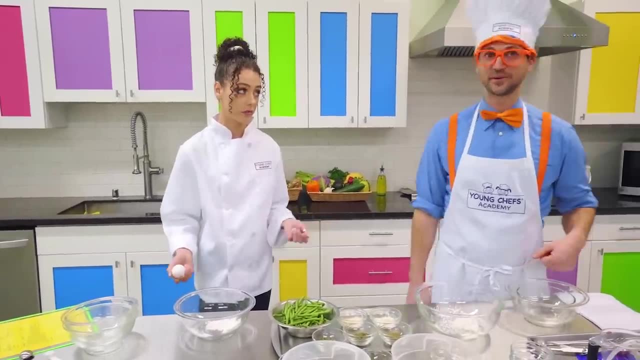 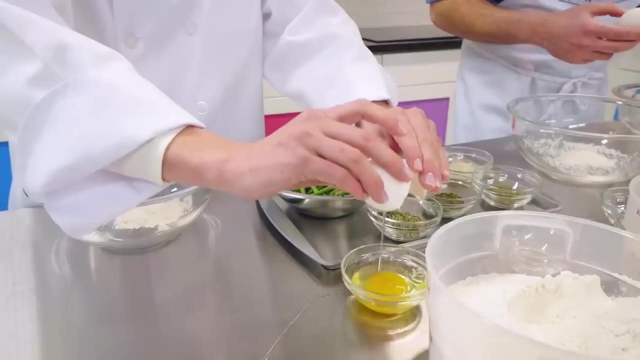 to crack an egg. okay, see, so at young chefs academy we crack an egg using the table, not the edge of the counter, so that it doesn't get all over the floor in the mix. okay, you want to crack hard and use your thumbs to break open the egg, just like that. perfect, you'll want to. 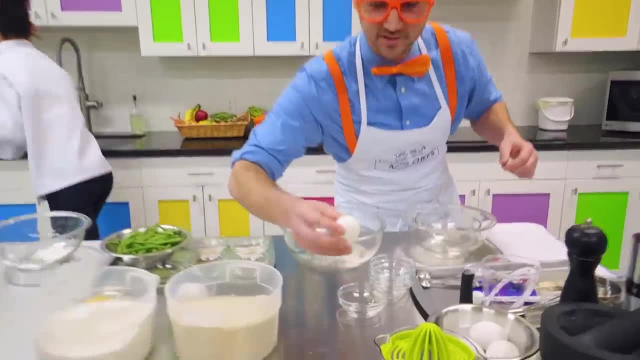 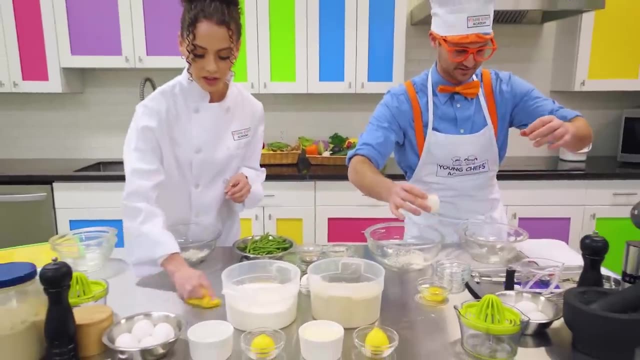 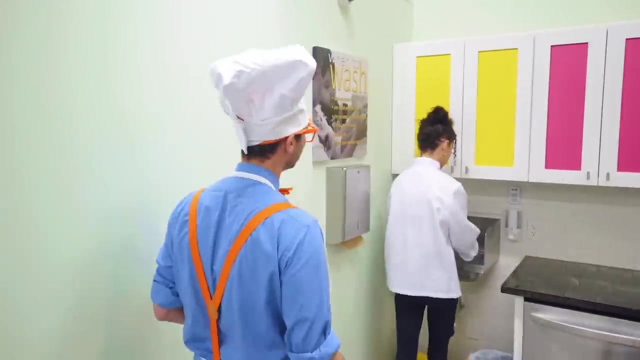 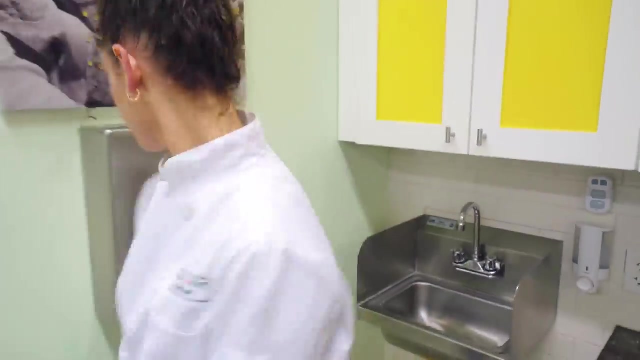 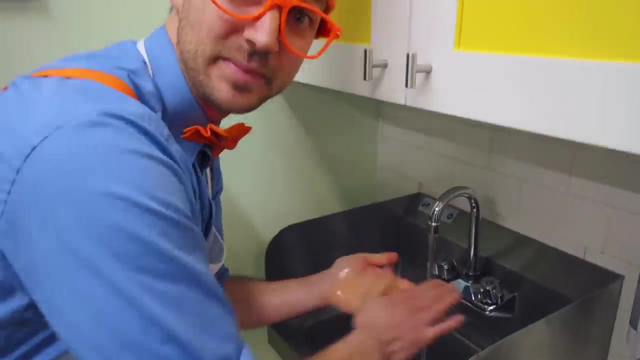 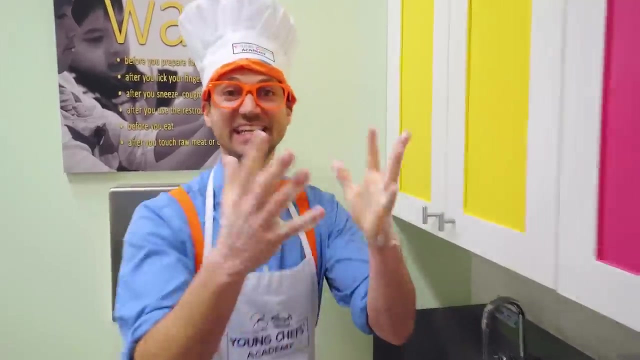 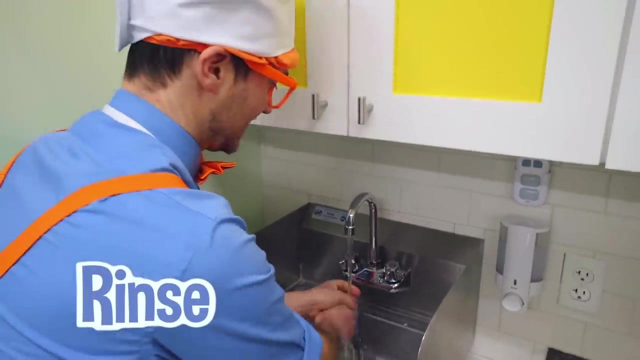 put the shell in a separate bowl. okay, here we go, let's use the table. there we go. great job, thank you. we're going to want to wash our hands because we touched a raw egg, all right. all right, there we go, let's rinse them off. it's really important to rinse off your hands and 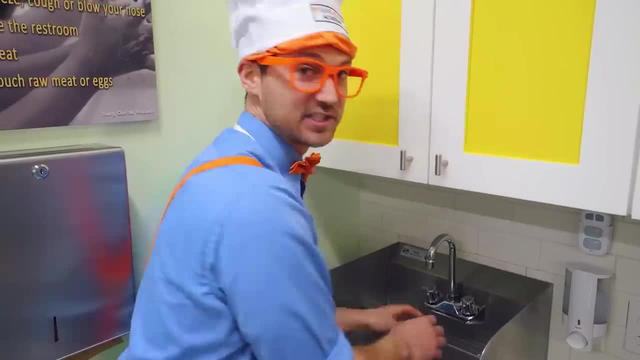 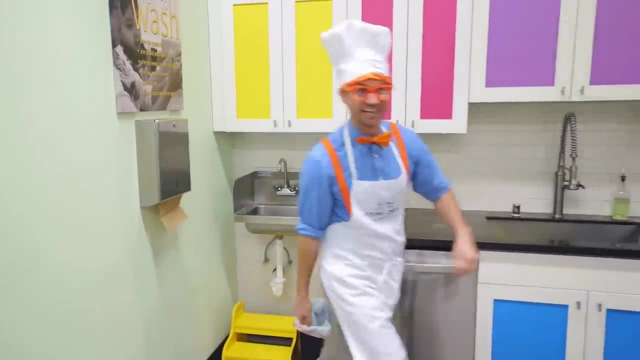 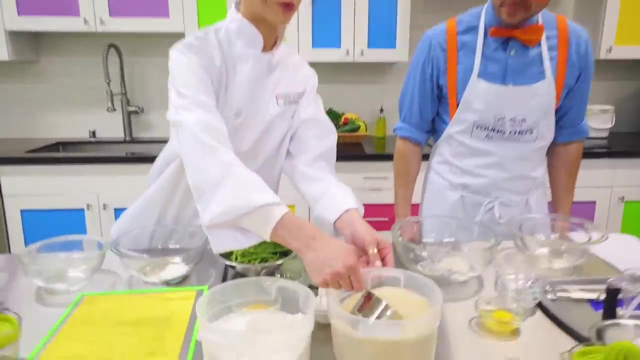 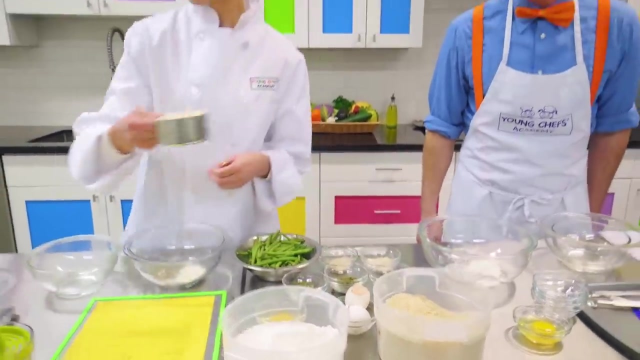 wash them completely after touching raw eggs or meat or anything like that. now we're ready. okay, all right. next we're going to want to do a cup of panko. okay, use our. wow, so this looks about right. yeah, it's just panko, just like bread crumbs. it is dried bread from. okay, all right. 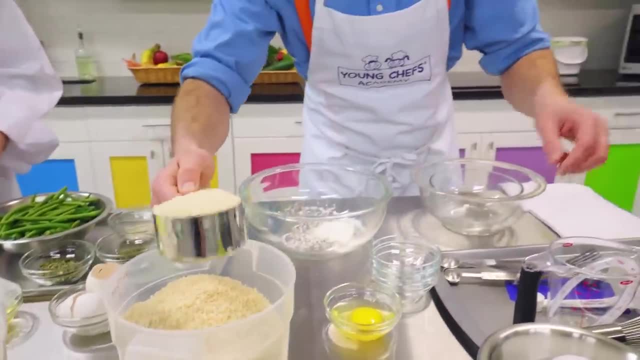 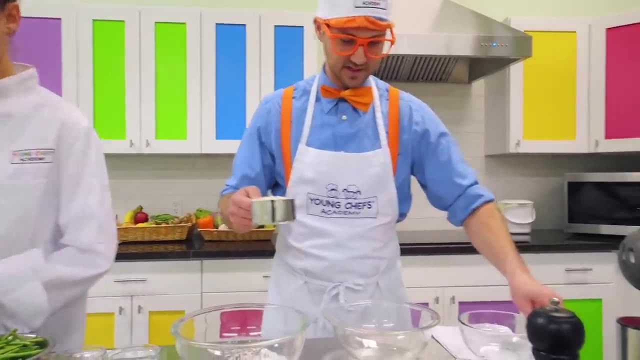 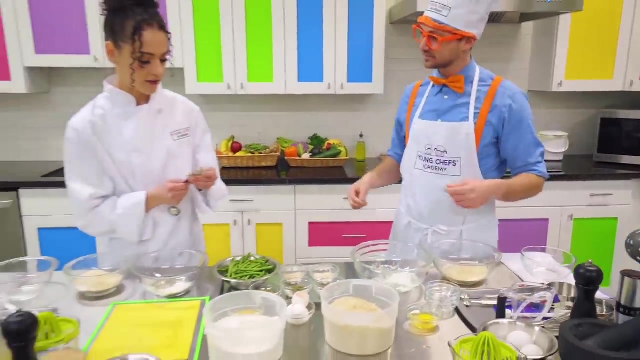 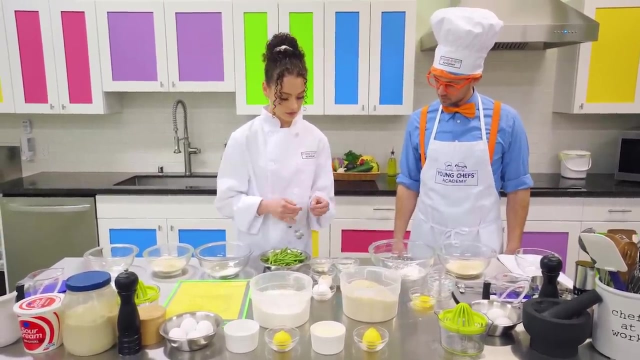 let's use that. okay, one big scoop, all right, in the same bowl. yeah, oh, so sorry, in a different bowl. okay, oh, thank you. okay, here we go, perfect, all right. next, we're going to want to add the rest of our spices, which is garlic sauce and salt. okay, so we're going to want to use a tea, a fourth of a teaspoon of garlic salt, in our panko. 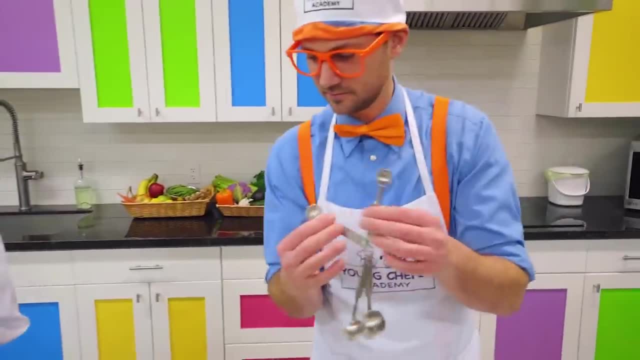 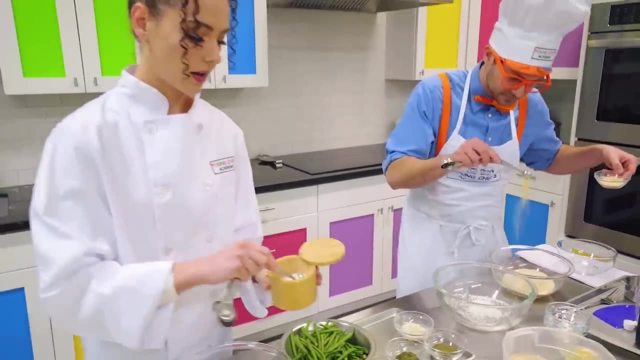 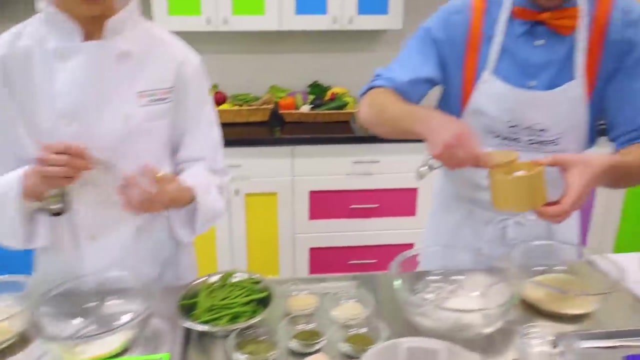 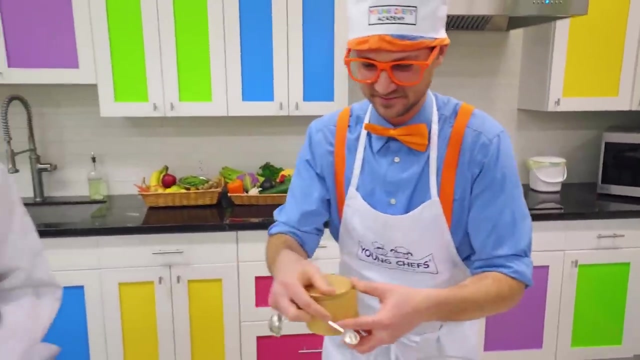 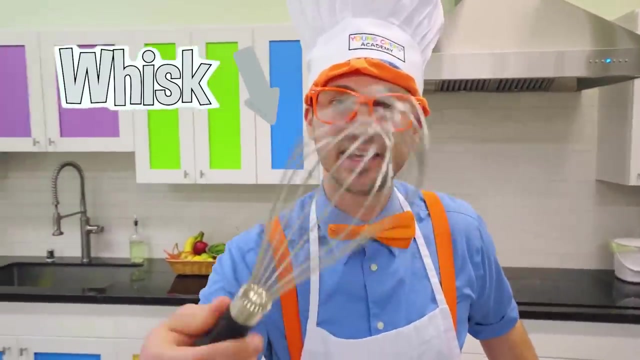 okay, here we go. this one, okay, and then put it in the panko. perfect, and then half of a teaspoon of salt. thank you, wow, salt is so yummy. here we go. can you use your whisk and whisk that up? yeah, check it out, this is a whisk. yeah, how do you do it? whisk with your wrist, okay. 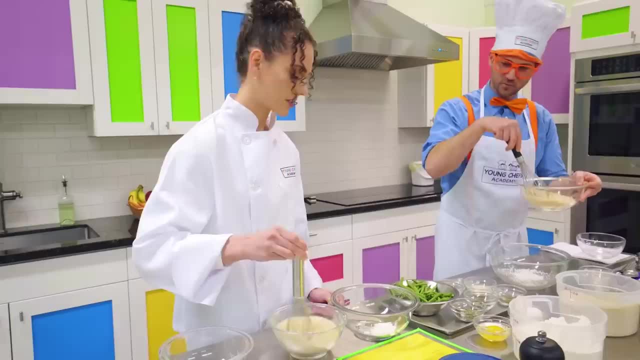 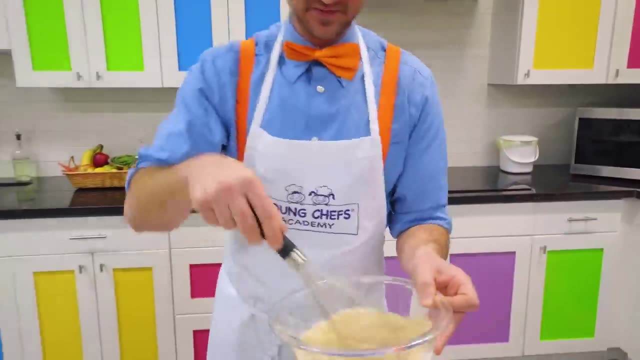 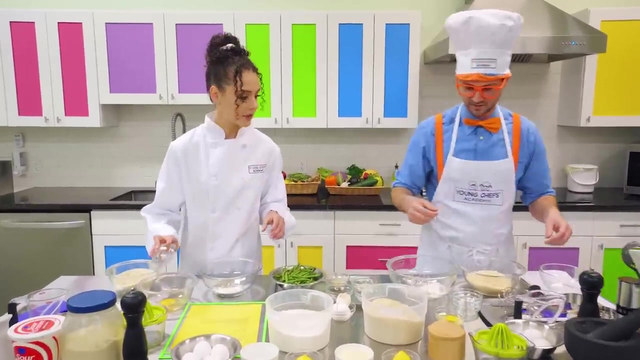 oh, this is a really good way to mix it all up. yeah, you want to use it like that, all right. next, we're going to want to put our egg into this mixing bowl, the clean mixing bowl that we have. okay, here we go, put the egg in this bowl. 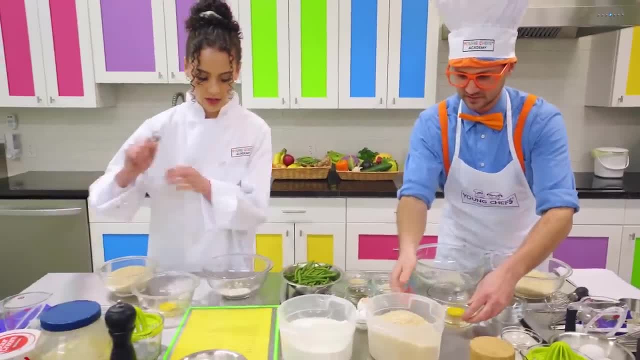 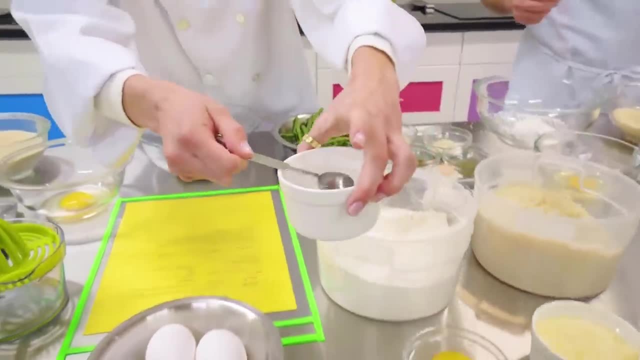 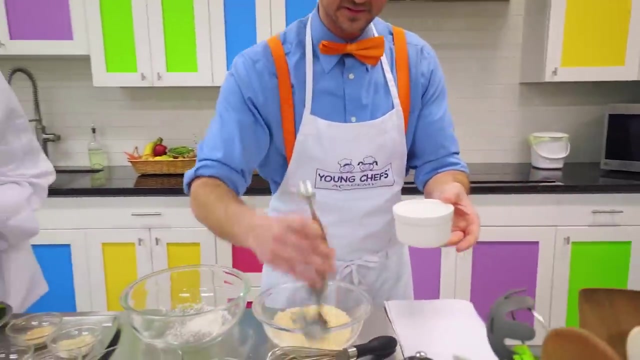 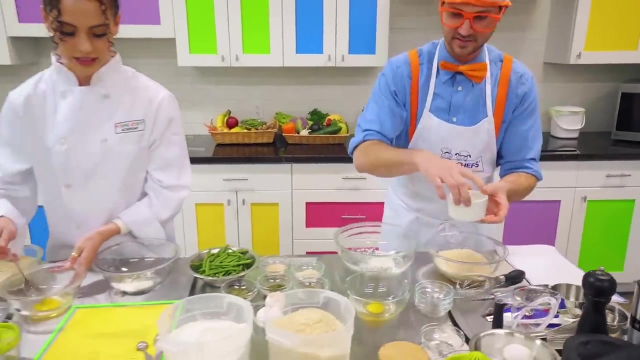 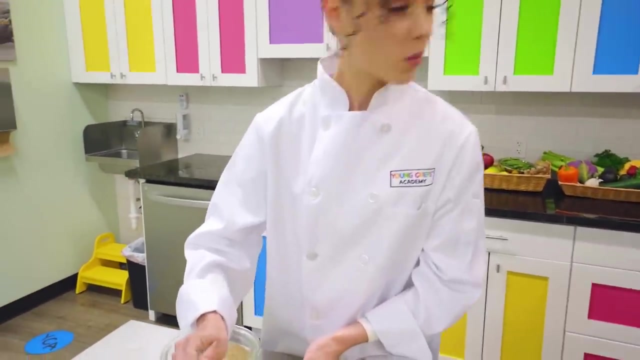 all right, and we're going to want to use a little bit of water, some water like this and with the egg. perfect, thank you. all right, put some water in with the egg. perfect, can you whisk that egg up with the fork? for me, with the fork, forks are easier to whisk eggs than a whisk is. oh, so you want to whisk it? 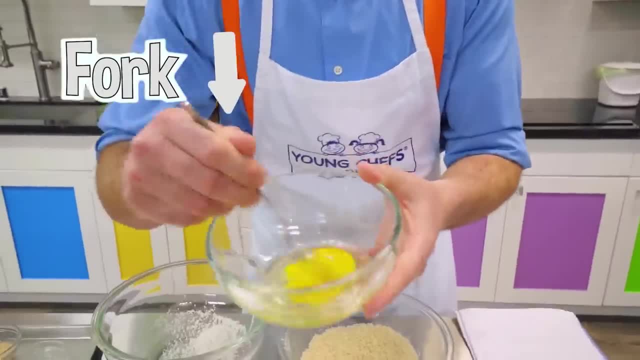 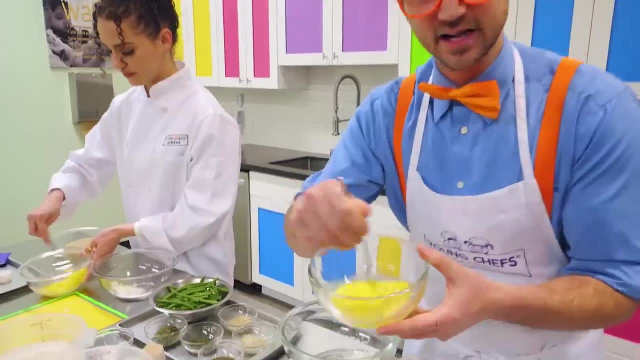 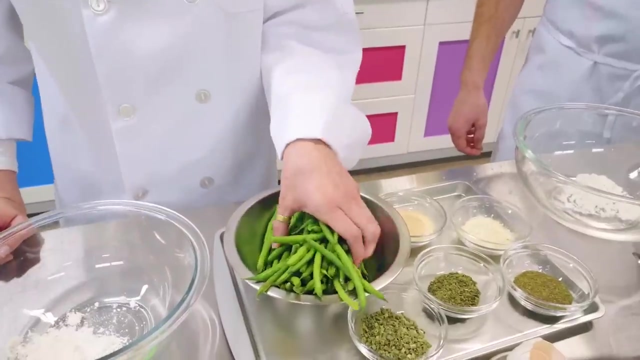 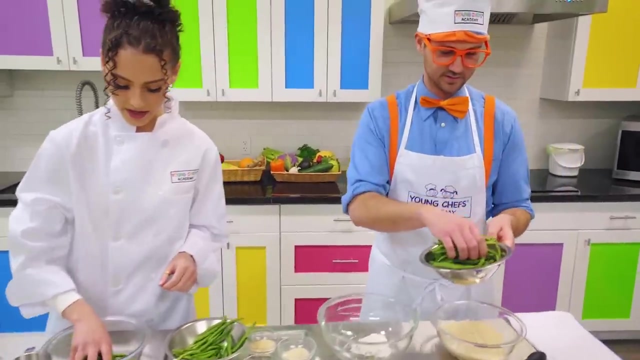 okay. so let's take the fork and let's whisk the egg. whoa, did you see that yolk broke up, and now it's all mixed up- perfect. we're gonna grab a couple handfuls of green beans right in here- all right, perfect- and toss it in our flour- all right, make sure you get them all nice. 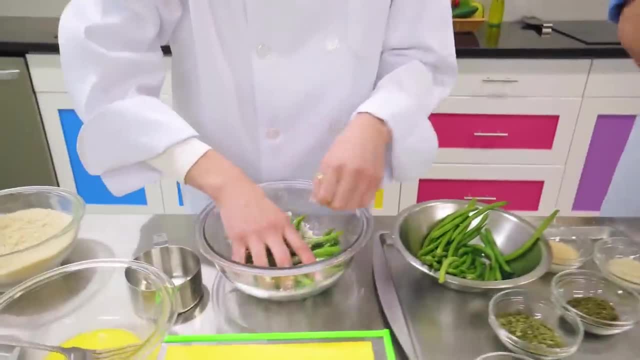 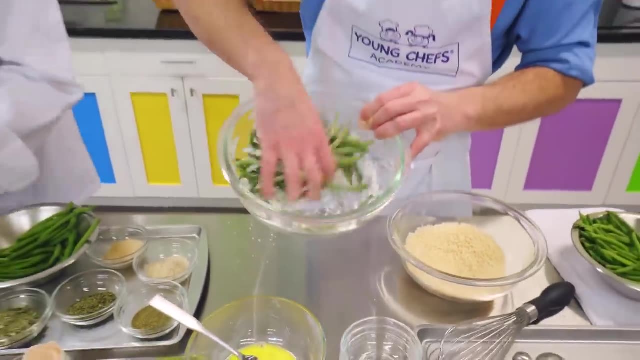 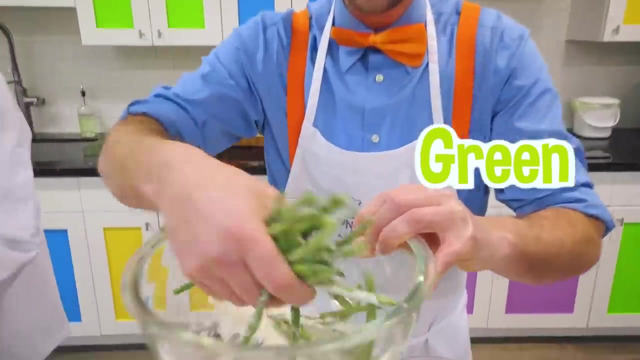 and mixed up and coated in flour. okay, toss it. okay, all right, all right, all right. Wow, This is gonna help the egg stick to the green bean. Okay, interesting. Look, they used to be green, but now they're green and white. 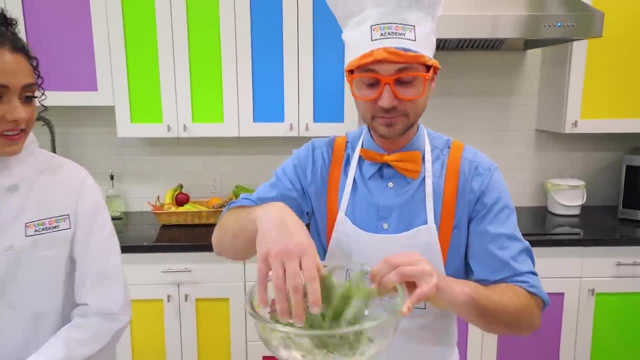 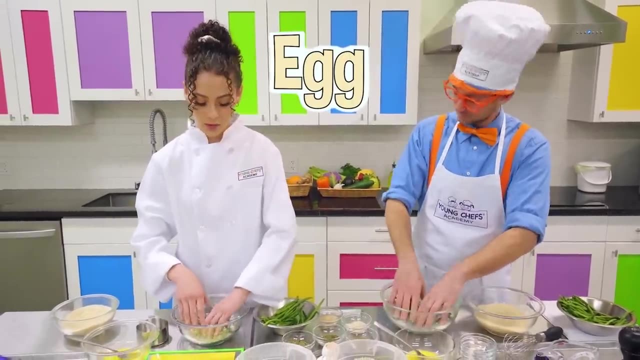 Hey, remember how we washed our hands? Yeah, good thing we did, because I'm touching food with my hands. You don't wanna touch anything after you touch egg or raw meat. You wanna make sure you wash your hands. Okay, All right, now we are gonna touch the egg. 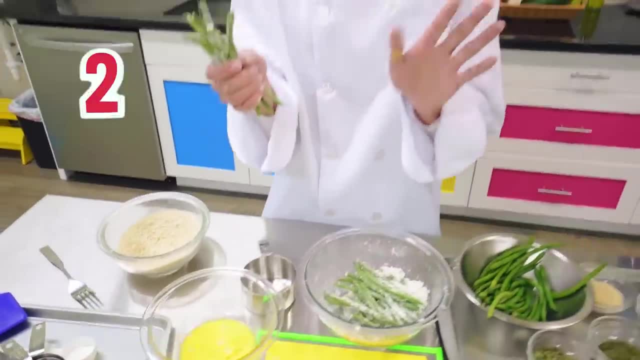 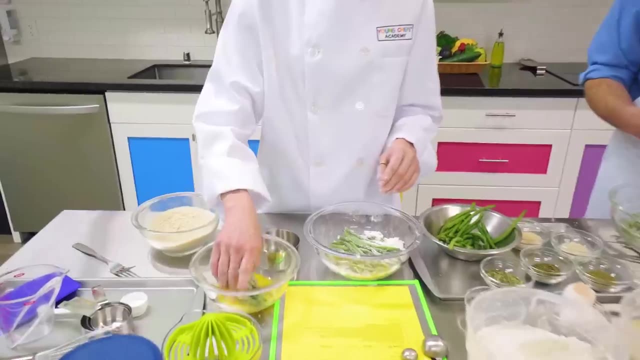 We're gonna put the green beans. We're gonna use two different hands. We're gonna have our dry hand and our wet hand, So we're not gonna touch the egg with this hand. We're gonna put our green beans in here and toss it around. 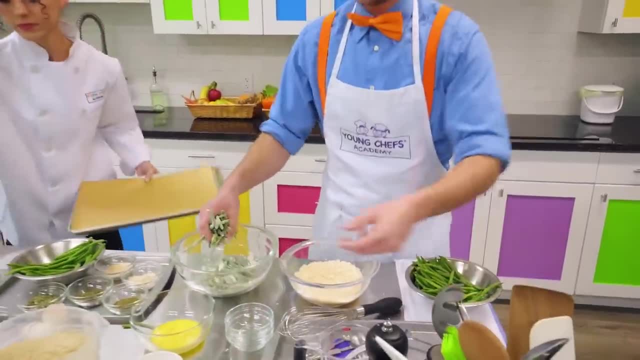 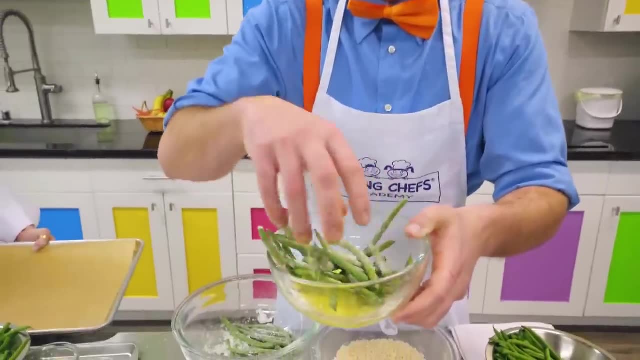 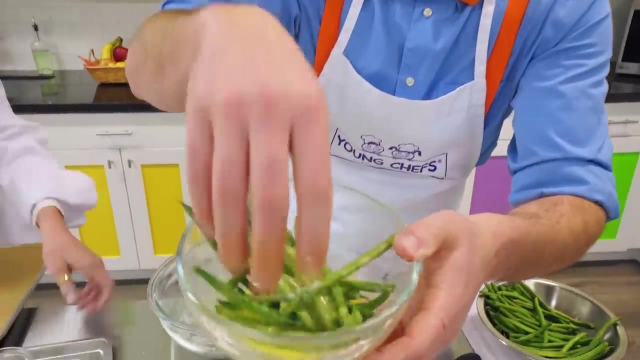 Okay, Take the fork out Now, let's do a little tossing. There we go. Whoa, I'm spilling, That's okay. Okay, Wow, Look at it, There's so much egg on these green beans, Okay. 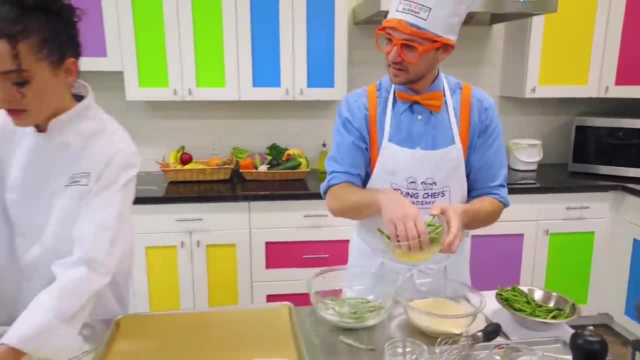 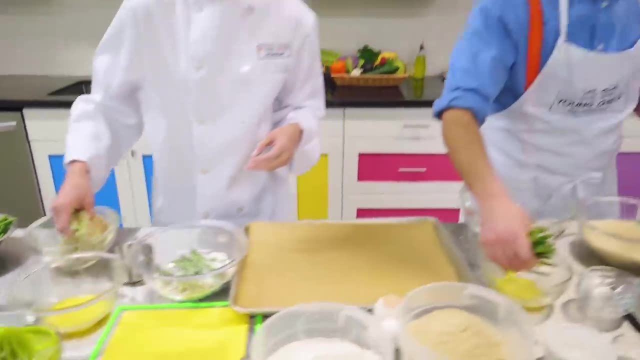 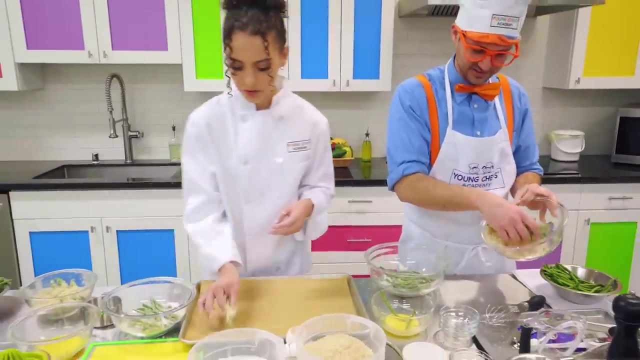 All right, great. Now you're gonna wanna put the green beans into the Panko, Toss them around real quick. Okay, Wow, Good job. That looks fun, And once they're nice and evenly coated in Panko, you wanna put them onto the tray. 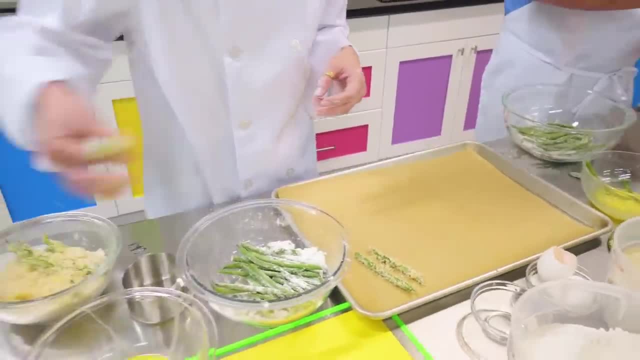 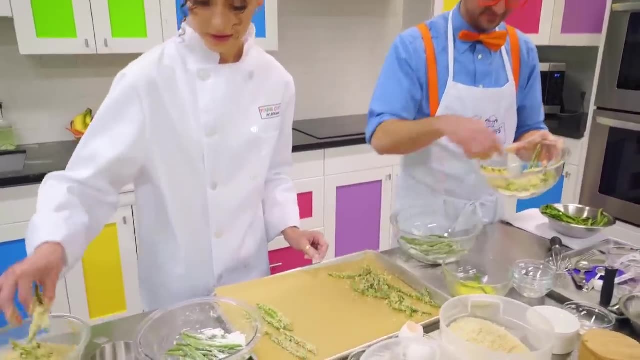 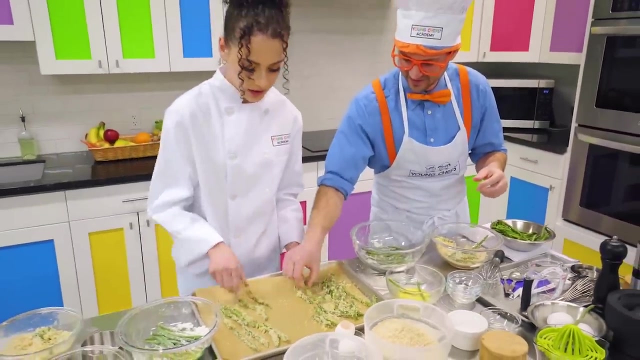 Okay, Whoa, These are gonna be so yummy. I know I'm excited. Let's put them a little bit nicer so that they're not so messy. Okay, That way they'll cook really evenly when they're spread out on the tray. 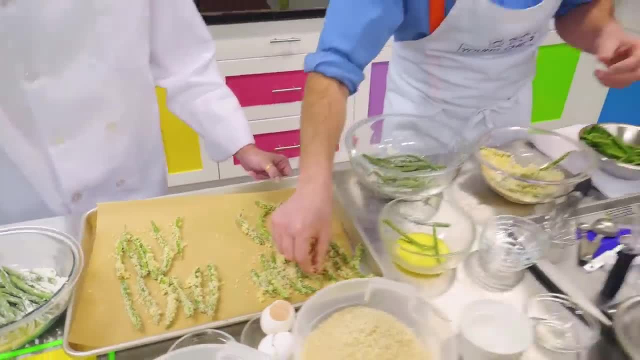 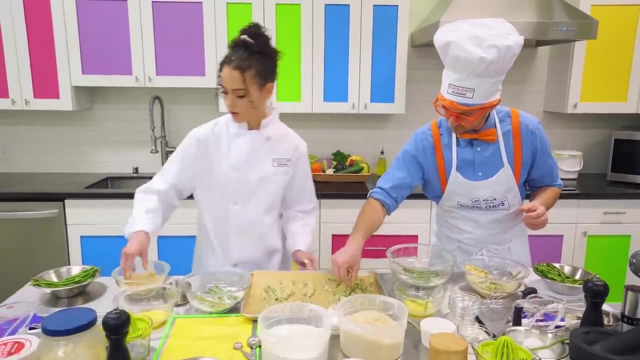 There we go. That makes sense. Oh, I see, Because if they're on top of each other then the heat can't touch the whole green bean. huh, Exactly, You wanna make sure that the Mm-hmm Okay. 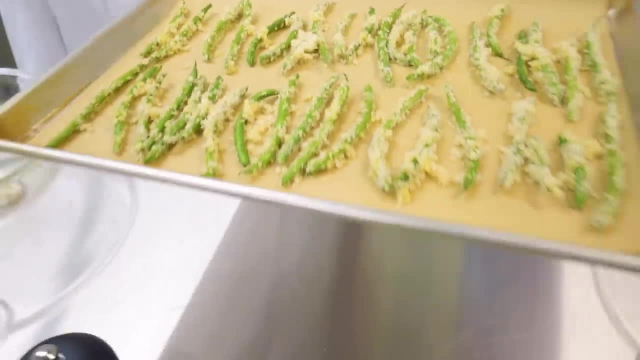 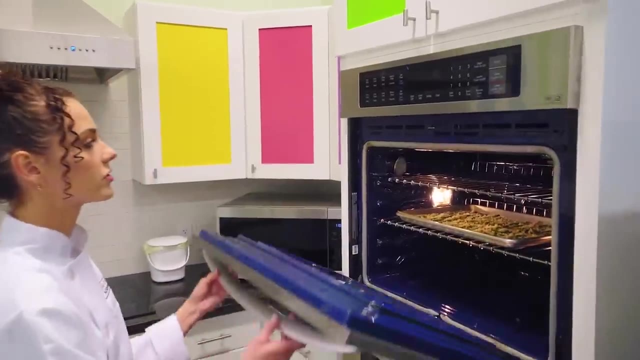 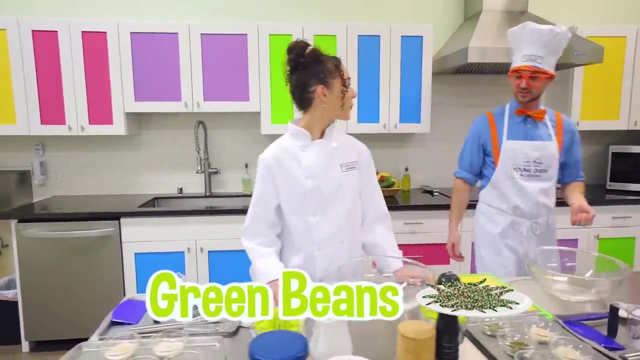 Cool thing is getting cooked. We're ready for the oven. Okay, here you go, Here you go. Thank you, Perfect. Those will take about 10 to 12 minutes to cook Whoa. that was really fun making those green beans with you, Wasn't it? Yeah? 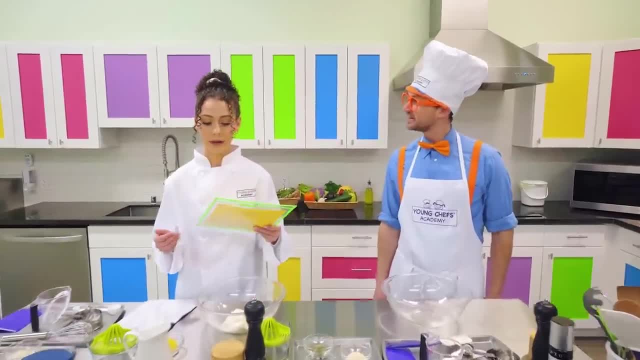 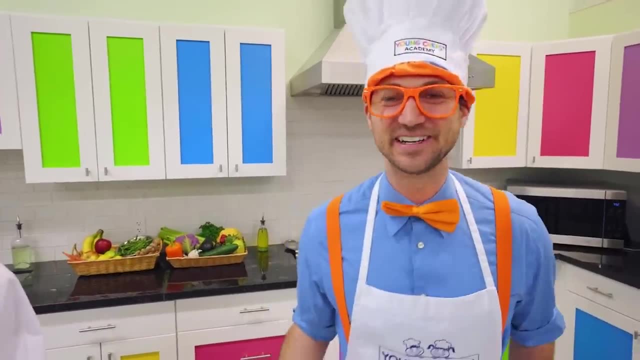 let's make some ranch to dip them in. What ingredients do we need? We need mayonnaise, sour cream, buttermilk. Wait, did you say buttermilk? Yeah, Oh, I said cream earlier. Okay, so we need buttermilk. Yes, they're very similar, but buttermilk smells different. 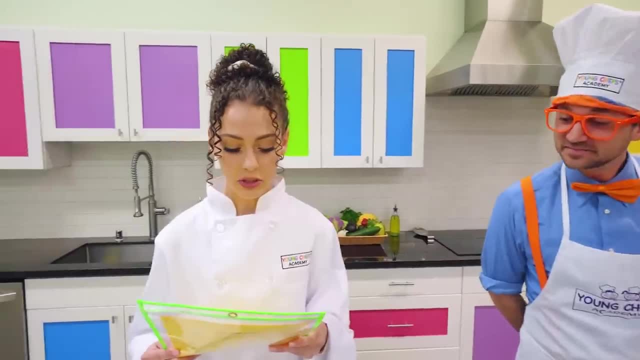 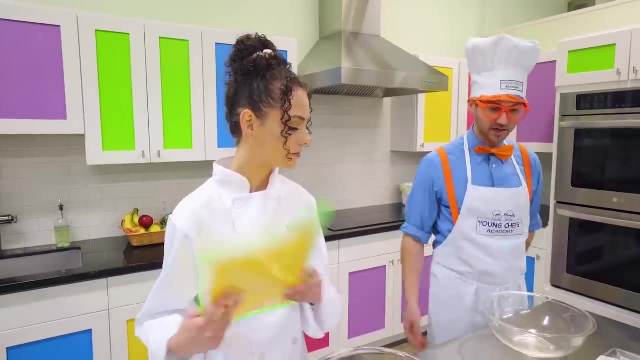 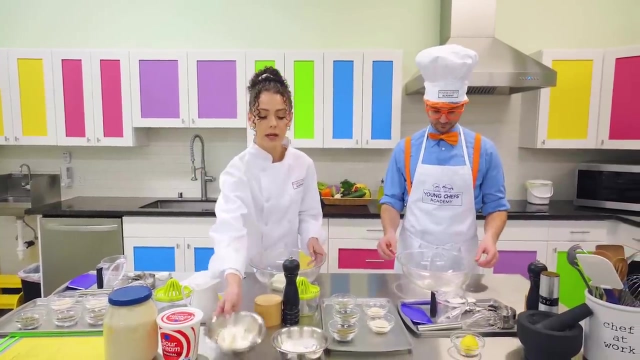 and it's a little thicker, Okay, All right. Lemon juice, dill, weed, parsley, chives, onion powder, garlic powder, salt and black pepper. Okay, perfect, Looks like we have everything I think we do. All right, next we're going to want to, So I have mine all mixed up. 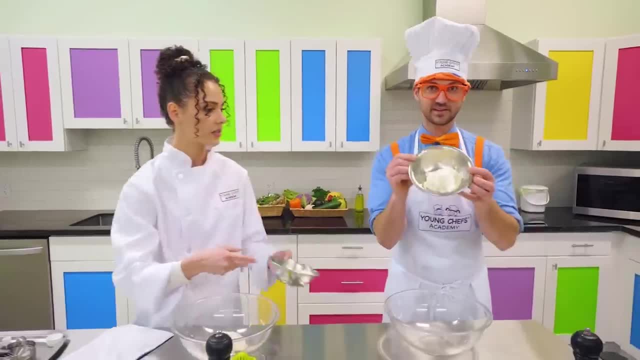 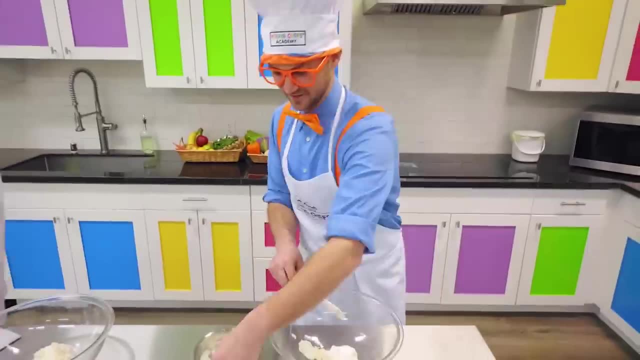 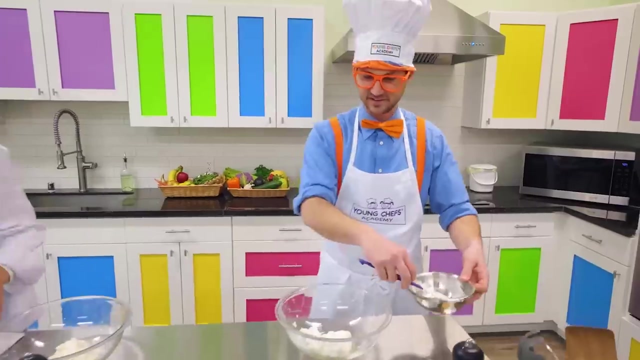 Can you put the mayo and the sour cream into your big bowl? Okay, here's the mayo, And then we have the sour cream. All right, there we go. Awesome. Now we're going to want to do half a cup of buttermilk. 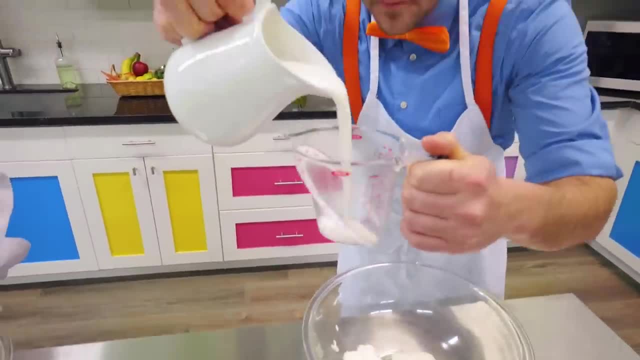 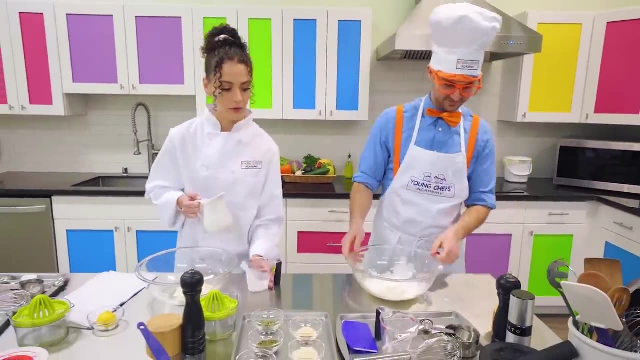 into your bowl. All righty, There we go. Perfect, All right, now we're going to want to get our one-fourth teaspoon. Okay, there we go. All right, now we're going to want to get our one-fourth teaspoon, Okay. 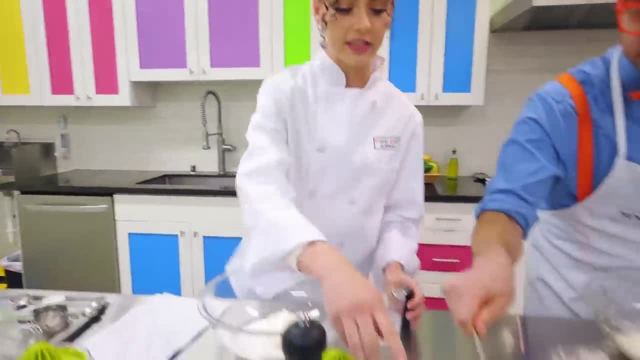 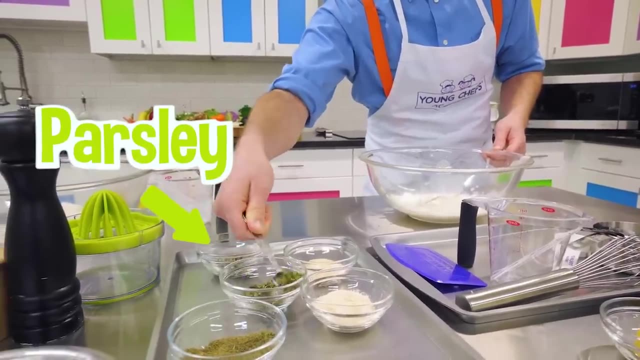 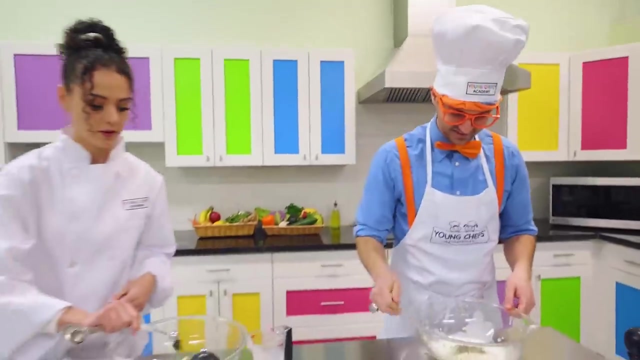 perfect, I'm ready And we're going to use that for our dill right here: parsley and our chives. Okay, dill, parsley and chives. There we go. Good job, puppy. Next we're going to want our. 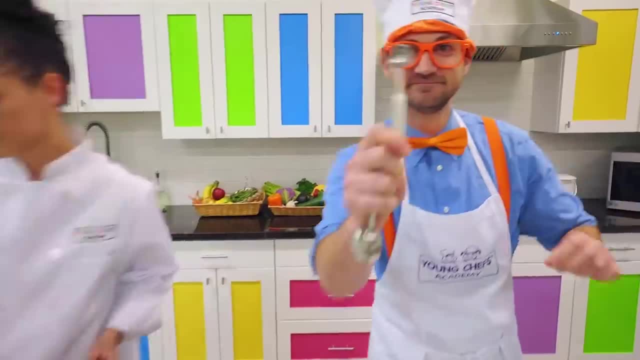 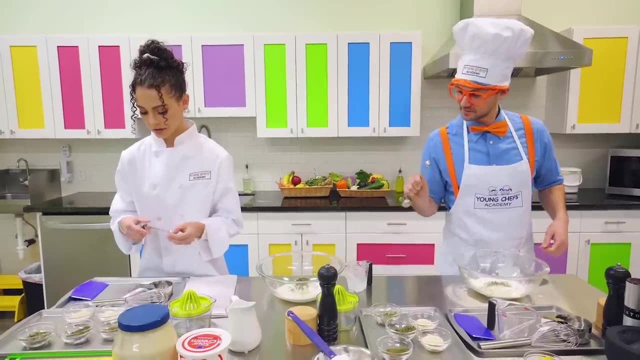 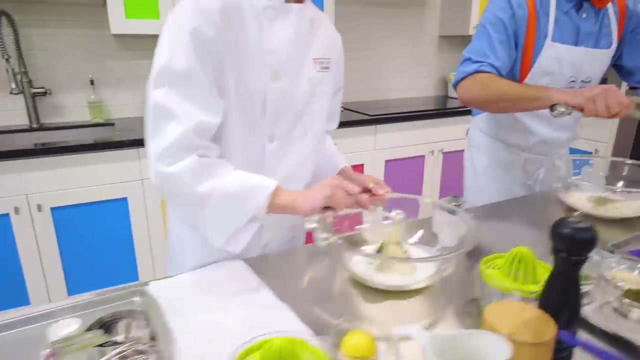 half teaspoon. Okay, a little bigger, All right. All right, and we use that for our garlic powder, garlic powder, and our onion powder And our onion powder, garlic powder. All right, Let's give it a little scoop. 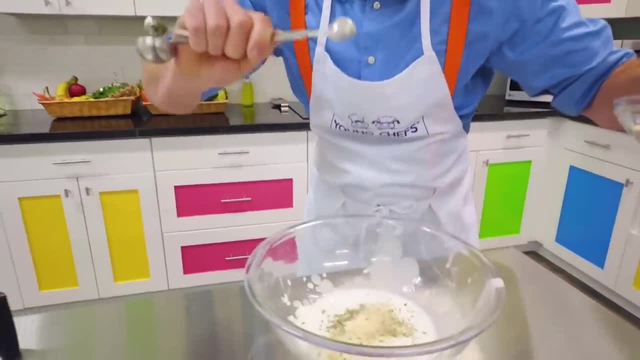 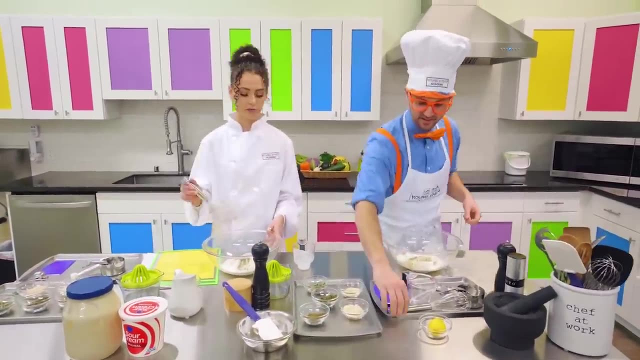 And then this one- Perfect. This is going to be so yummy. And then this one: Perfect. This is going to be so yummy. All right, perfect. Let's mix that up with our whisk- And don't forget, we whisk with our wrist. 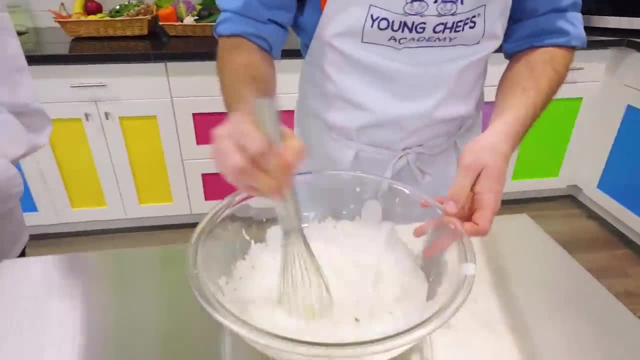 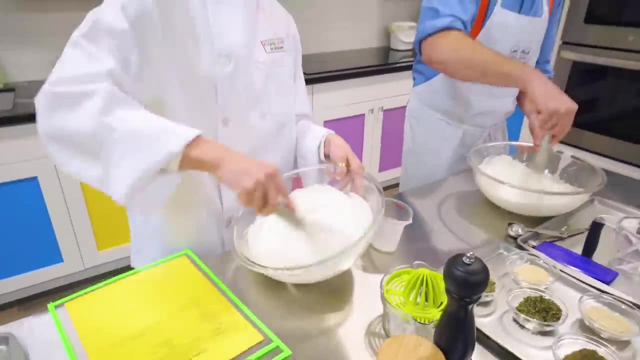 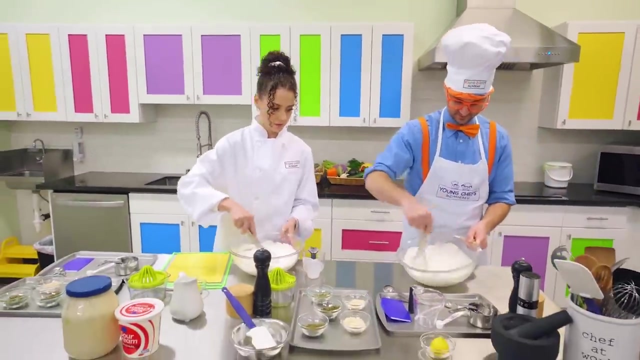 All right, Woo, Woo, Woo, Woo, Woo Woo. This smells so good. Woo, Woo Woo. Once it's all mixed up, we're going to cover it and place it in the fridge to cool. All right, we only have three more ingredients. 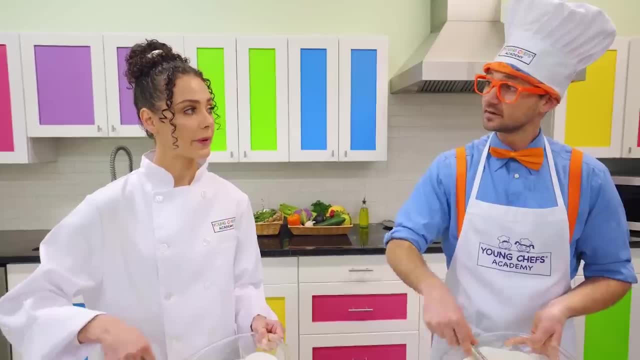 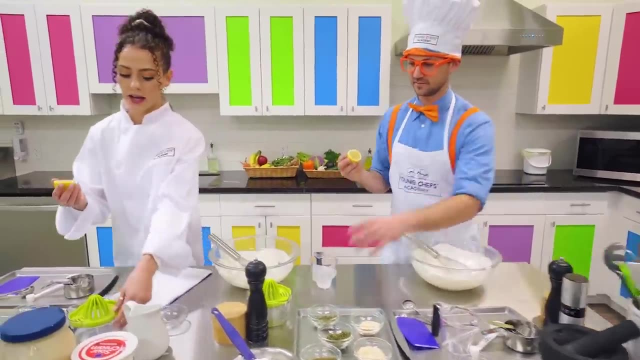 Okay, what are they? Lemon juice, salt and pepper. Okay, First we want to juice our lemon. Okay, So you have a lemon right up there. Perfect, We have it cut in half and we'll use our juicer here. 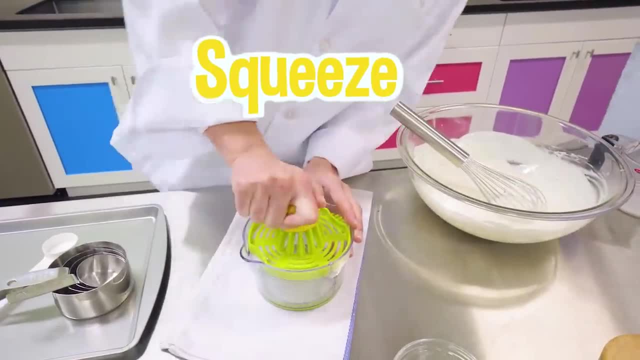 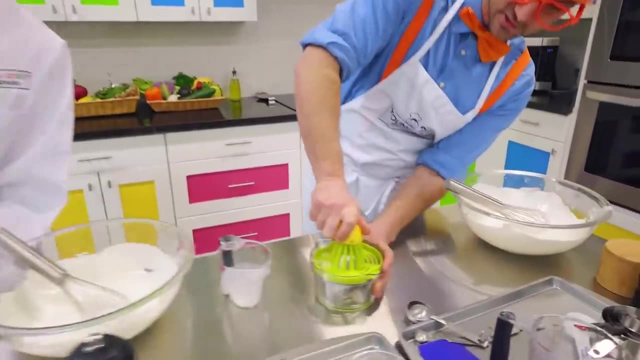 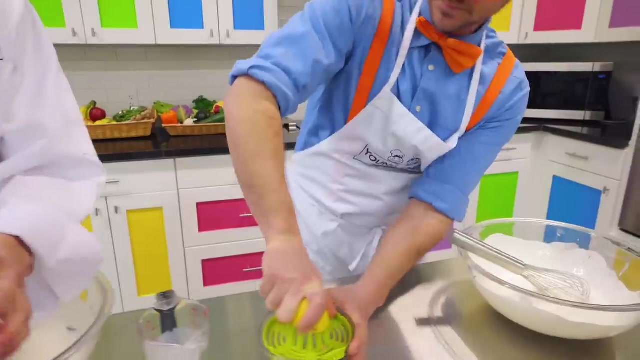 We want to make sure we squeeze really tight, pushing down and twisting it around to get all of that juice out. Okay, I guess I'll try it. There we go. Good job. Yeah, When you take it off, your lemon should look something like this: 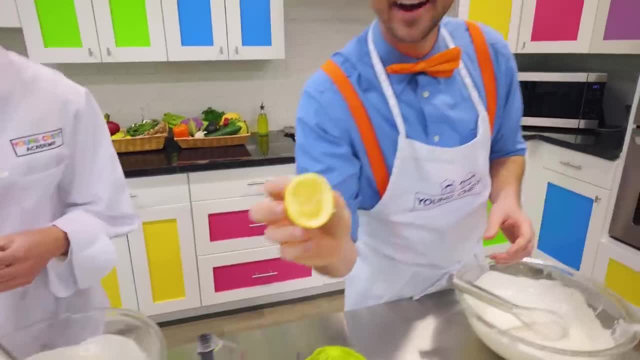 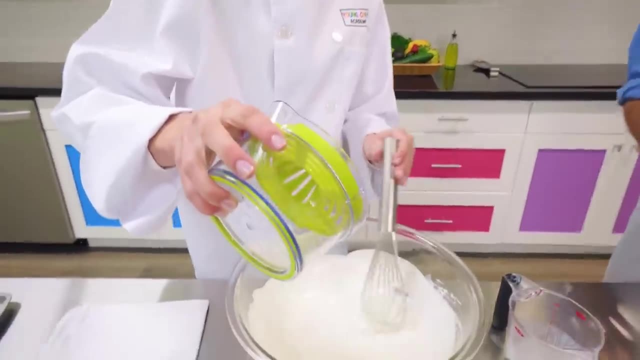 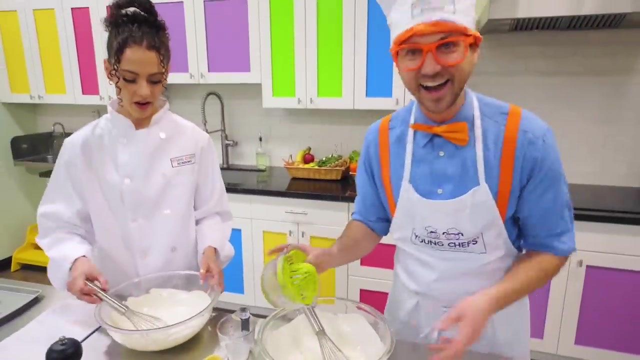 Yeah, It's almost empty. Perfect, Good job. Okay, And it's done for you. And then we want to pour our lemon juice into our ranch. Okay, Here we go. Wee Awesome, Mix that up, All right. 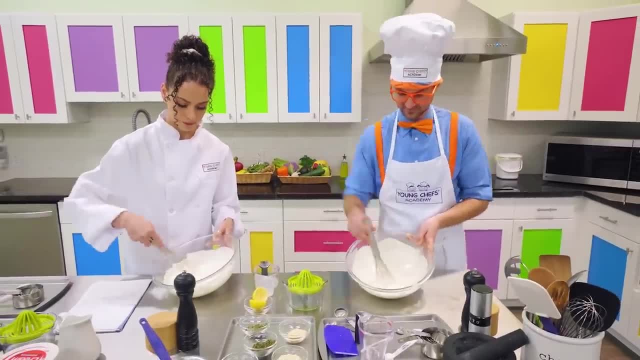 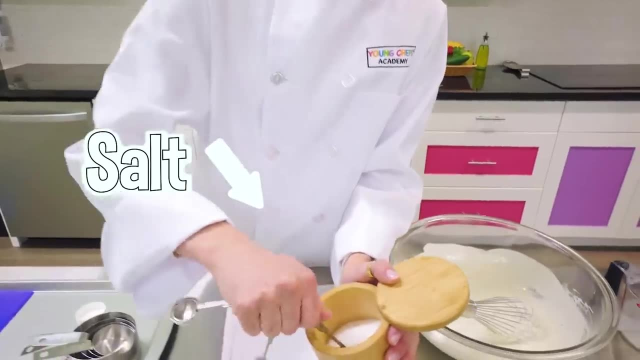 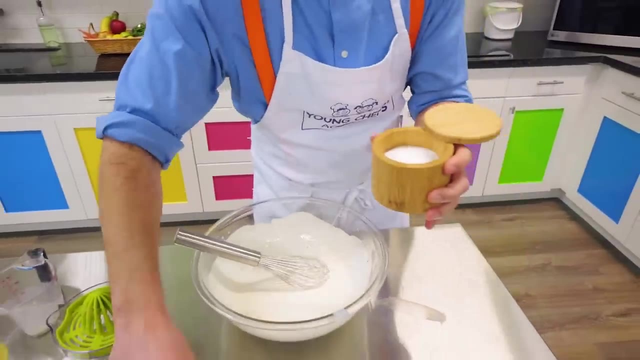 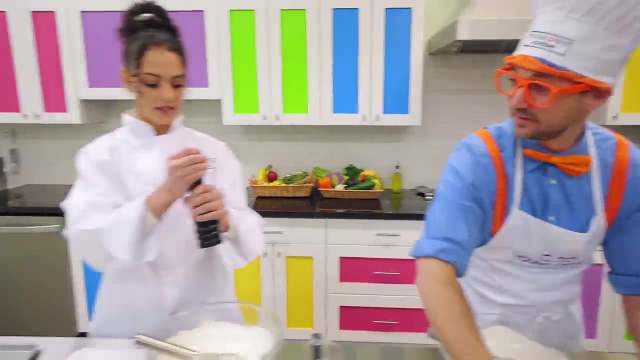 Yum, Now we want to do one fourth teaspoon of salt, Right like this. Okay, Put some salt in here. Here we go, Wee, And here we go, Wee. There we go And a pinch of pepper. 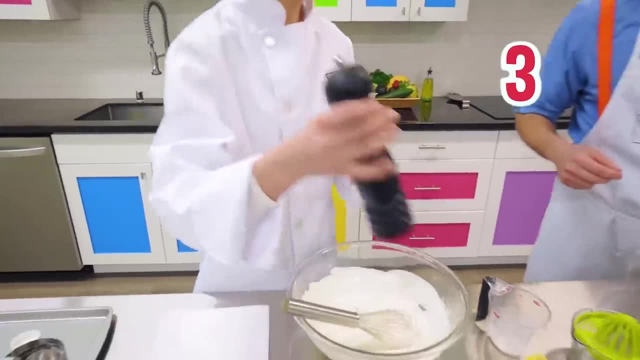 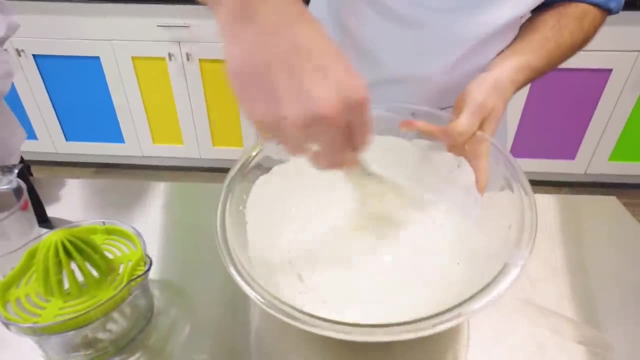 So we'll go about three twists, Okay, One, two, three, Perfect, Perfect. All right, Let's mix that up. All right, Mix, mix, mix. Remember to mix with your wrist. Oh yep, Oh wow. 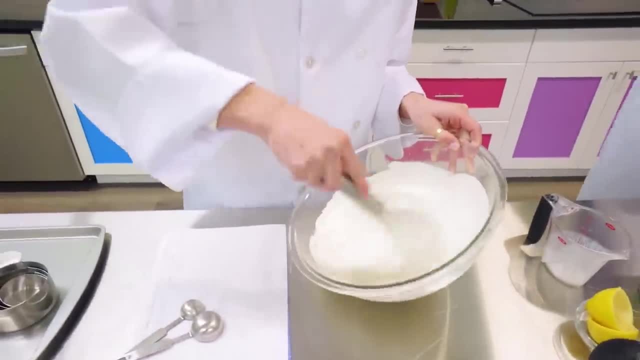 This is going to be so yummy, Delicious. Did you hear that I did? Does that mean the green beans are done? It? does You want to grab them? Sure, Oh, this is going to be awesome, Oh, wow. 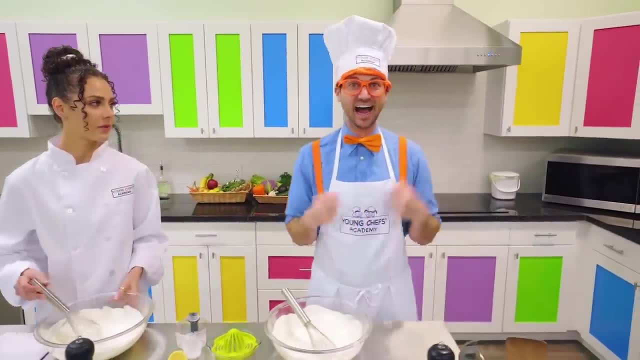 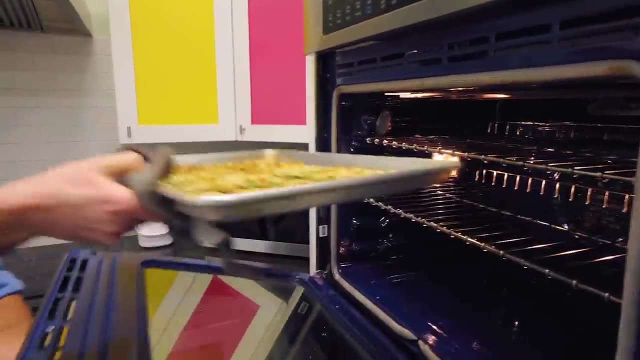 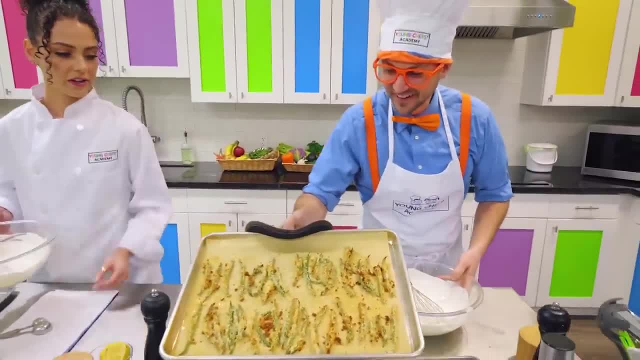 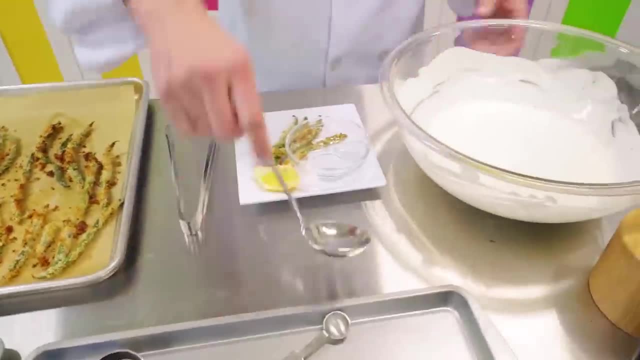 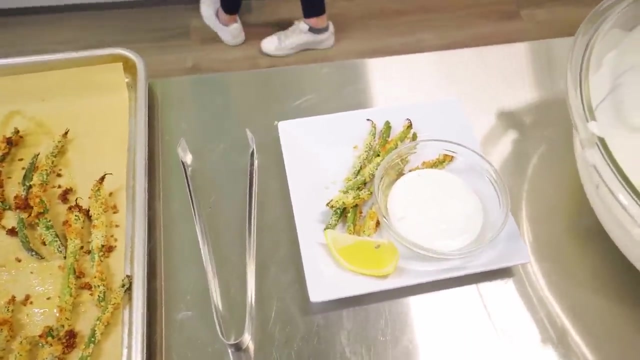 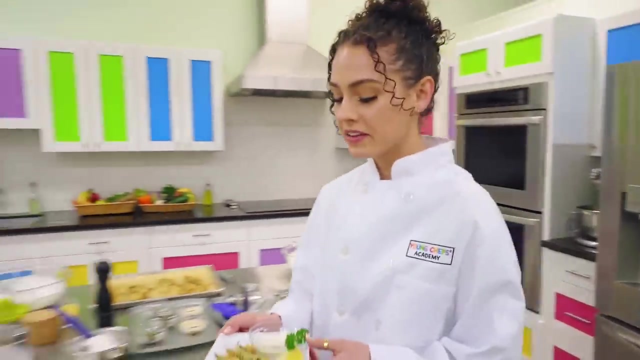 Check them out. Oh my gosh, Let's see. Oh my gosh. Hey, that's the stitcher. All right, Blippi, it looks like our green beans and zesty ranch are all ready. They look so good. 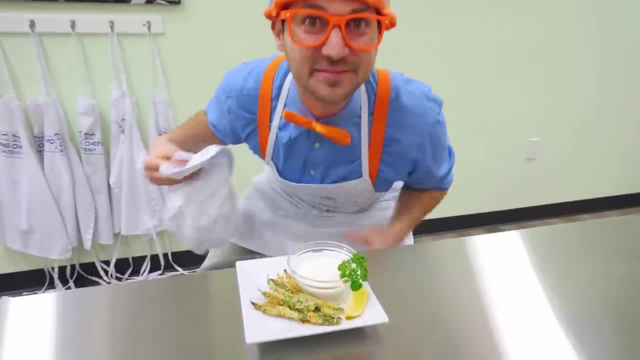 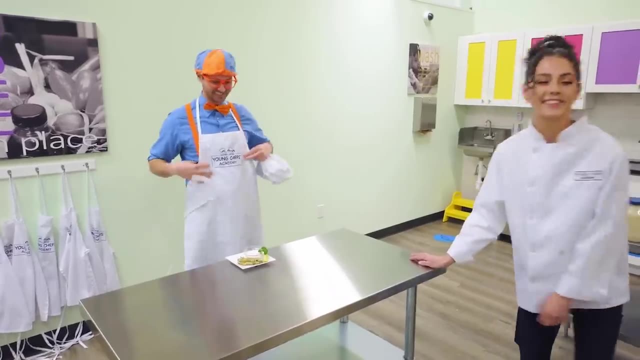 Those look yummy. Check them out. Whoa, I am so excited. Thank you so much for teaching us how to bake these. Of course, you did such a good job. Come back every time, Oh well, thank you, See you later. 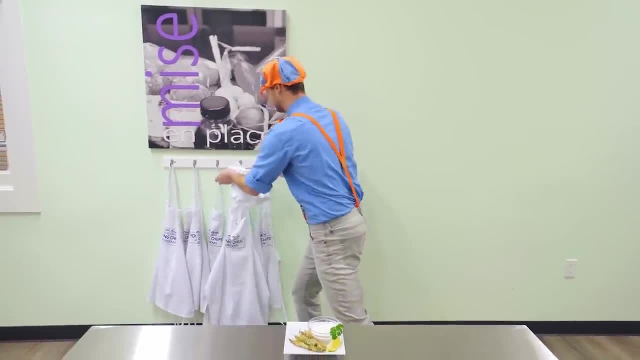 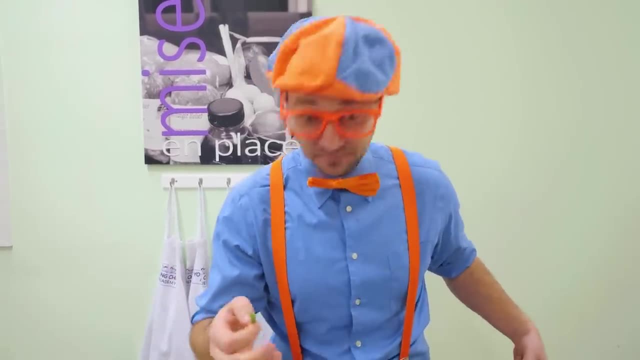 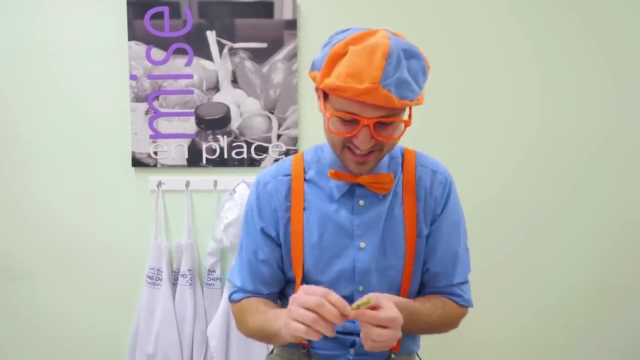 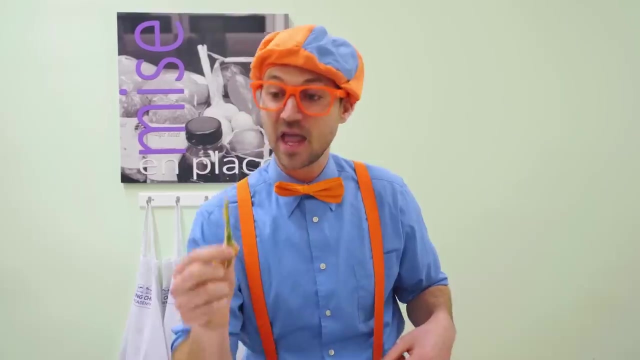 See you. Wow, I am so excited. Here we go. Mmm, Mmm, Yum, That is dippalicious. So silly, Yeah, you'd think, because they're greens, they're not good. Hmm, But hey, trust me, it's really fun to try new types of foods. 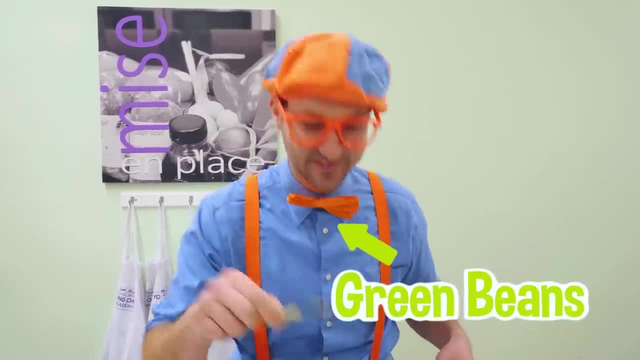 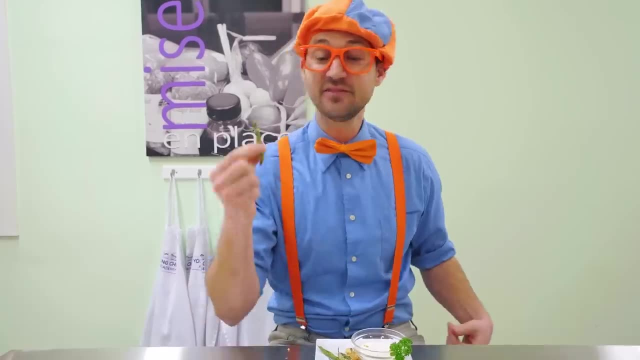 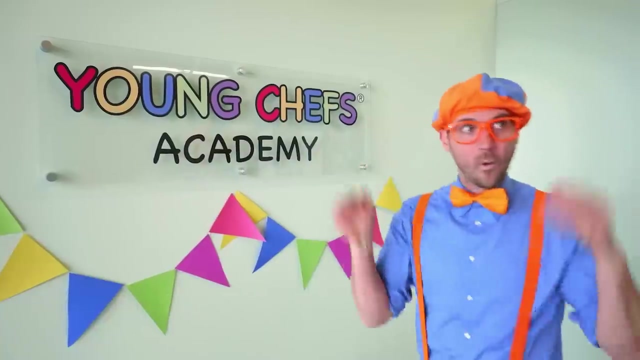 Yeah, like these yummy green beans that we made. Yeah, Mmm, Mmm, Mmm, Yum. Even healthy foods can be really yummy. Good job cooking, Whoa Yee-haw, Blah, Blah. 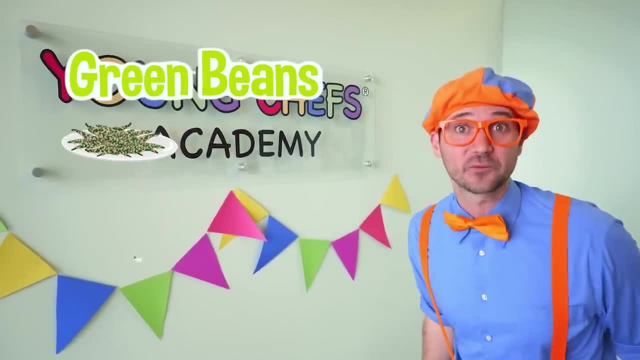 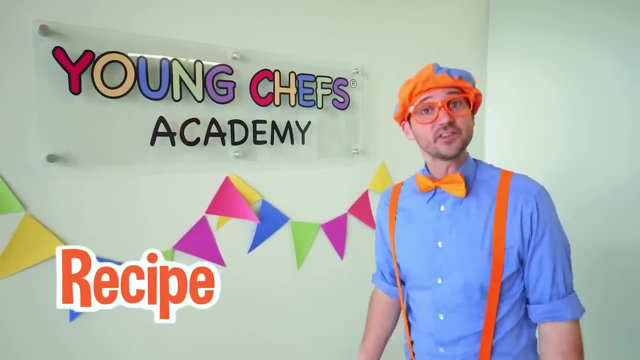 Ha-ha, Wasn't that fun making those green beans and that ranch. Did you like the green bean sauce? Yum, It was so tasty. Hey, if you want to check out the exact recipe, you can go to Young Chefs Academy website. 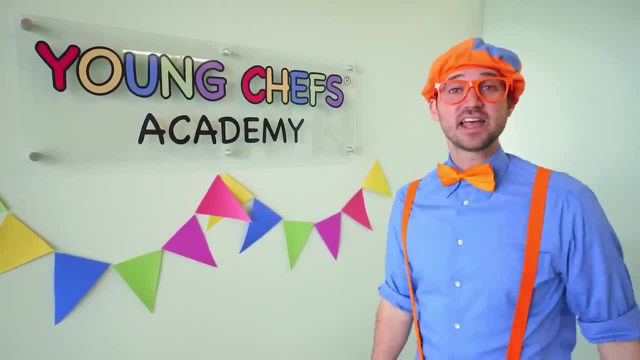 and check out their blog, Woo-hoo. Well, this is the end of this video, But if you want to watch more of my videos, all you have to do is search for my name. Will you spell my name with me? B-L-I-P-P-I. 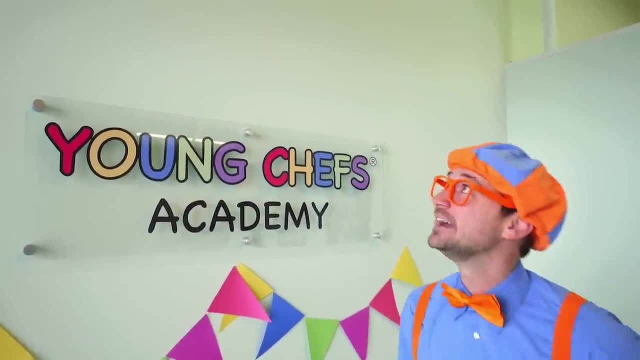 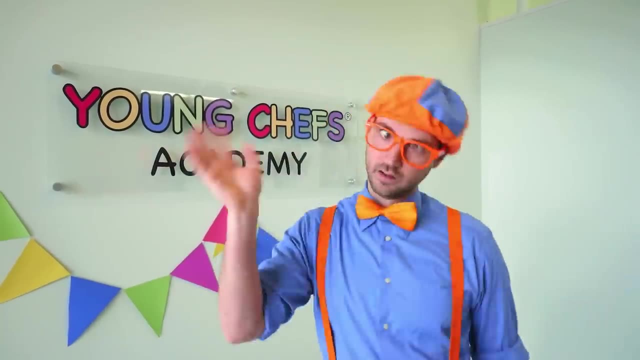 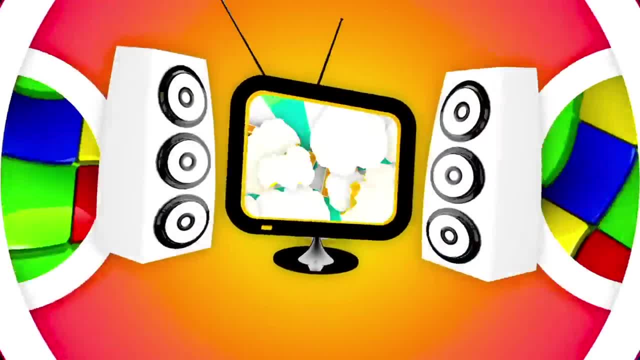 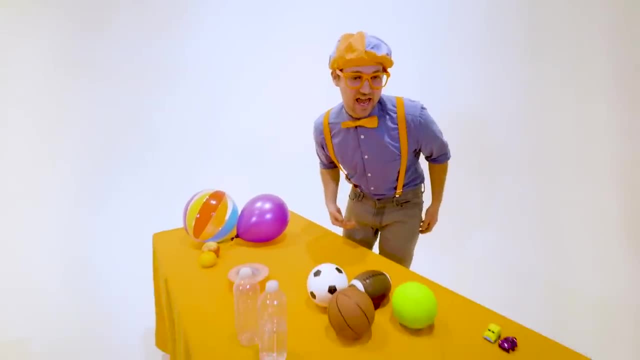 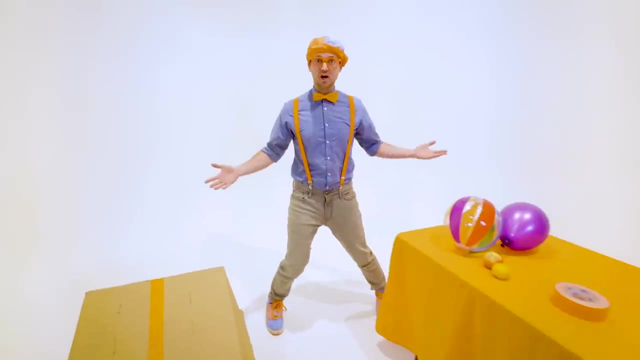 So much to learn about Blippi. It's me Blippi, And look at all the items that I have. Whoa, So many random things. But hey, in this video we are going to do the Blippi Velocity Race. 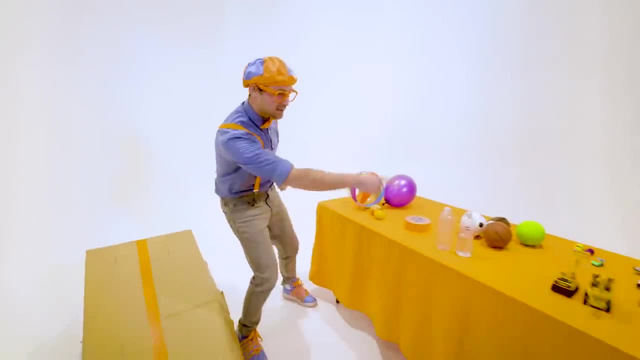 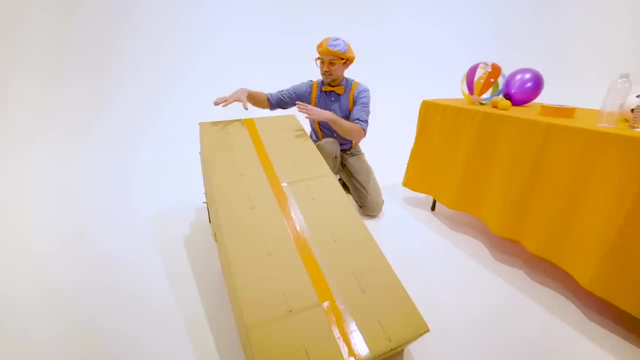 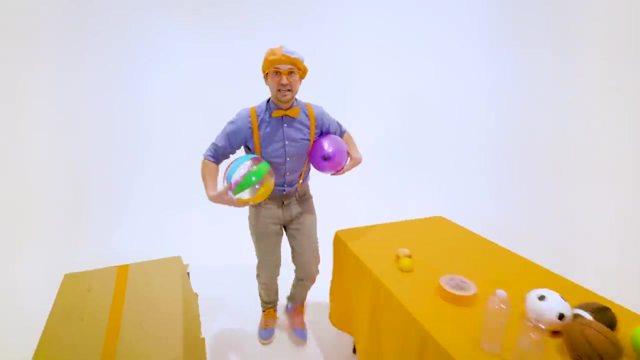 Yeah, That's where we put a lot of these items on this ramp. Yeah, See how this ramp is at an angle. Yeah, we're going to let them go at the same time and see what item reaches the bottom first. Okay, so let's go with heat number one, the slow pokes. 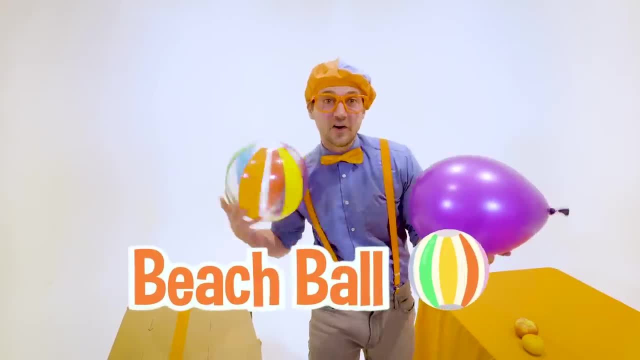 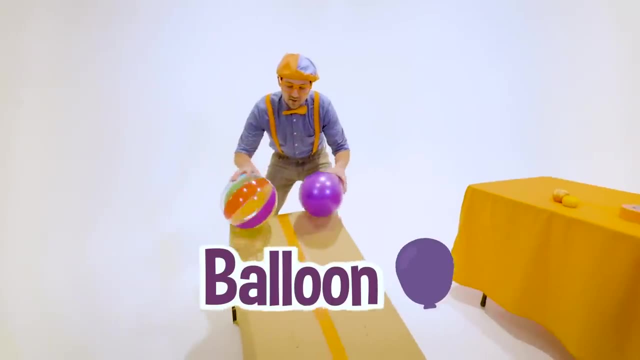 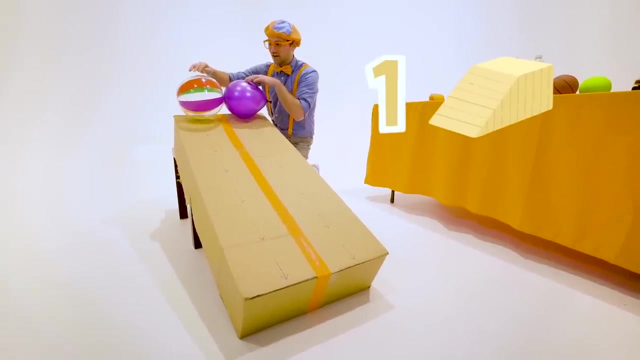 We have this sweet colorful beach ball and then we have this really light balloon. Okay, all right, What one do you think is going to reach the bottom first? I think I know Three, two, one. Whoa, did you see that? 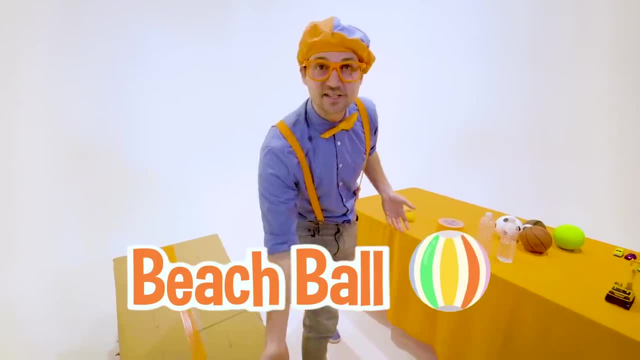 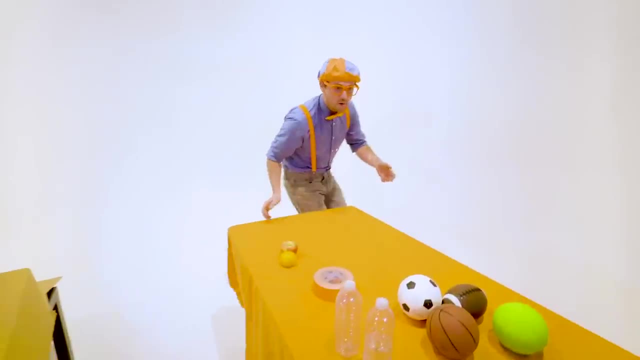 Yeah, the beach ball went to the bottom first. Okay, let's let them just, you know, get warmed up for later, and then we'll use some more items. Yeah, I'm sure all these items are going to be a lot faster. 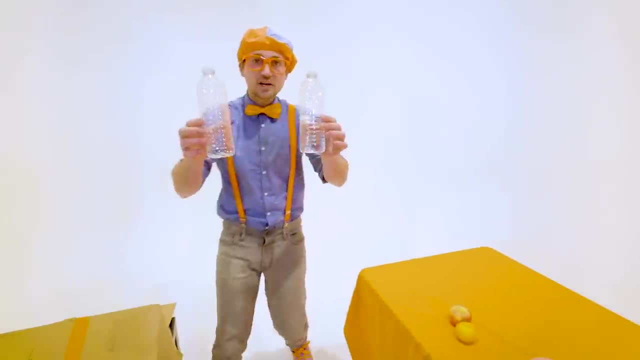 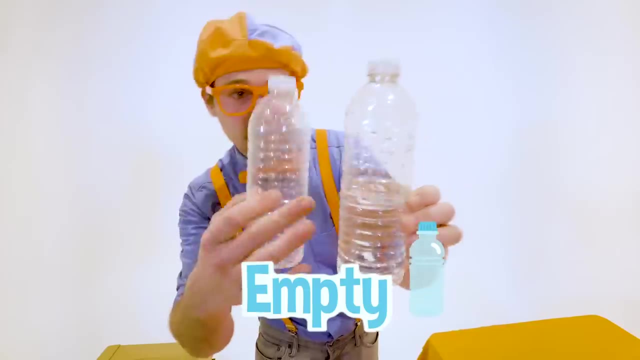 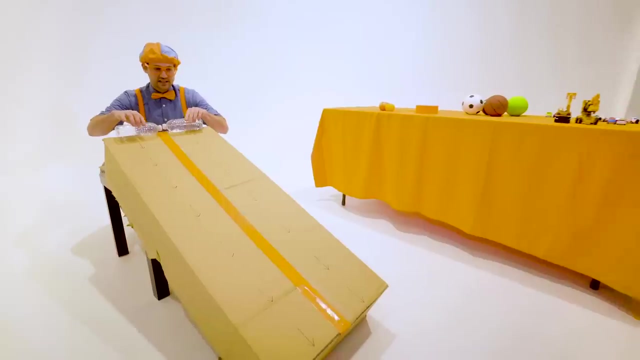 Okay, here's another set of items. They're actually the same item: water bottles, Yeah, but this one is empty And this one It's half full. All right, let's put them on their side and then let's let them roll down. 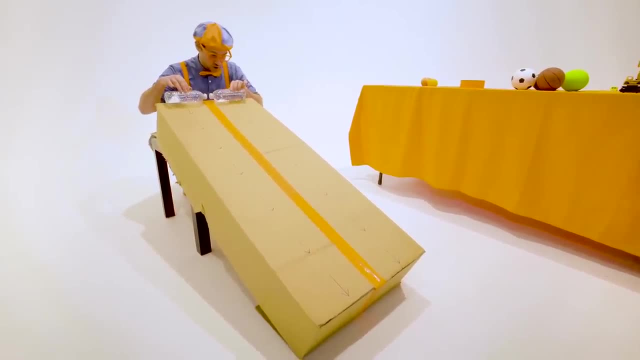 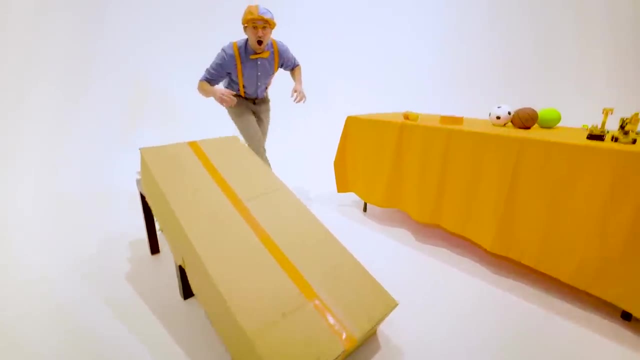 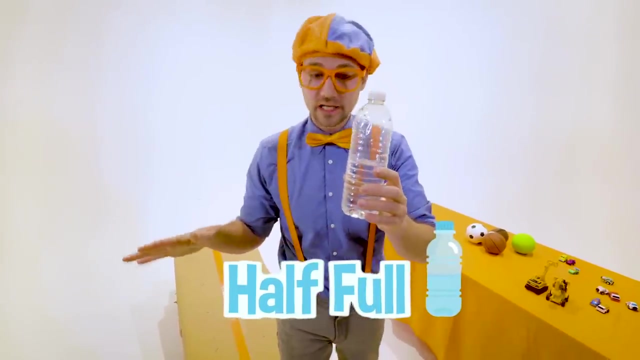 Okay, are you ready? Yeah, I'm ready. Are you ready? Oh, I'm ready? Awesome, Three, two, one, Whoa, yeah, Wow, Wow. the half full water bottle totally beat the empty water bottle. 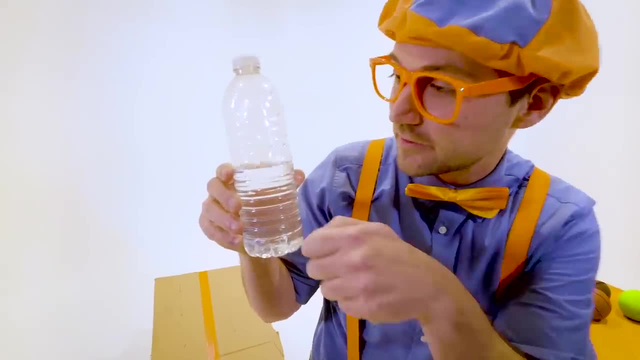 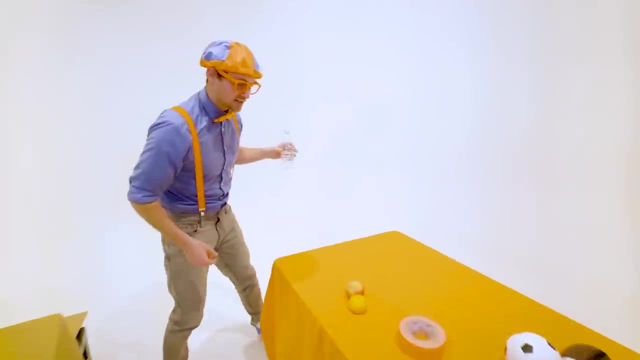 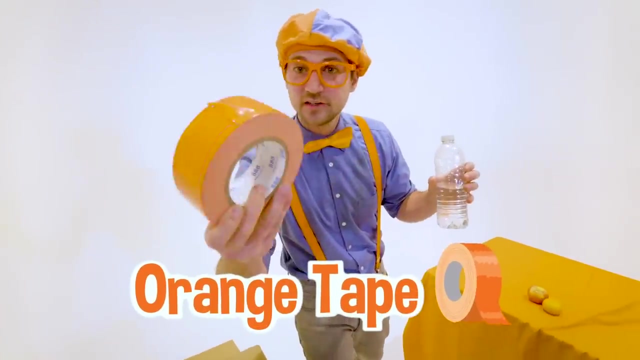 How do you feel? How do you feel after your race? half full water bottle. Oh, Blippi, I feel amazing. I can't believe I've won. Great. Well, it's going to move on to the next race. Half full water bottle versus extremely bright orange duct tape. 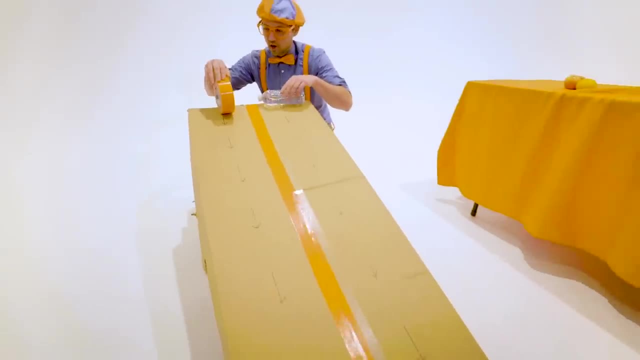 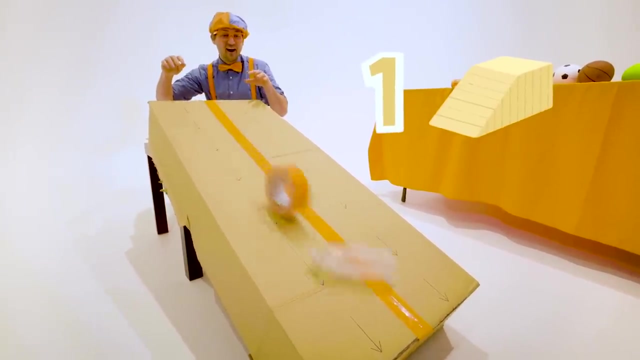 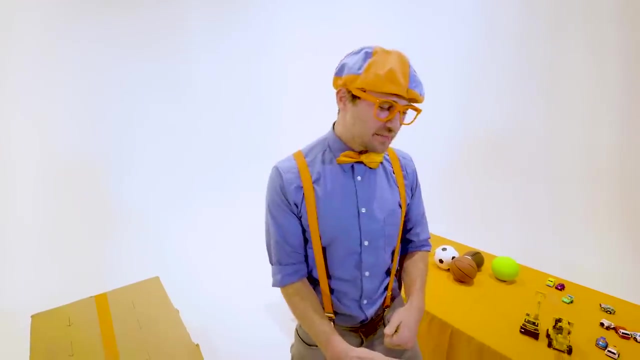 All right, here we go. Are you ready? Ready to race? Are you ready? You know I'm ready. All right, three, two, one, Whoa, Whoa. Did you see that? Yeah, The water bottle rolled down way to the bottom way quick, way, faster than the duct tape. 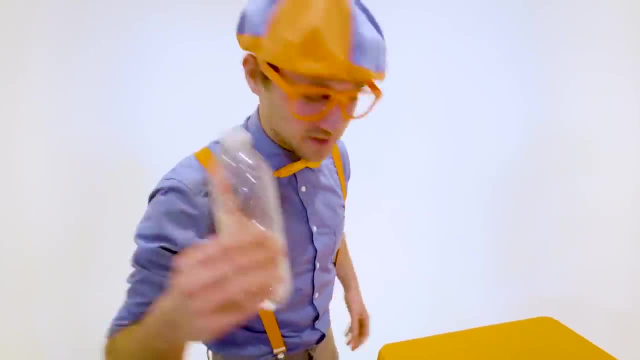 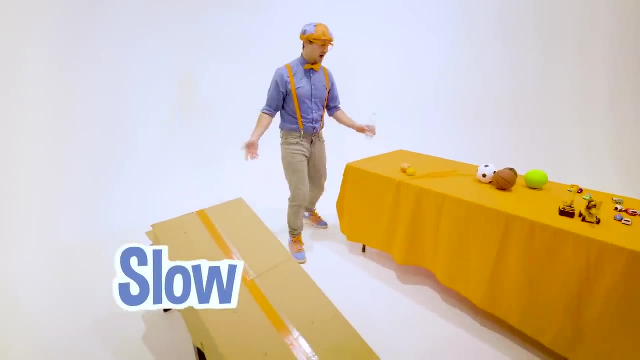 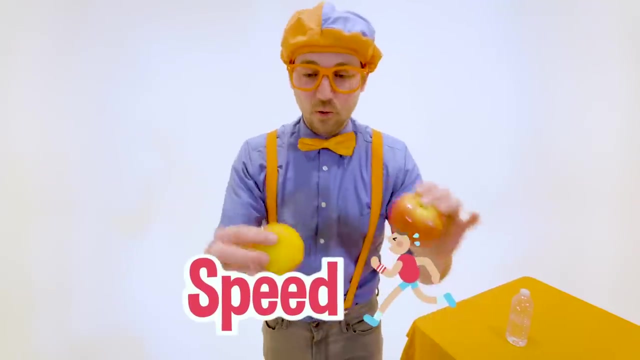 Perfect, So now it can move on to the next round. Have you ever wondered why these items some go fast and some go slow? Yeah, it's because their velocity. yeah, velocity is basically the speed at which they're rolling down. 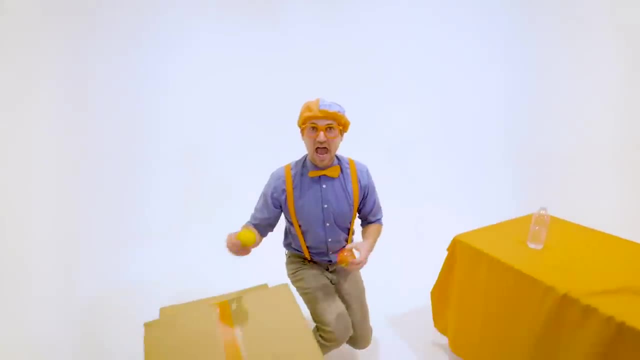 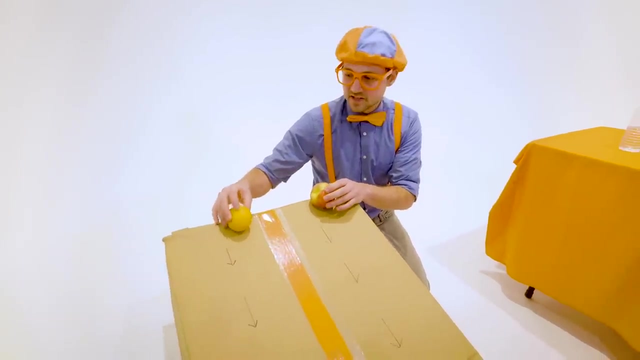 The speed and the direction. Yeah, there's a lot of things that actually determine what the item's velocity is. I mean, like, think about it like this: There could be a lot of friction and it like can't slide, or maybe it rolls, compared to. 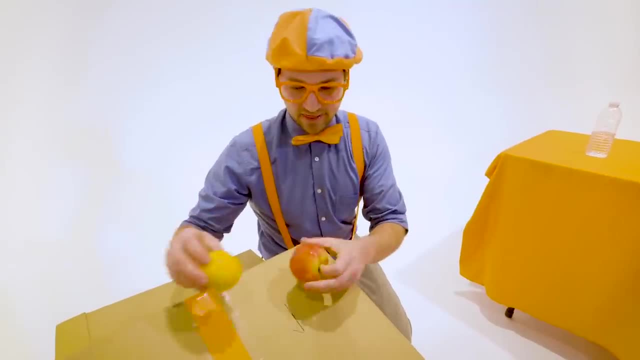 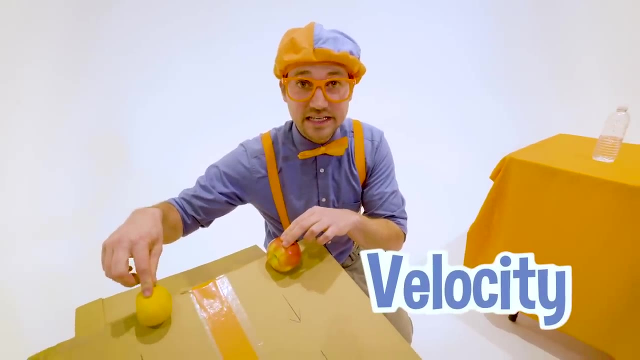 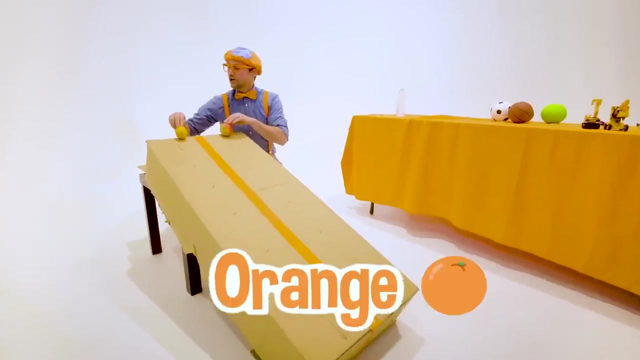 you know, maybe there's sharp edges. There's just so many things that you know determine how fast, how much velocity these items have. So let's let these two items go. We have orange over here and apple over here, and let's see who wins. 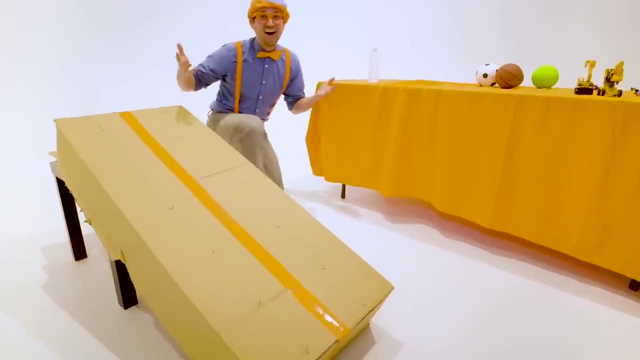 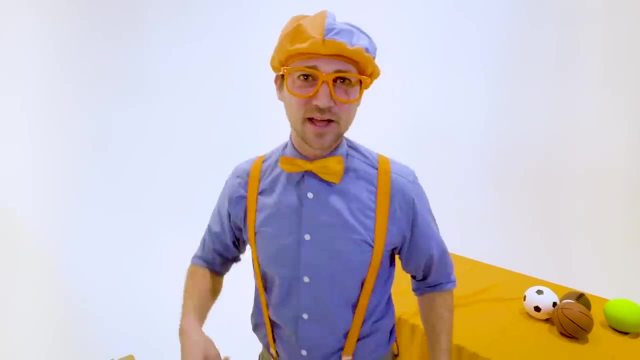 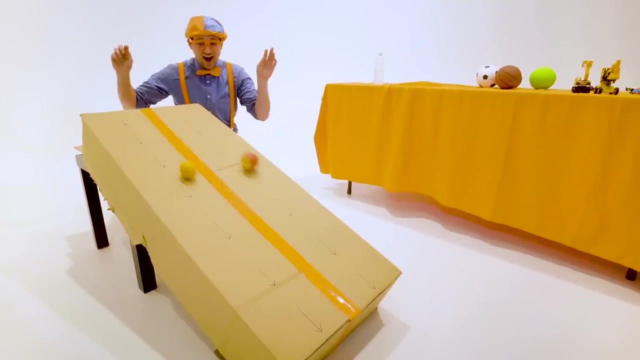 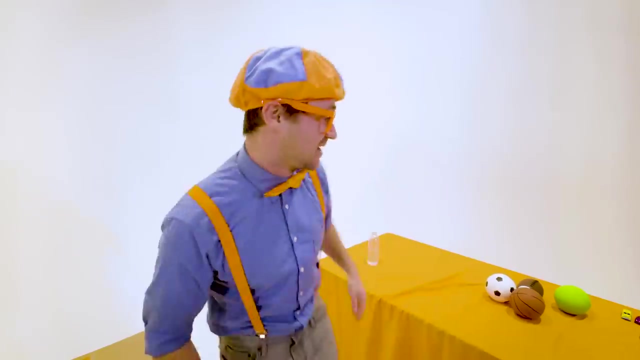 Go Whoa, They were actually really close to each other. I don't even know who won. Let's see that instant replay. Whoa, That was awesome. All right, Let's pick two more items. We have a soccer ball or a football, depends where you live- and the half full water bottle. 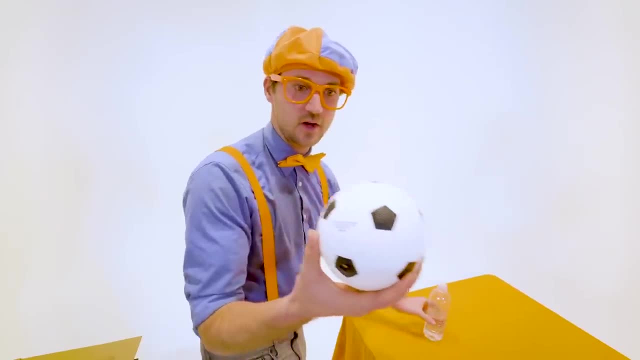 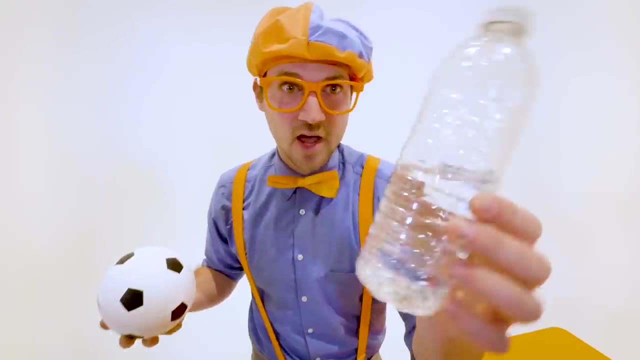 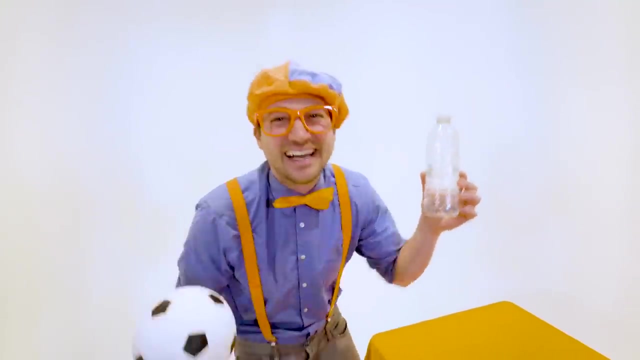 The champion. Yeah, That was awesome. All right, Let's pick two more items. We have a soccer ball or a football, depends where you live- and the half full water bottle. The half full water bottle. That's it Good. 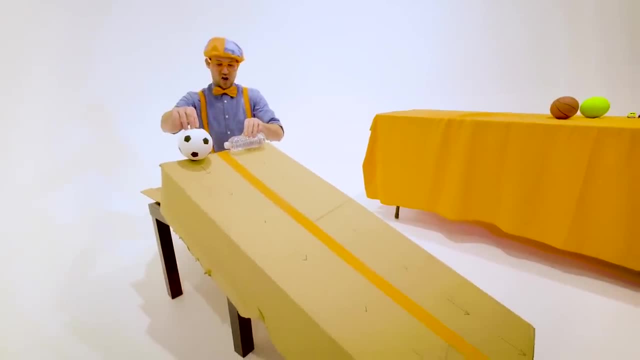 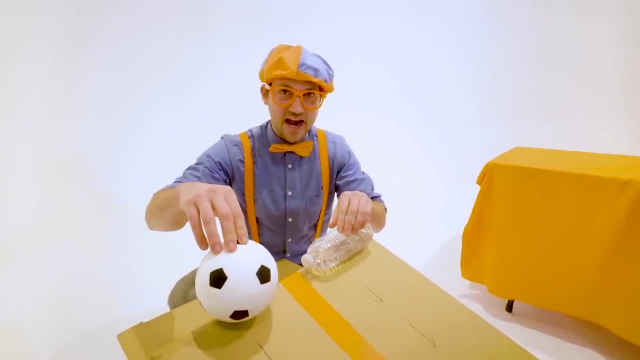 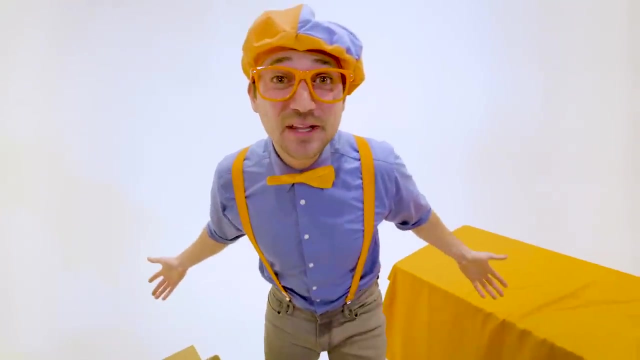 Okay, Let's see who wins. All right, Here we go. Are you ready? I'm good to go. Are you ready? I was born ready. All right, And away we go. Whoa, I cannot believe it. The half full water bottle wins the velocity race. 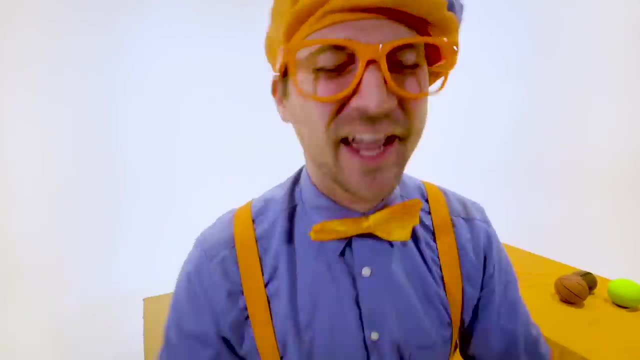 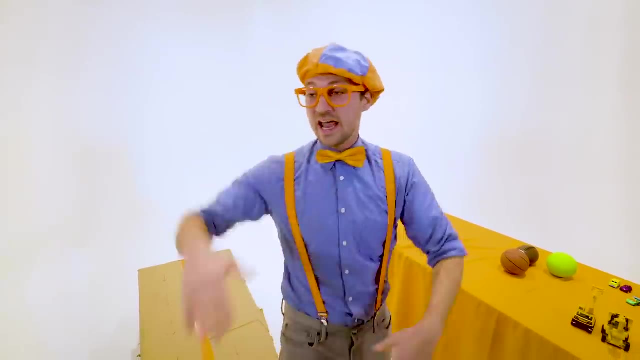 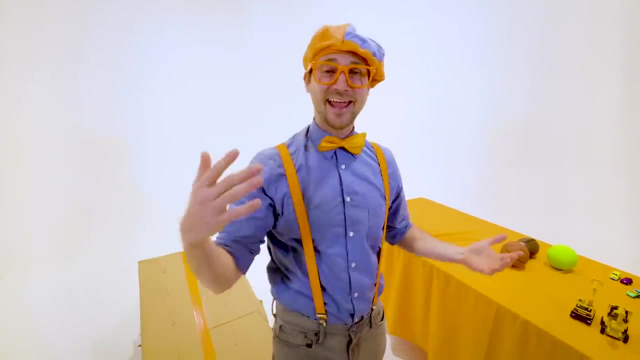 Whoa, That was awesome learning about velocity and how fast that water bottle went and how the ramp is angled. But yeah, if the ramp was flat it definitely wouldn't go anywhere, right, Yeah, Hey, can you think of a machine? that is actually really fast. 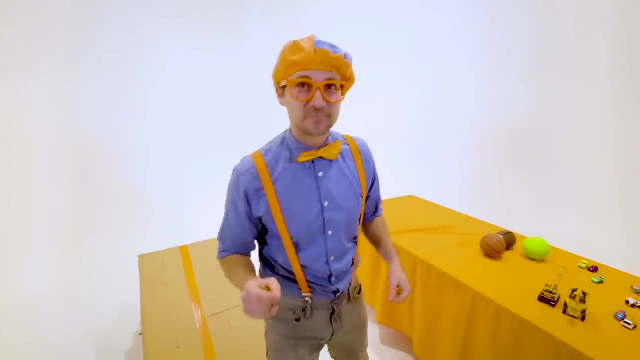 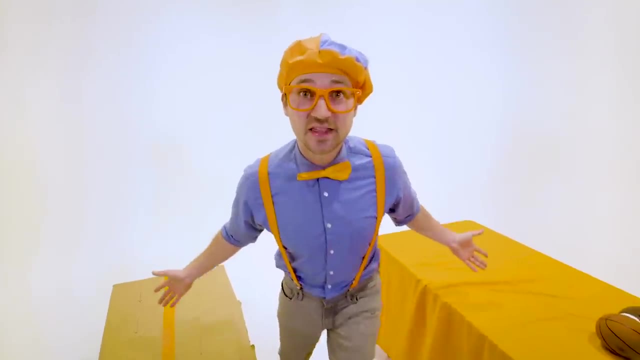 Yeah, there's a lot of them. Okay, let me give you a hint. Okay, this machine does not go on the ground. Well, it does, but then it goes in the air. Yeah, Whoa, I hear one. 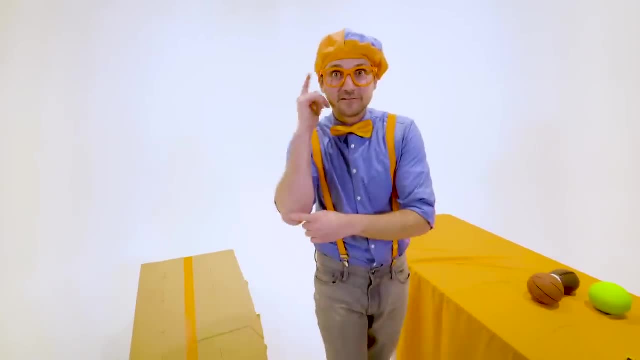 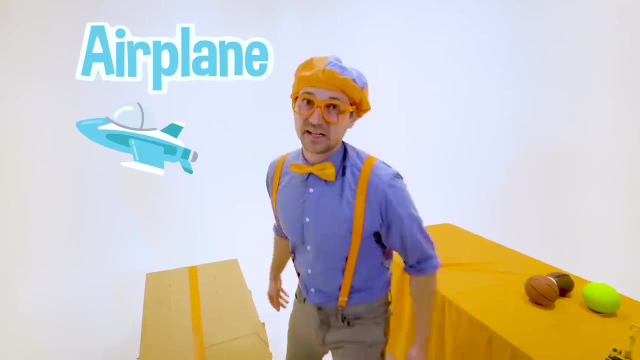 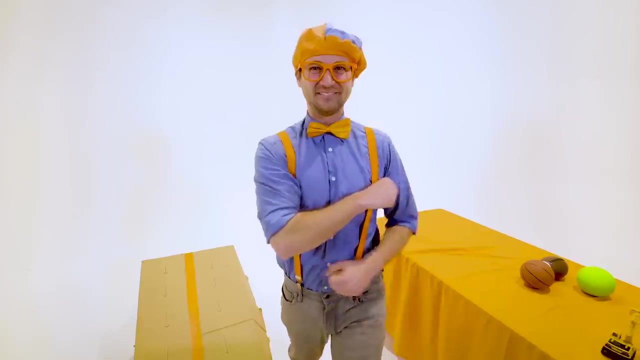 Yeah, maybe you've got to fly in one before Fly. Yeah, they fly in the air. Yeah, airplanes, Yeah, airplanes are really fast. And speaking of speed and velocity, I think you and I should watch this Airplane video. 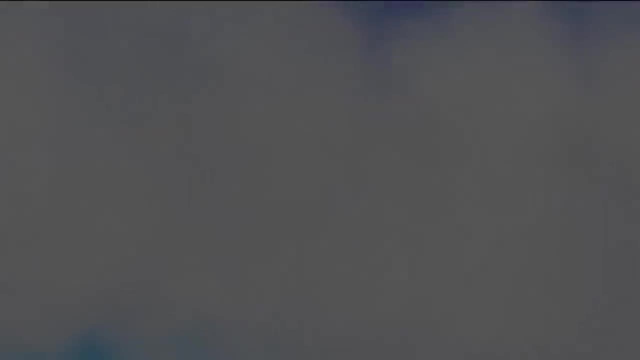 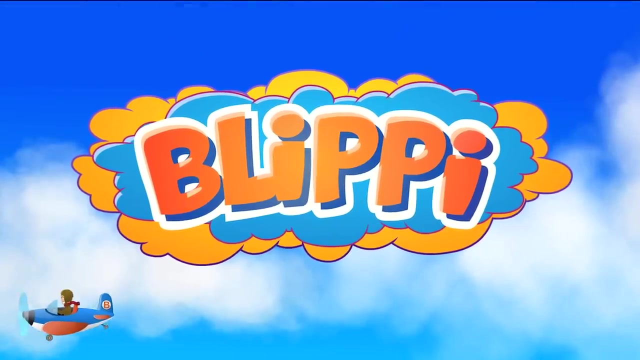 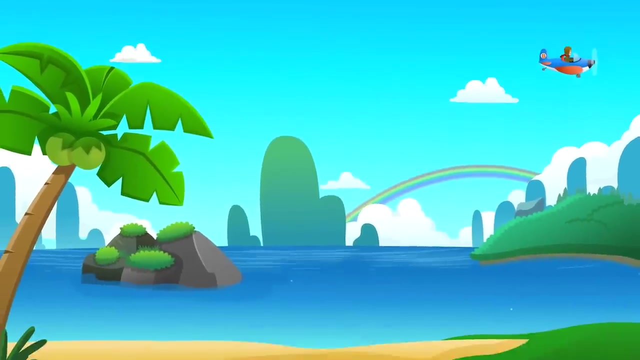 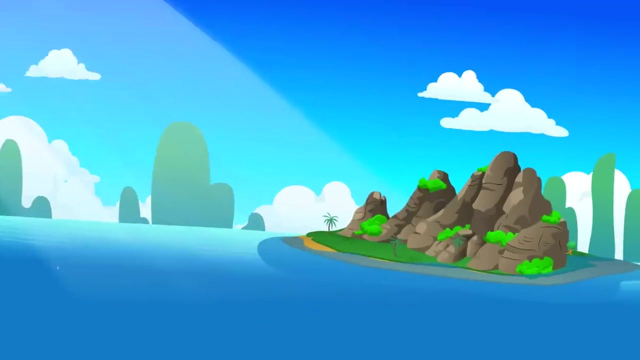 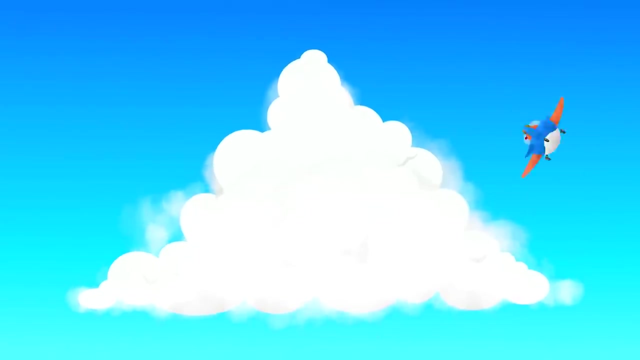 Woo Woo Airplanes, airplanes flying all around the sky. Airplanes, Airplanes flying way up high. Some airplanes are as big as a building. Some are as small as a car. That's amazing. Some airplanes transport people. 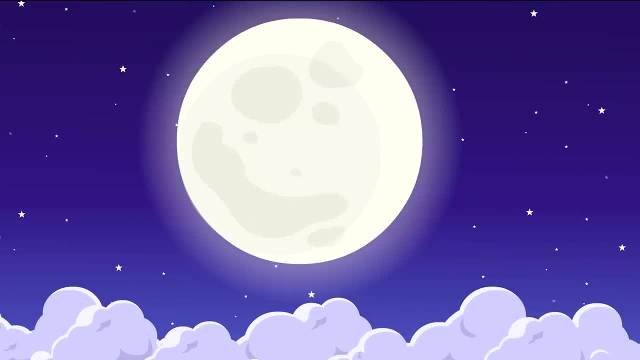 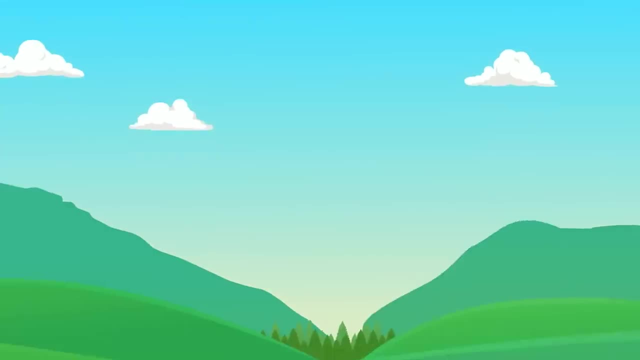 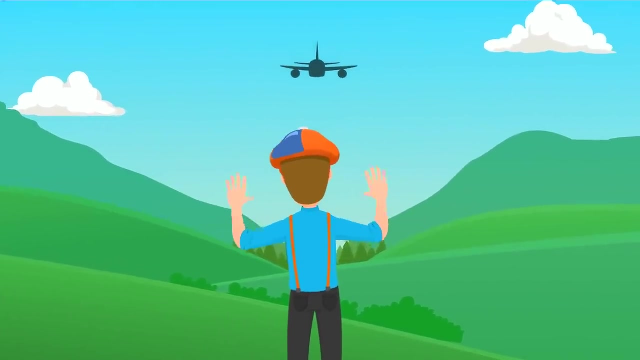 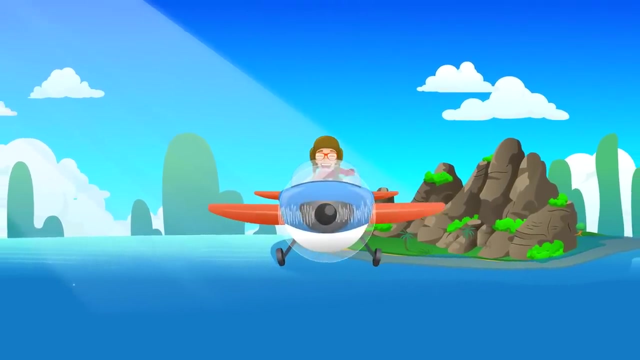 Some fly near to the stars, That's far. Some airplanes fly with propellers. Some airplanes fly with jet engines. I love to look. I love to look up and see their wings waving down at me. Hey, airplane, Airplanes, airplanes flying all around the sky. 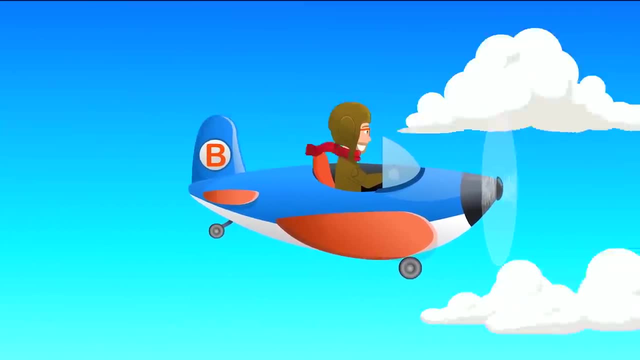 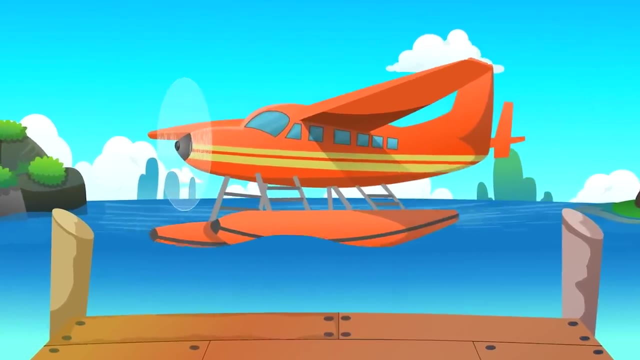 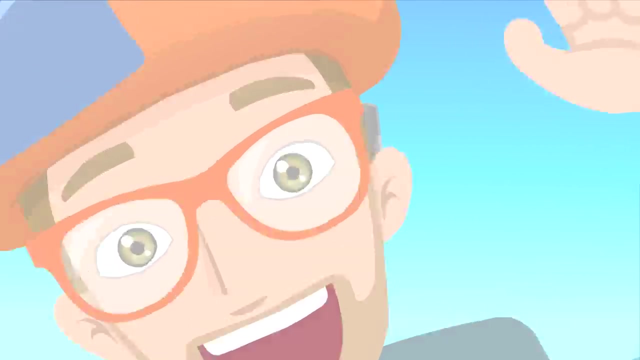 Airplanes, airplanes flying way up high. Some airplanes can land on water, but most land on landing strips, No way. Some airplanes fly just for fun. Some airplane fly just for fun. Some fly for business trips, Business or pleasure. 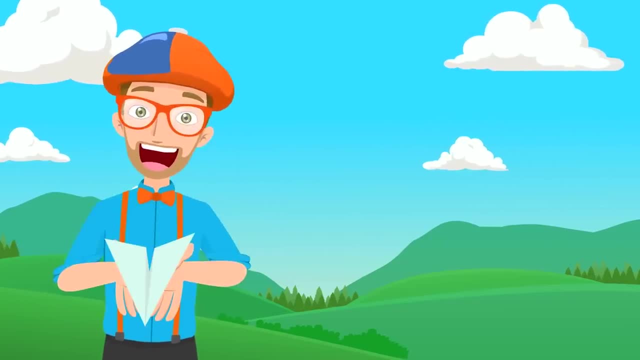 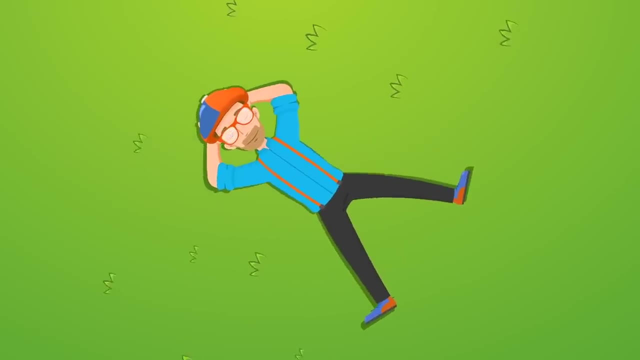 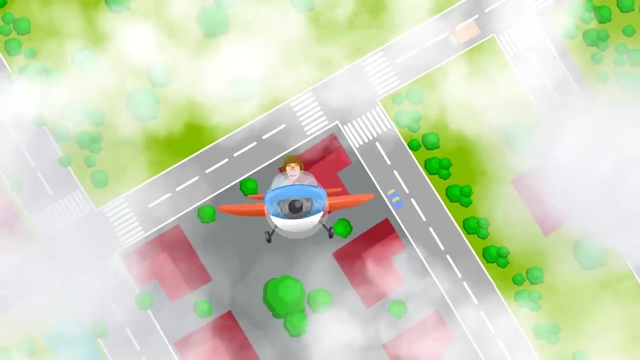 You can make an airplane out of paper, throw it in the air and watch it go. I love to look up and see its wings waving down at me. Hey, airplane, Airplanes, airplanes flying all around the sky. I love to look up and see its wings waving down at me. 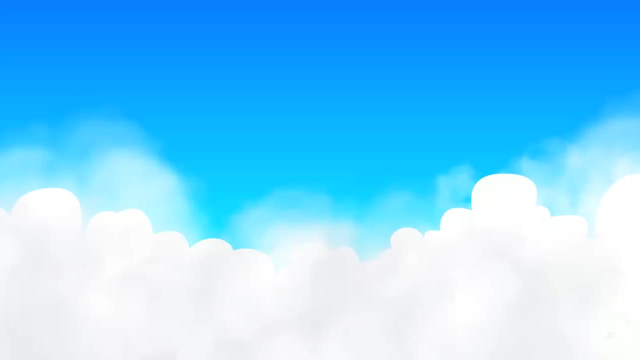 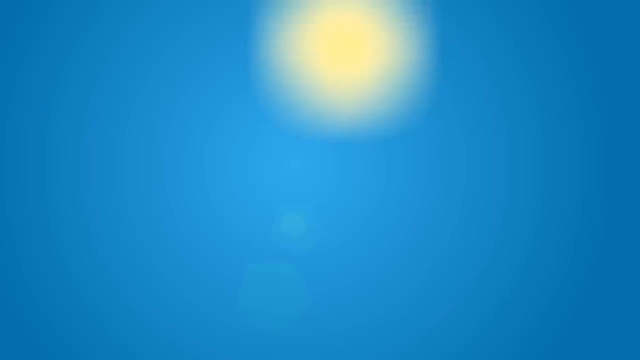 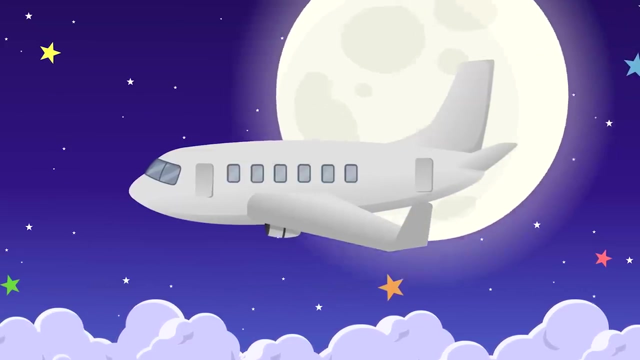 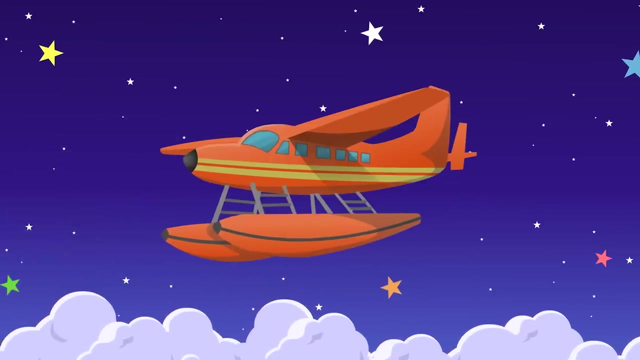 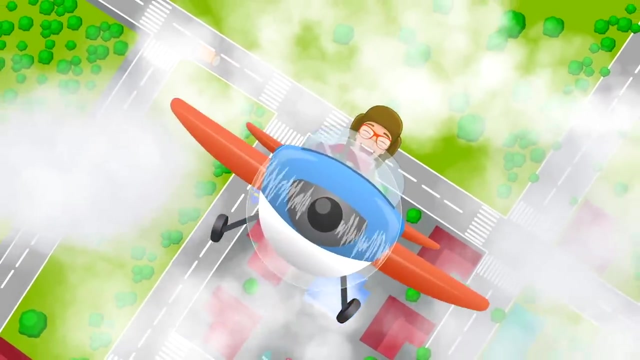 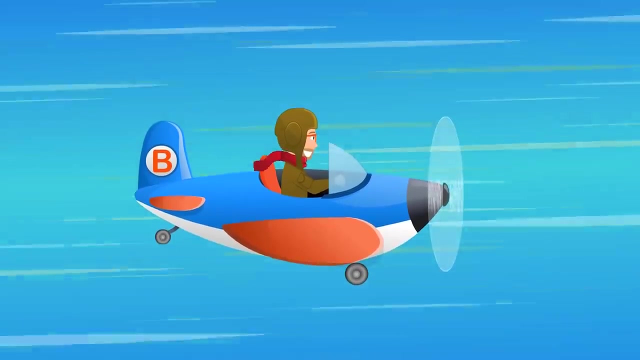 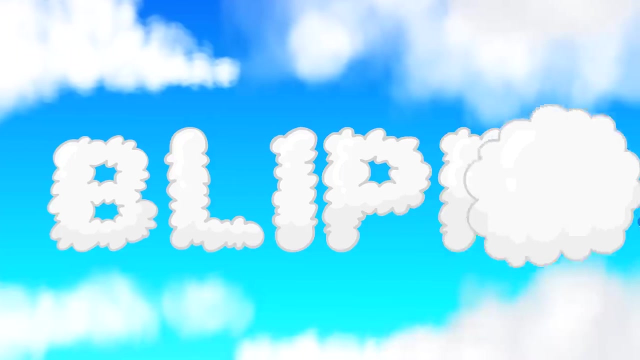 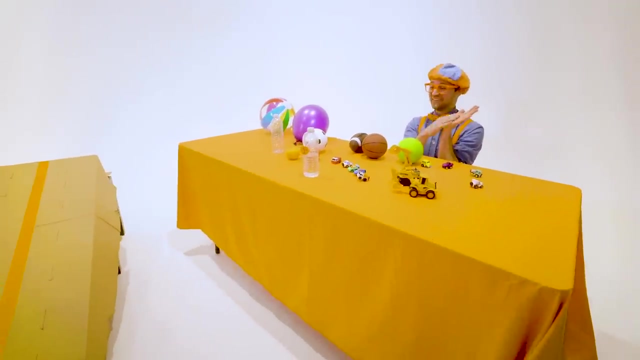 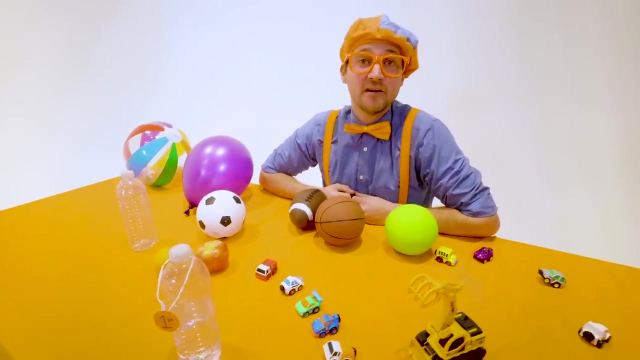 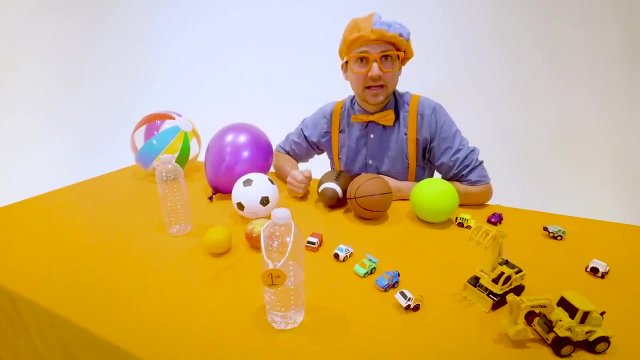 Hey. airplane. Airplanes flying all around the sky. Airplanes- airplanes flying way up high Airplanes. airplanes flying all around the sky. Airplanes- airplanes flying way up high. Airplanes- airplanes flying way up high. 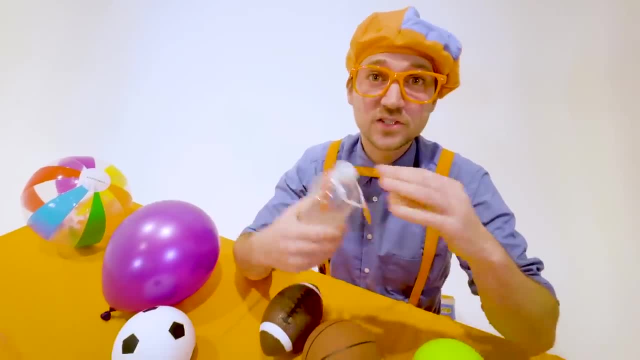 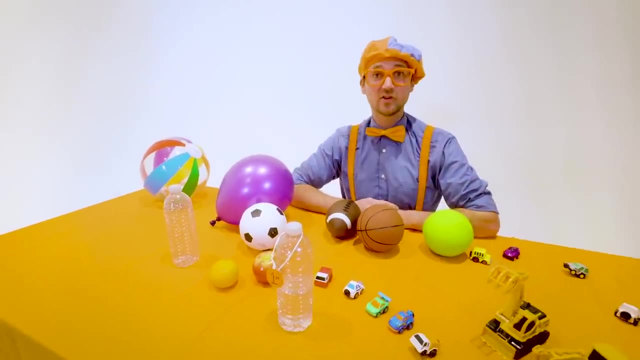 One champion, and today that was water, Wow, Well, this is the end of this video, But if you want to watch more of my videos, all you have to do is search for my name. Will you spell my name with me? 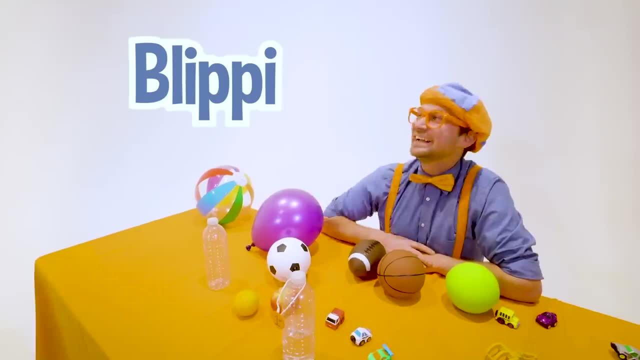 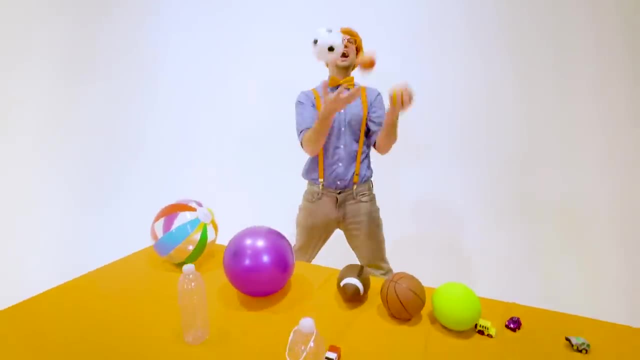 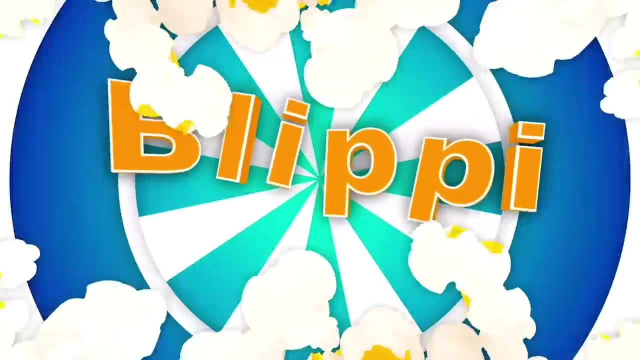 B-L-I-P-P-I- Blippi. Good job, All right, see you again, Buh-bye. So much to learn. It'll make you want to shout Blippi. Hey, it's me, Blippi. I'm just out on a walk. 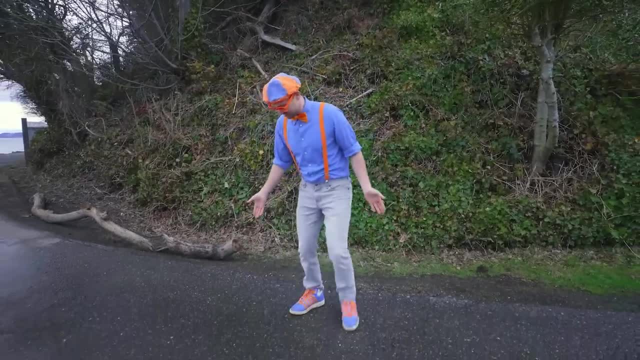 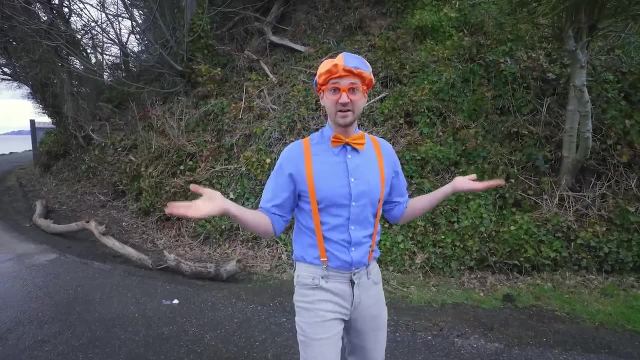 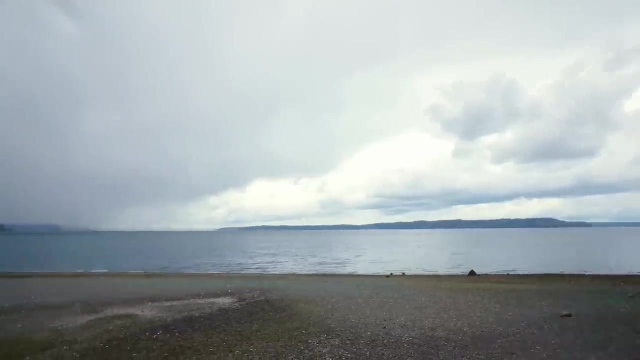 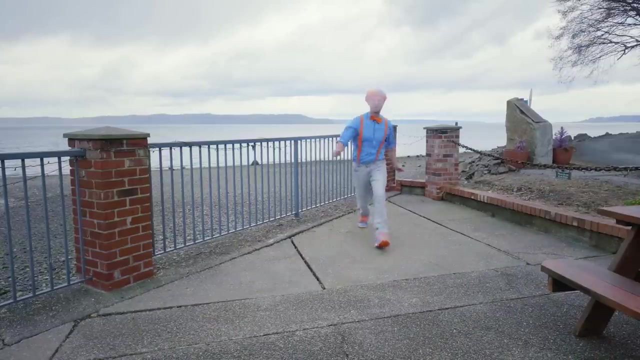 And hey, did you notice the ground is really wet? Yeah, it must have rained here recently. Maybe today you and I can learn about rain weather, rainbows and walks, Ha-ha, Wow, weather can sure be very unpredictable. 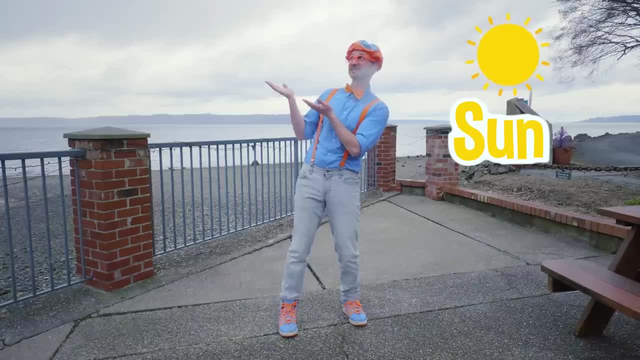 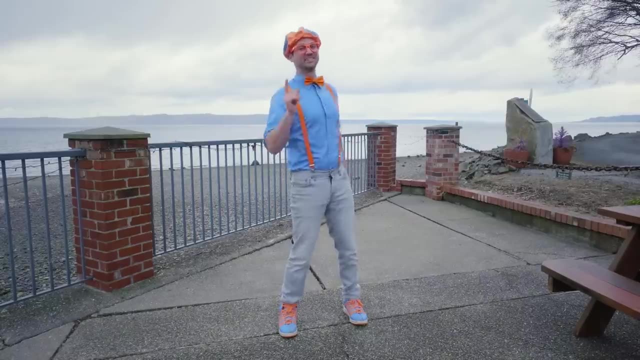 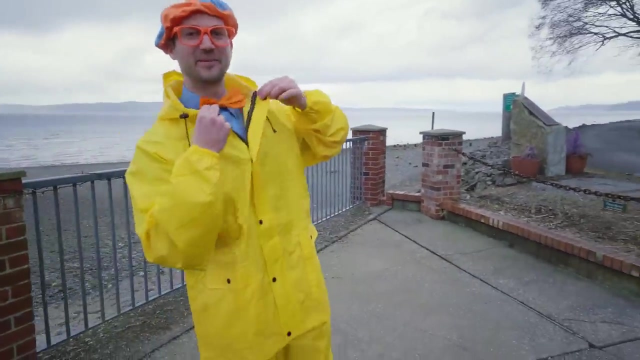 Yeah, Hey, if it's sunny you might need a tank top, If it's cold you might want a stocking cap, But if it's about to rain, you definitely want some rain gear on. Check it out. Yeah, I got my rain jacket on. 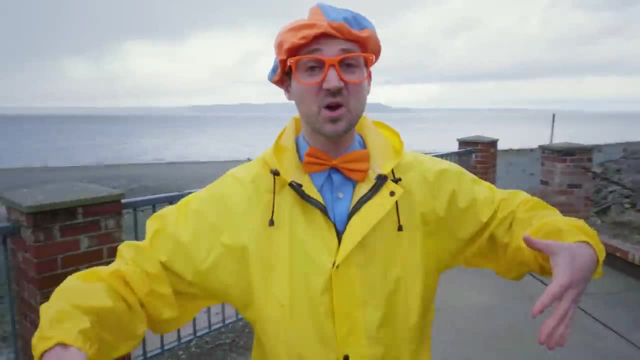 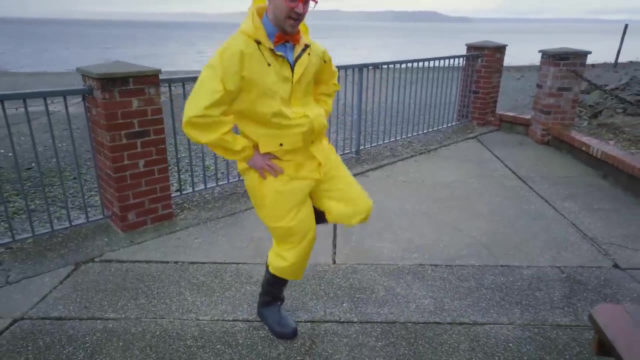 Whoa, it's fully waterproof. So even if it Pours down tons of rain, Yeah, I will stay really dry. And I got my matching bottoms on. Yeah, what color is my outfit? Yeah, it's the color yellow. 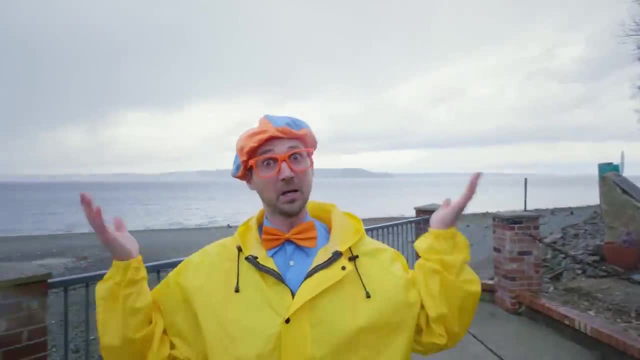 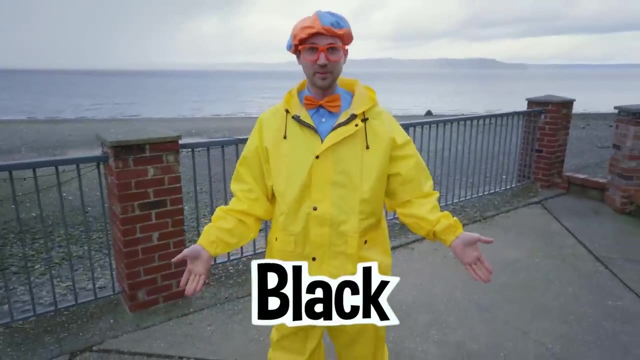 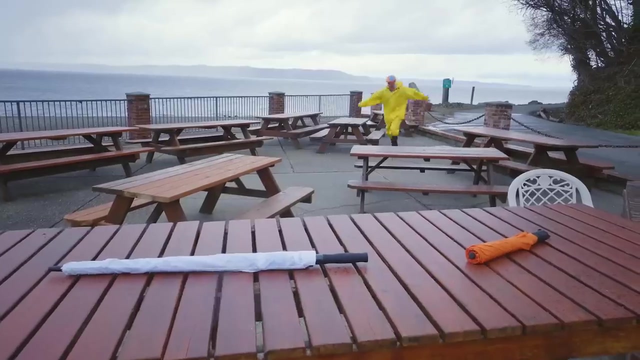 Just like the sun. Where's the sun? I don't know. But hey, check out my boots. Yeah, I have black rubber boots on And the last thing that I'm missing. Yeah, let's go find an umbrella. Okay, let me put my hood on. 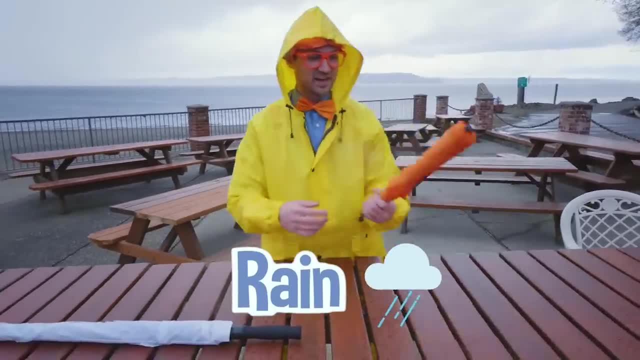 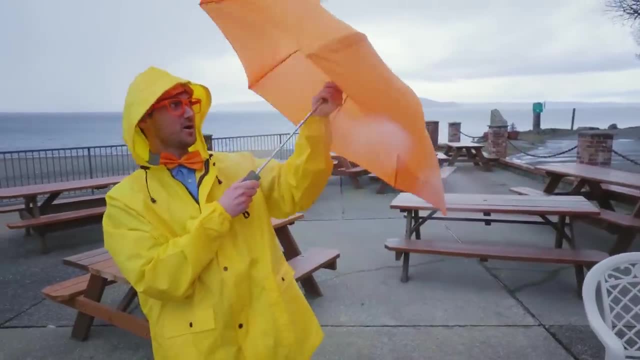 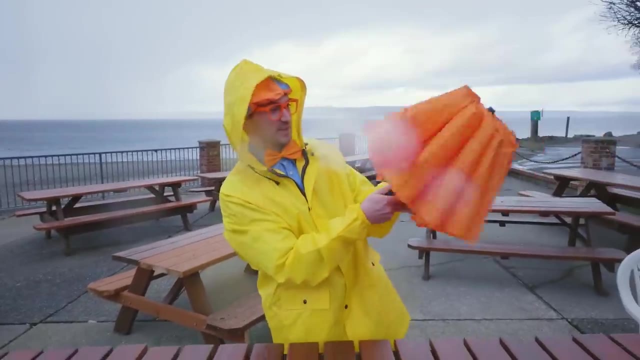 Wow, It's really starting to rain. All right, check it out. An orange umbrella, Open it up. Wow, Now there's no rain hitting me at all. Wow, Okay, let's put this one away. What's this next one? 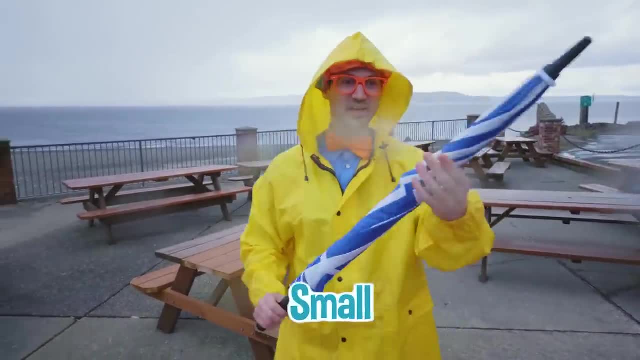 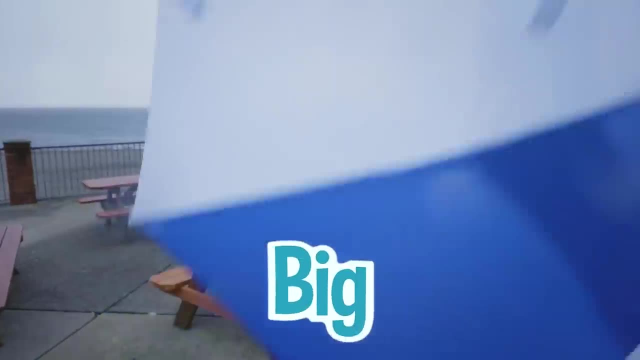 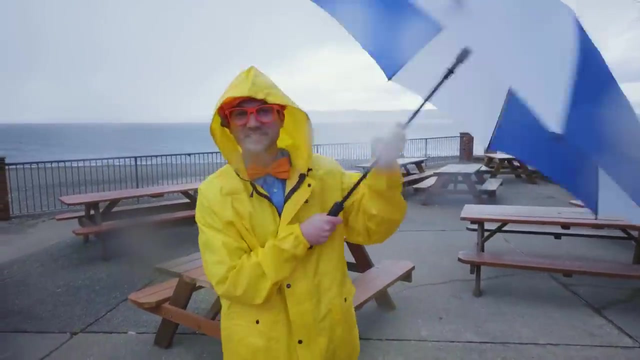 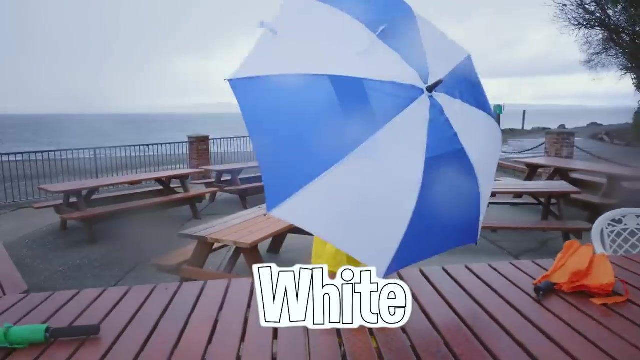 Yeah, The first umbrella Was really small And this one, Whoa, it's so Big. Check it out. What color is this umbrella? Yeah, blue and white. Okay, let me put this down before I fly away. 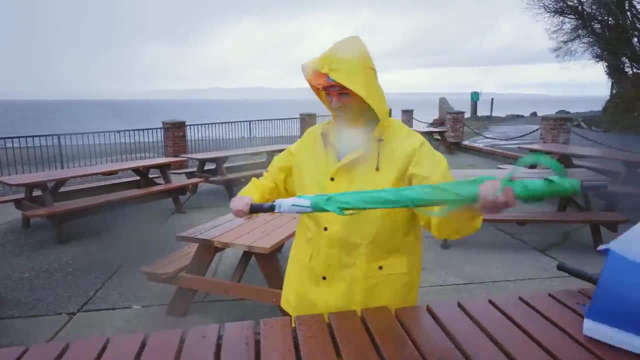 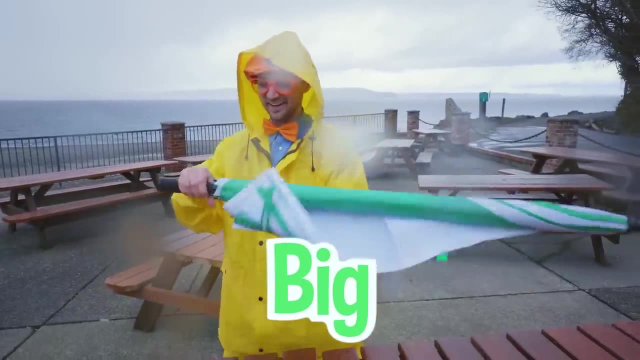 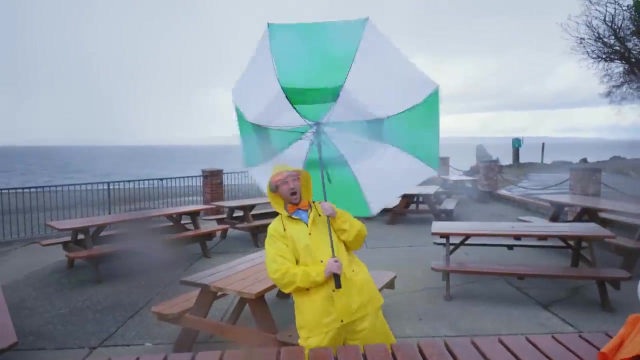 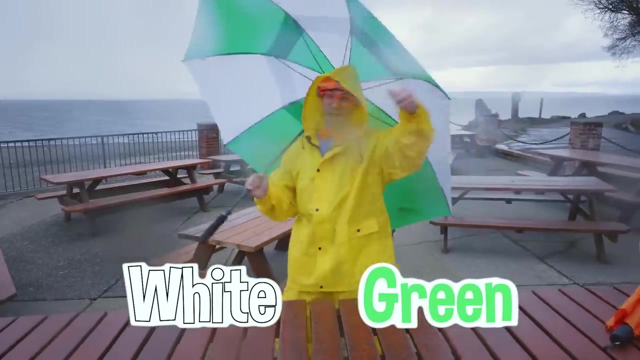 Okay, And for this umbrella. Whoa, Check it out. Yeah, another big umbrella. And the colors of this umbrella are. It is so stormy out. Yeah, it is white and green. Woohoo, Let's go. 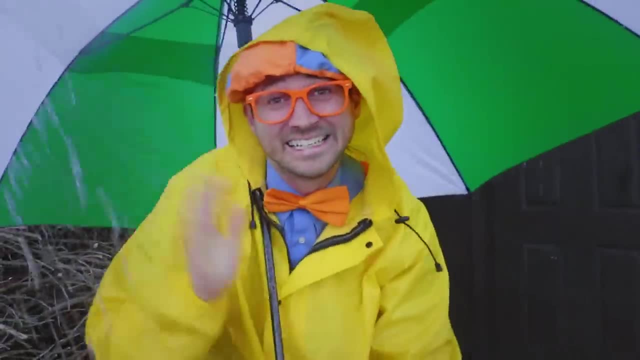 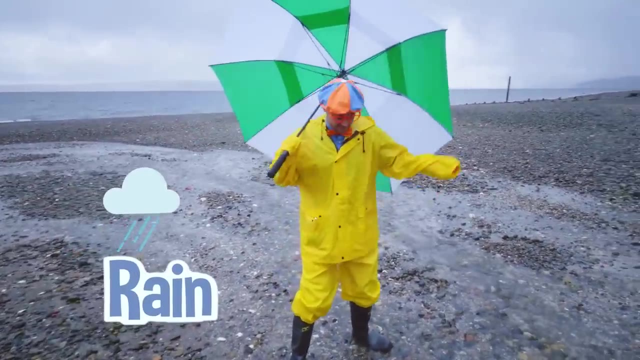 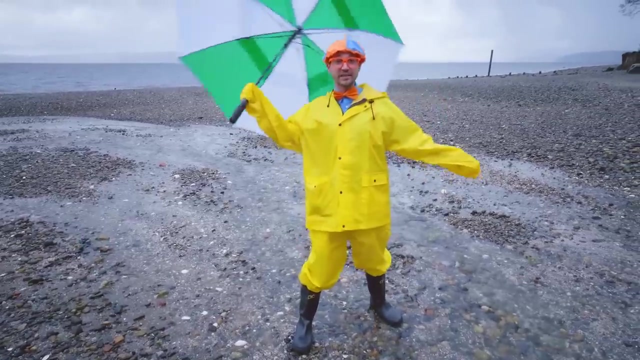 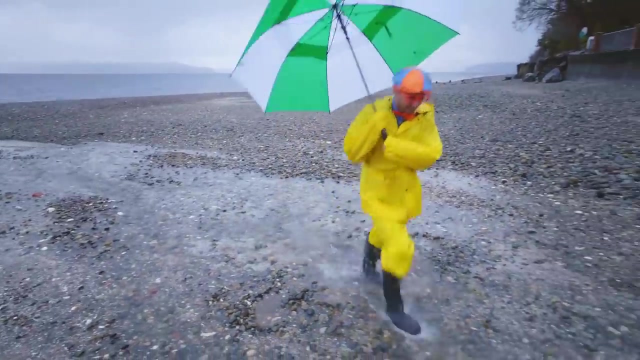 Wow, I love the rain. The cool thing about rain gear is you can even splash in the puddles and streams that were created by the rain And you won't even get wet. Hahaha, Woohoo, Woo, Woo, Woohoo. 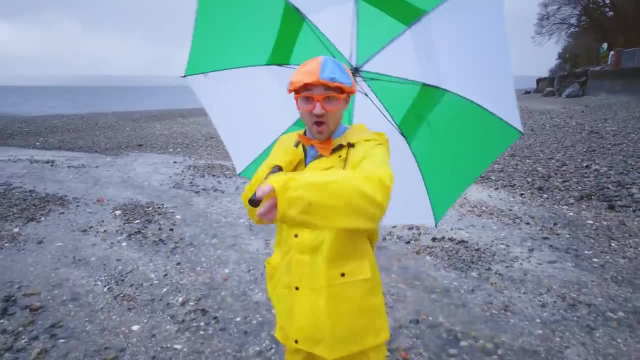 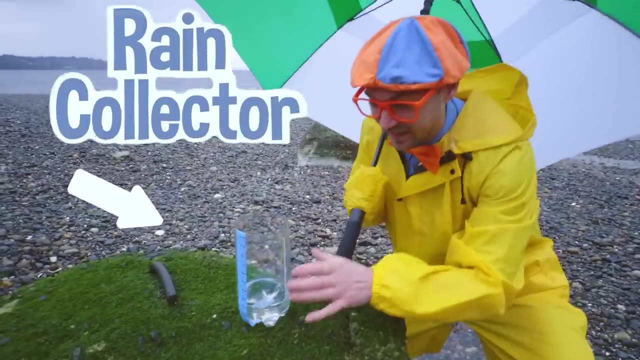 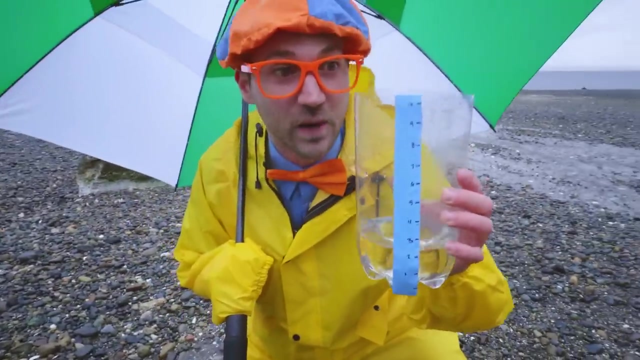 Yeah, Yeah, Hey, check it out. Look back here. Look back here. Wow, Do you see this? Yeah, this is my rain collector. I set this out earlier, before it started to rain, And then all this rain collected from the top. 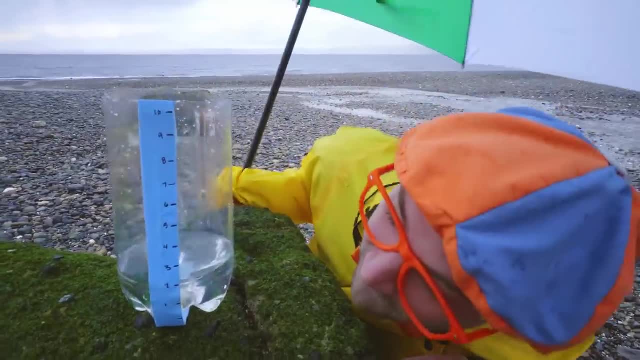 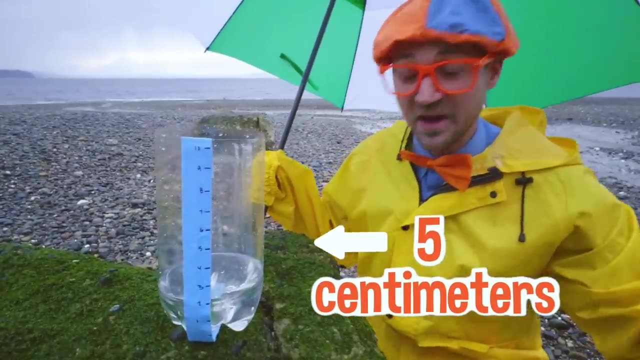 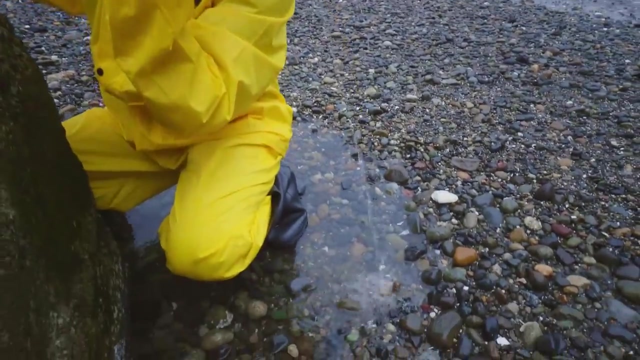 Do you see how much it says Wow? Yeah, it says about two inches. Yeah, that's just over five centimeters of rain. Wow, That's a lot of rain. Okay, I'm going to pour it back: Yep, onto our planet Earth. 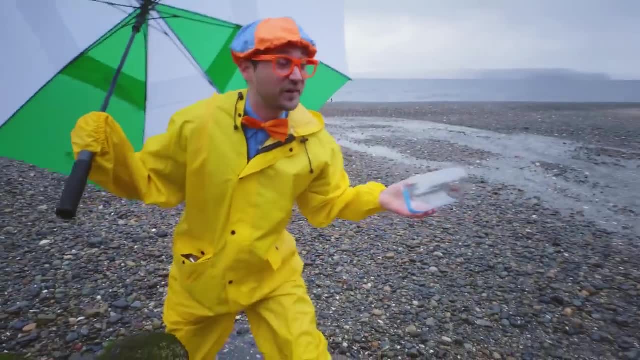 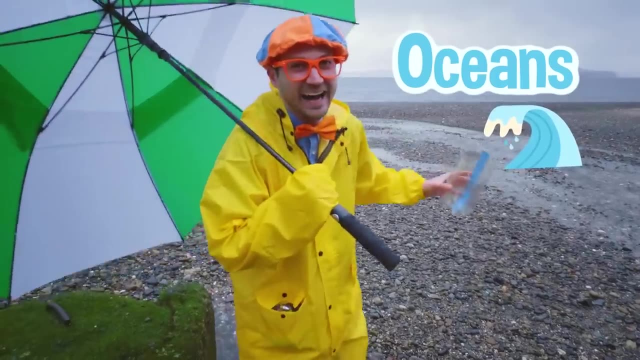 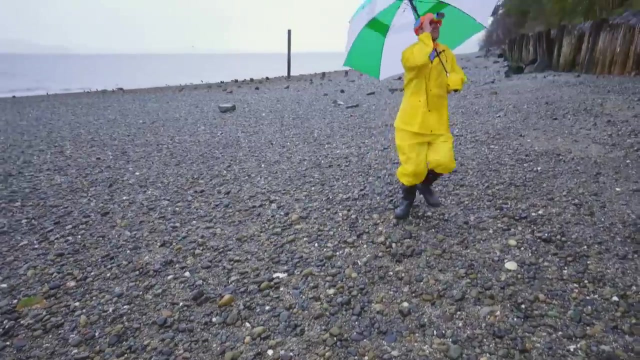 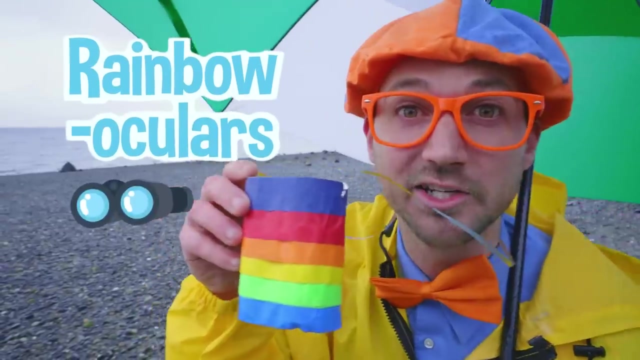 Because when the rain falls on our planet, it's really good for it. It helps keep all the plants nice and moist and our oceans nice and full. Woohoo, Hey, check it out. Yeah, these are my rainbow oculars. 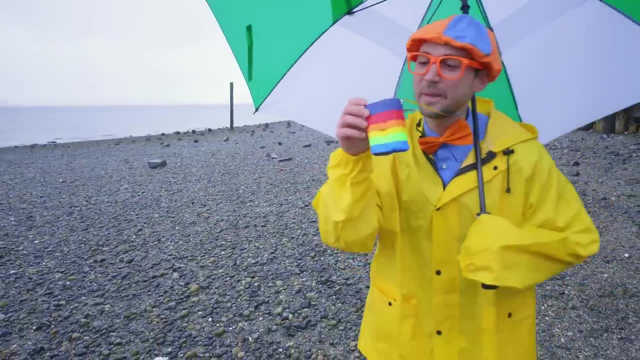 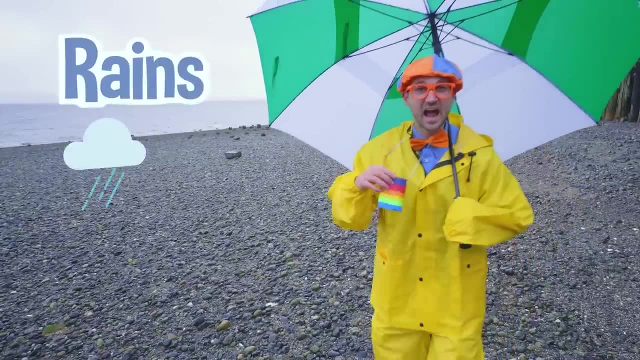 Yeah, isn't that cool. Yeah, they're the colors of the rainbow. Have you ever seen a rainbow before? Yeah, they love to come out after it rained. Yeah, a rainbow is an arch of colors made by light and water. 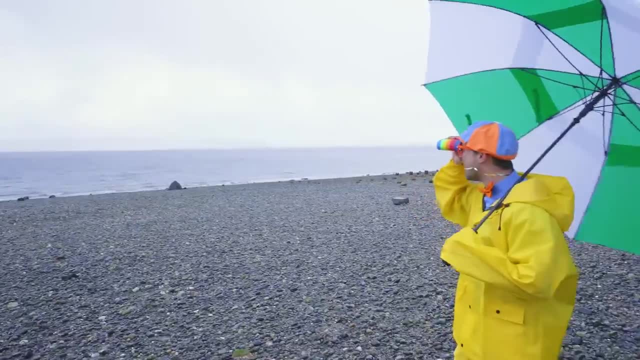 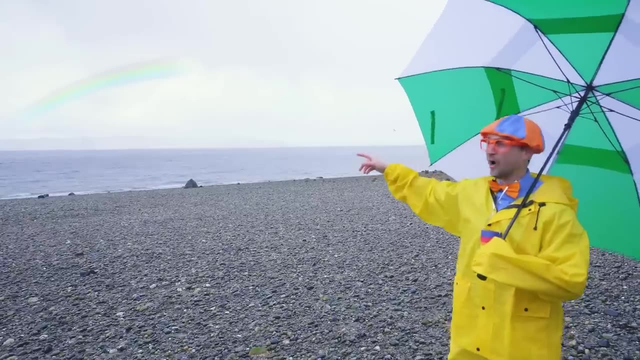 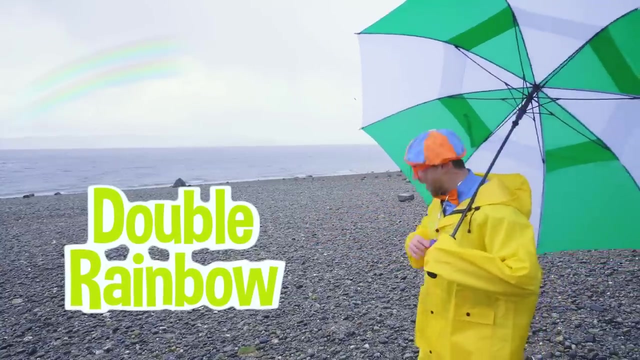 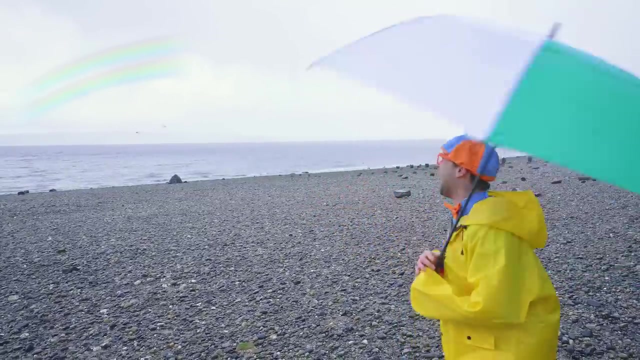 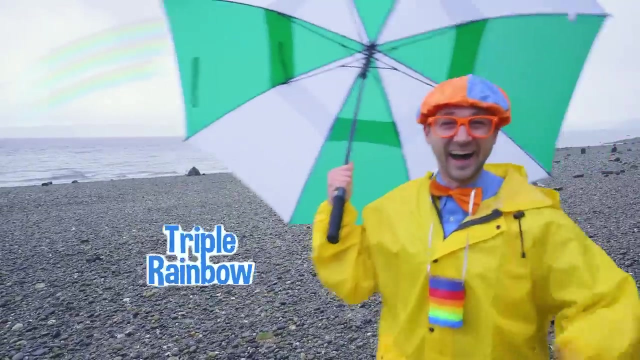 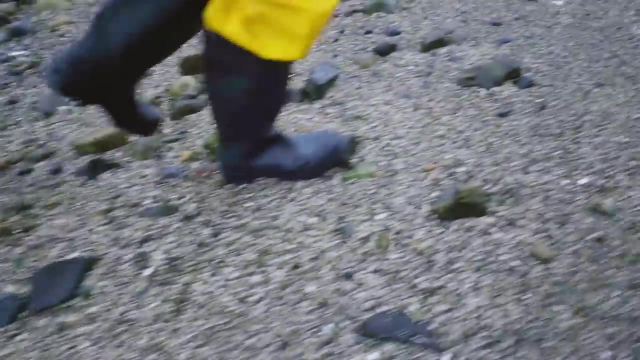 Let's see if we can find one. Oh, Oh, Oh, Oh. A rainbow, Oh A double rainbow. Oh, Oh, Oh, It's full on. Even a triple rainbow. Woohoo, Woohoo, Woohoo. 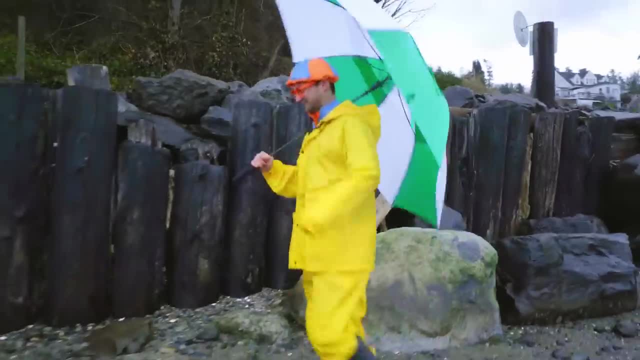 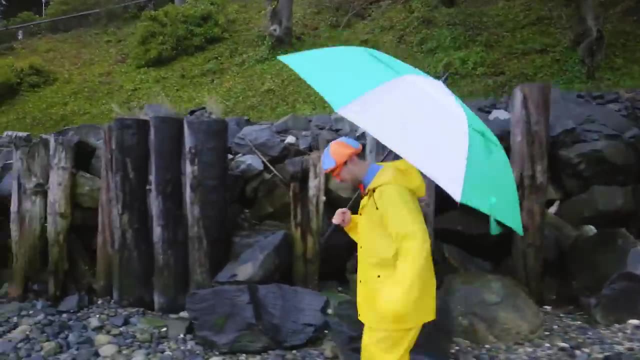 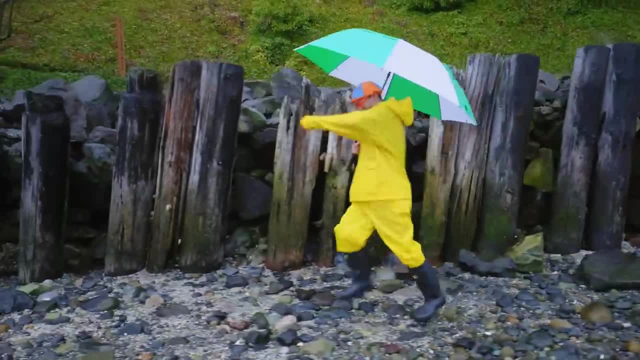 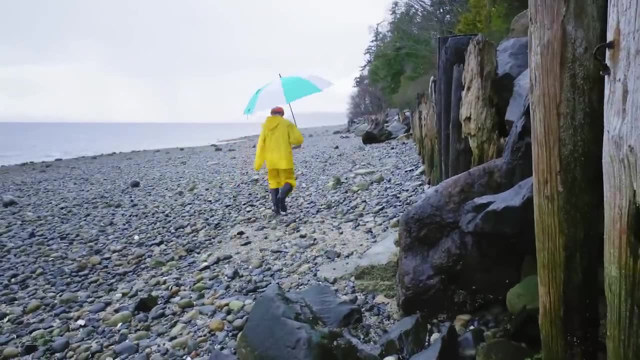 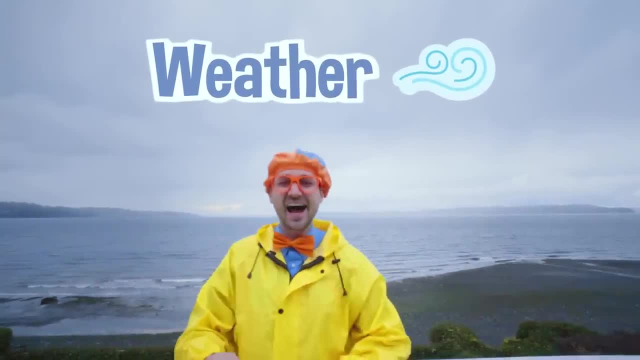 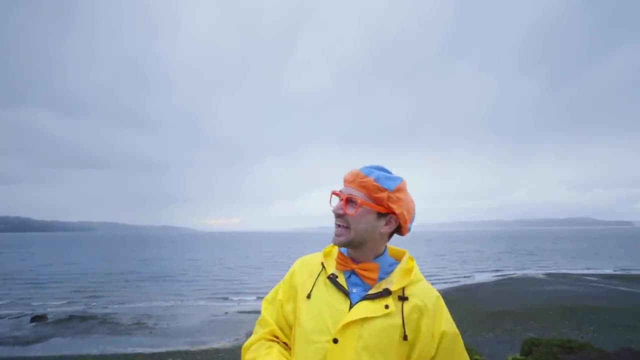 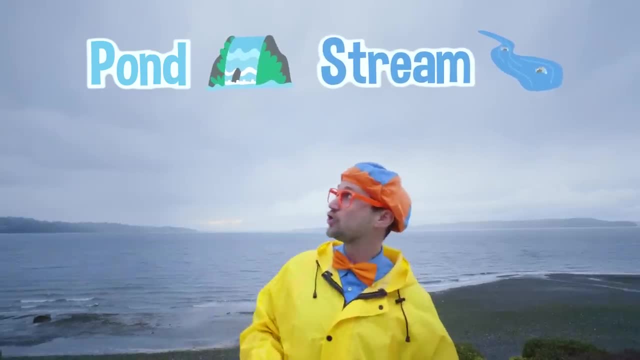 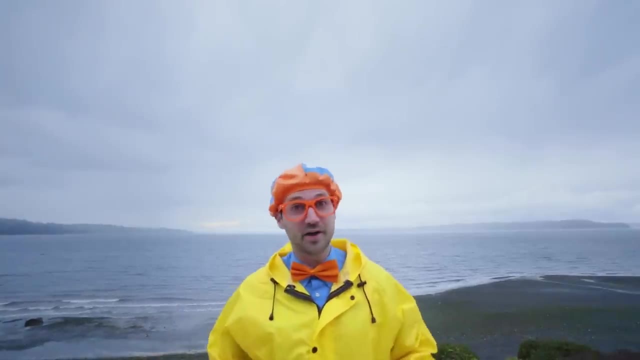 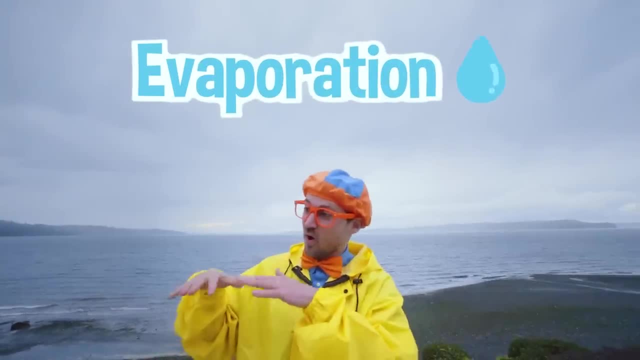 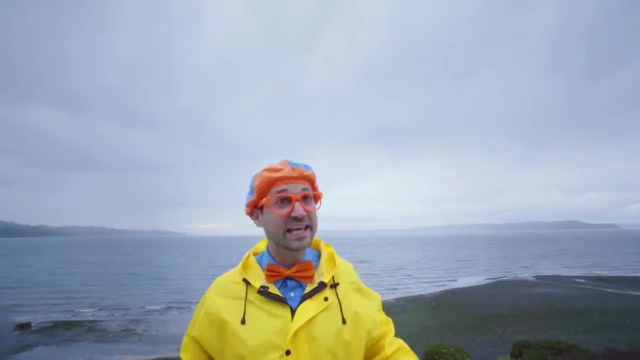 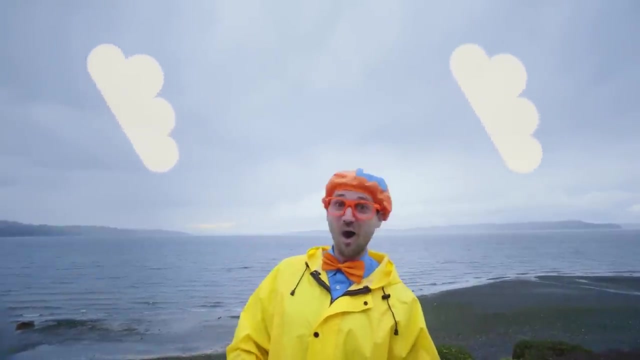 Woohoo, Woohoo, Woohoo, Woohoo. Water becomes these little tiny particles and goes up in the air. Yeah, it turns into a gas. It goes up in the air and then turns into some clouds. Whoa. 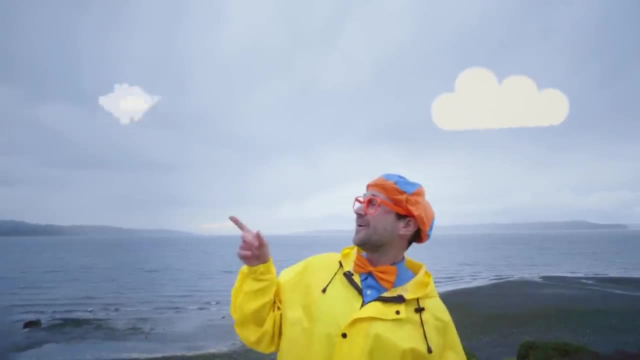 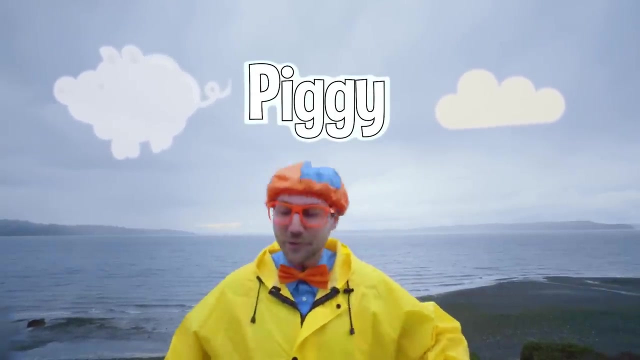 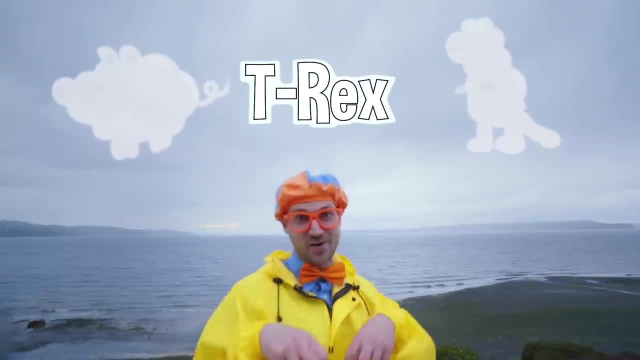 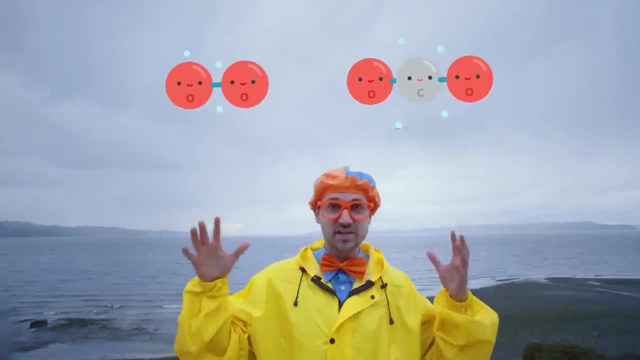 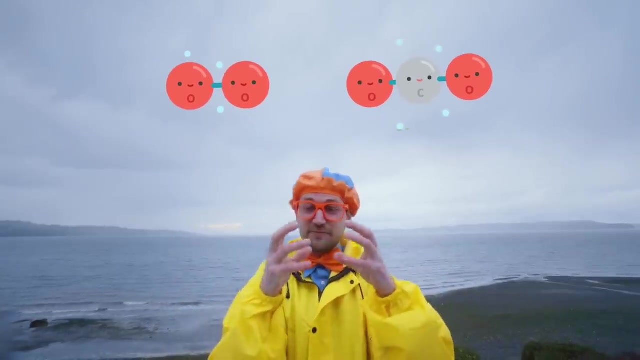 That cloud looks like a T-Rex: Rawr, rawr, Wow. And then all this gas water starts to come closer and closer and closer, Yeah, and those clouds start to form into liquid water again, Yeah, and then rain starts to fall. 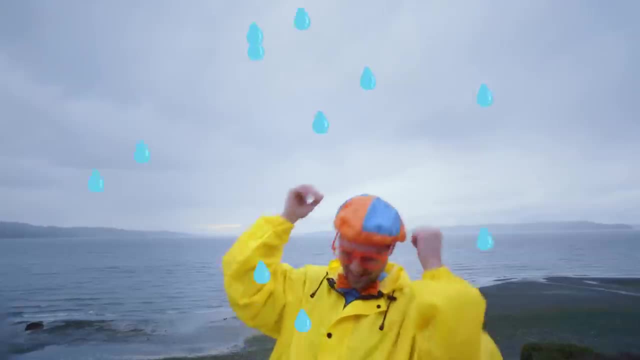 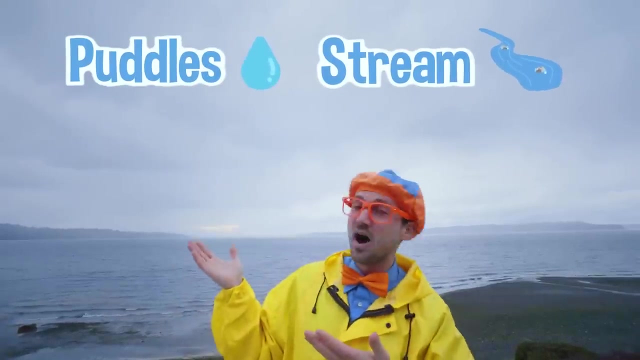 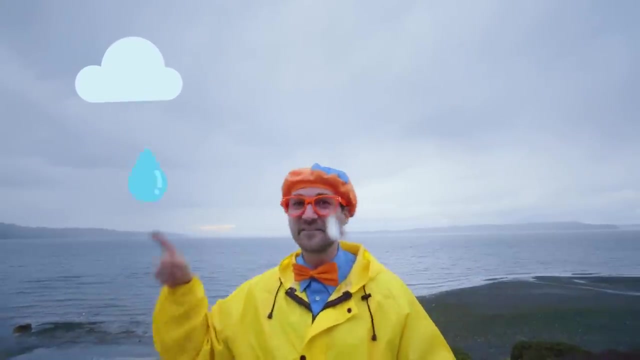 Whoa, Yeah, it's raining, Whoa. And then they create puddles and streams and ponds and the water goes back into the ocean again, And then the cycle goes over, and over and again and again. Wow, that water cycle is so great. 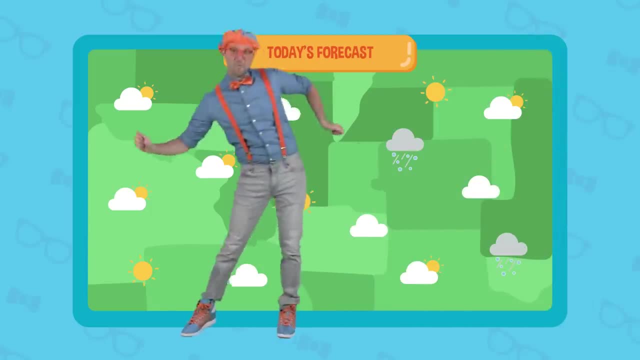 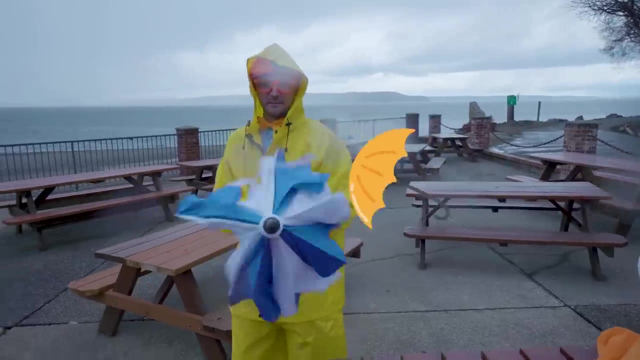 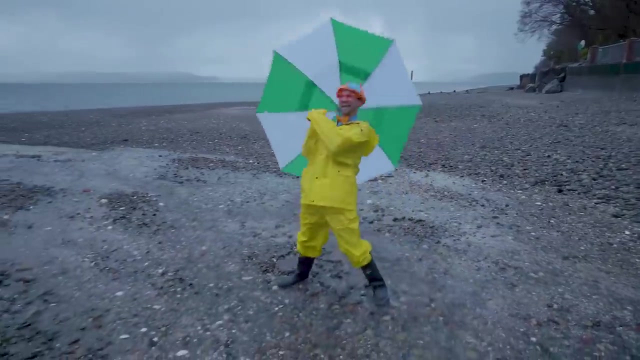 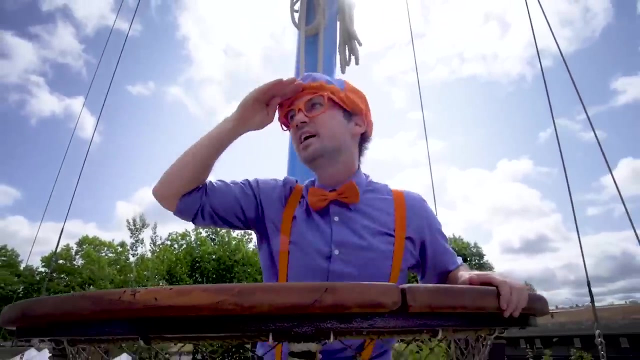 Woohoo, Today's weather forecast: sunny skies in the morning, followed by storms in the afternoon. Don't forget your umbrellas. Don't forget your umbrella. The morning looks nice: lots of sunshine, Clouds of white and a bright blue sky. 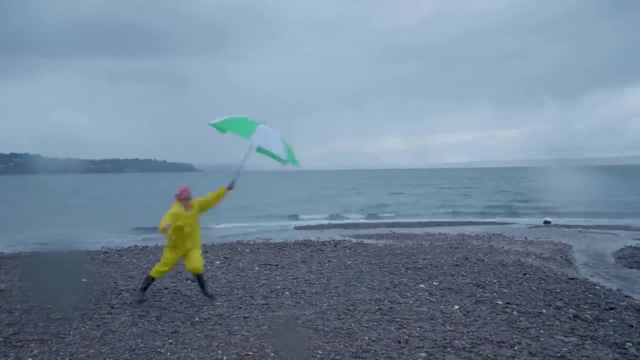 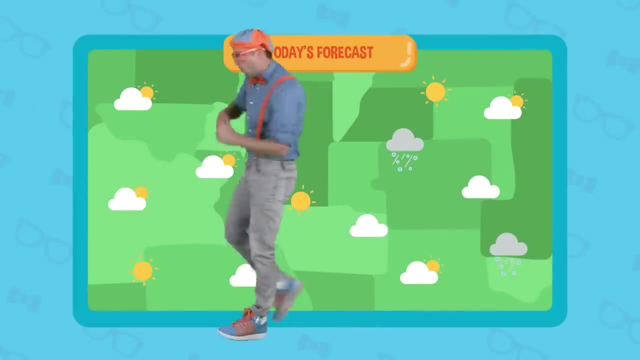 But the sky's turning gray, there's wind and some rain. It looks like it's gonna be a stormy day. Weather weather, all kinds of weather: Black, sunny, breezy, cloudy, warm, sunny, Blue skies, discovery retour. 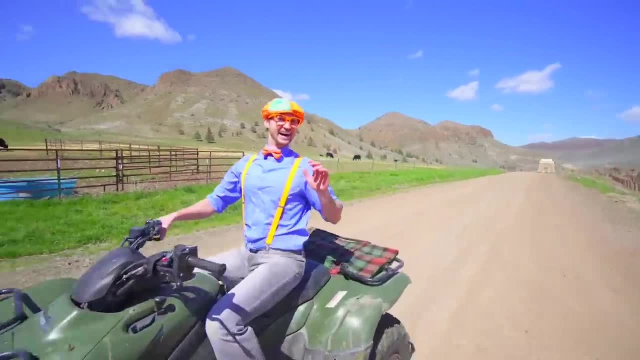 Not only the wüns near me with my cloud, but also currents. It's gonna get a little warmer when there's not a little nice temperature when things circle south of me. Cool, breeze, pleasant days, Weather, weather, all kinds of weather like windy, rainy, stormy, hot. 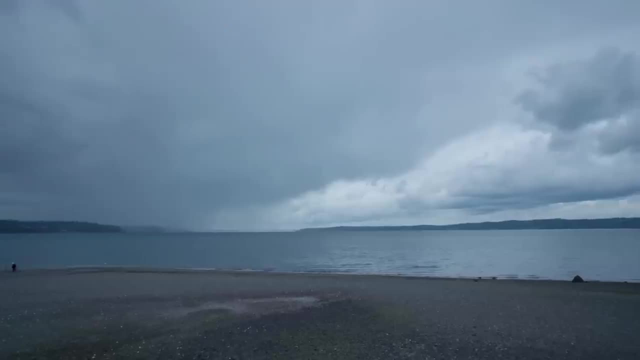 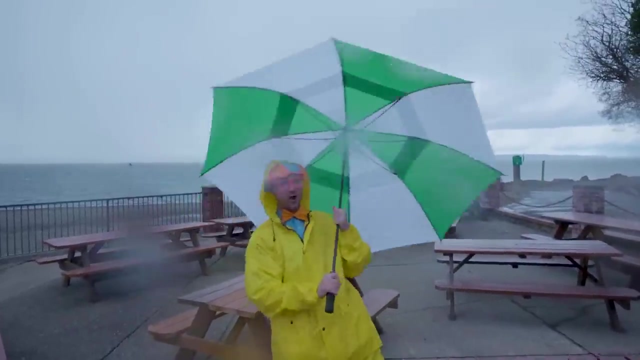 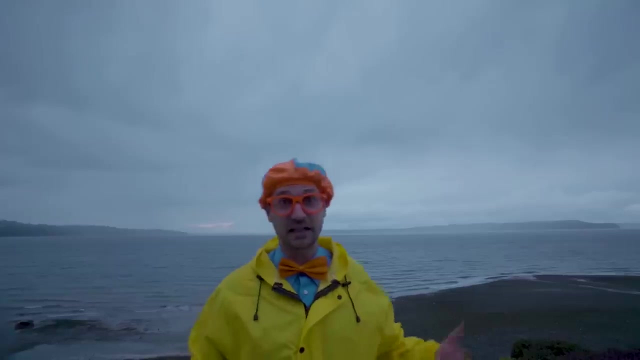 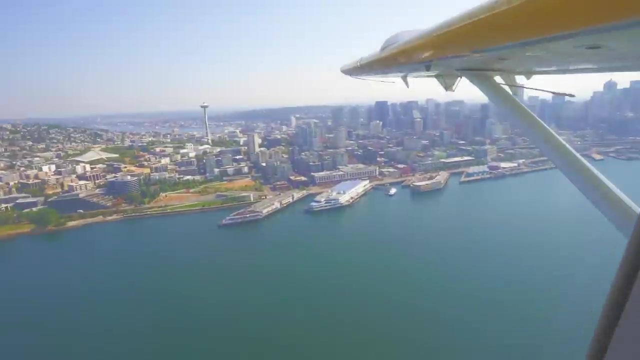 muggy days, A lightning bolt, that thundering sound. There's a storm coming any moment now. Tornadoes, hurricanes and floods. Sometimes weather can be dangerous Weather weather, all kinds of weather, like sunny, breezy, cloudy, warm, pleasant days. 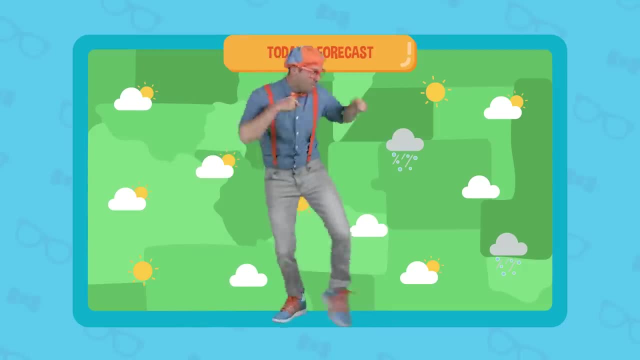 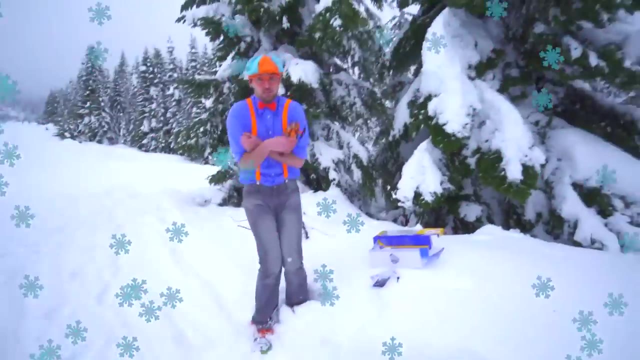 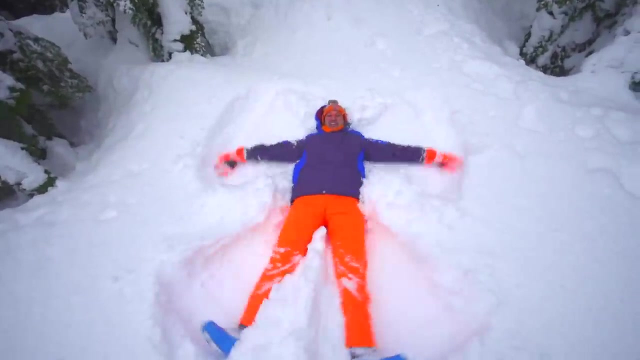 Weather weather. all kinds of weather like windy, rainy, stormy, hot, muggy days, And when it's really really cold, snowflakes will fall from the sky, Everything goes quiet and everything is covered in white. 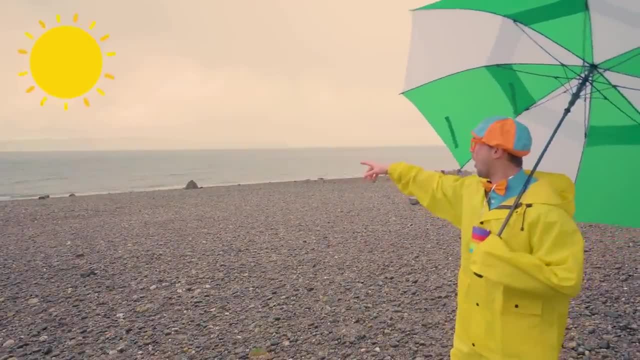 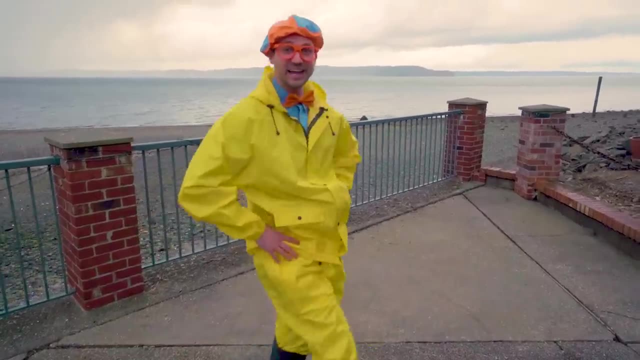 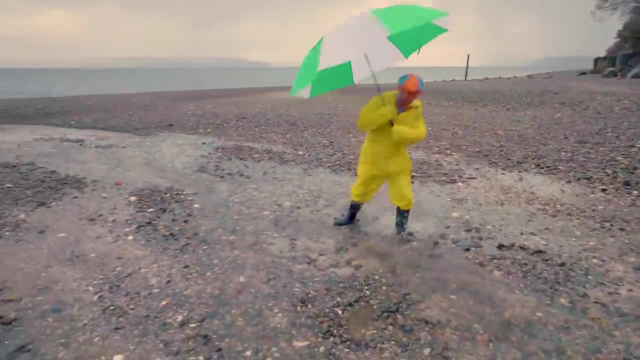 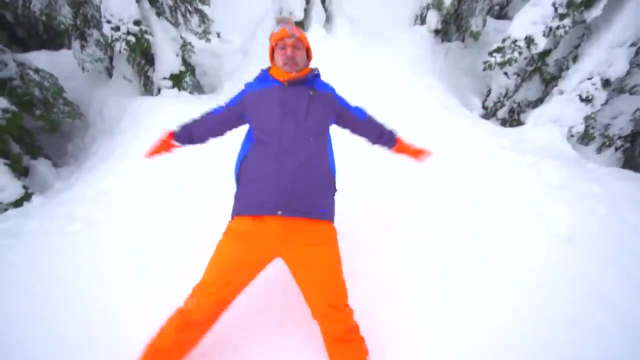 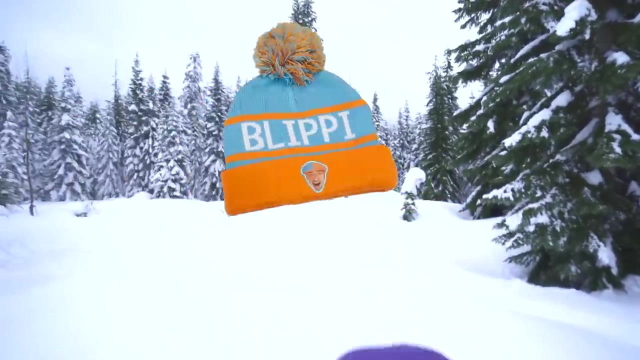 Hey, The rain has stopped and the sun's shining again. Weather weather- all kinds of weather like snowy, icy, blizzard, cold, frigid days. Weather weather- all kinds of weather like sunny, rainy, stormy, hot, muggy days. 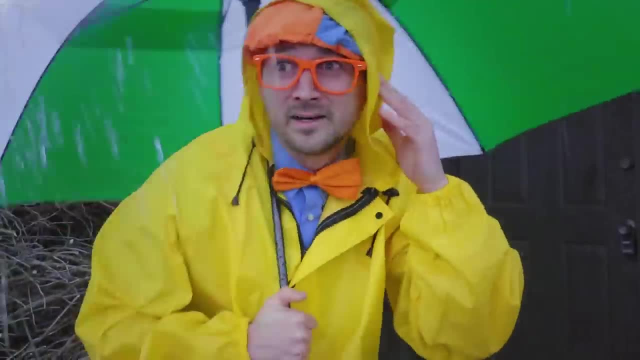 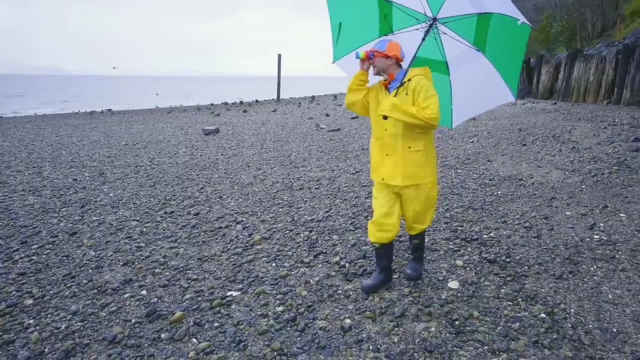 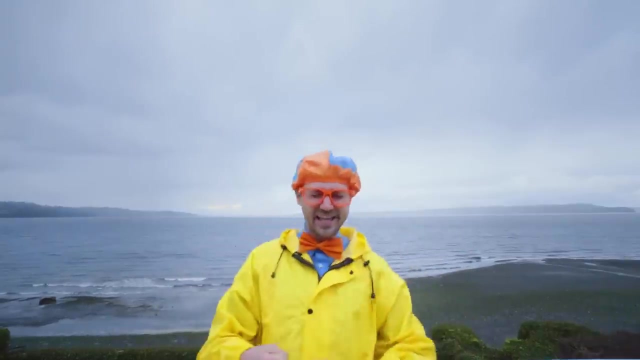 Well, this is the end of this video, But if you want to watch more of my videos, all you have to do is search for my name. Will you spell my name with me? Ready B-L-I-P-P-I. Blippi, Good job, All right, See you later. Buh-bye. 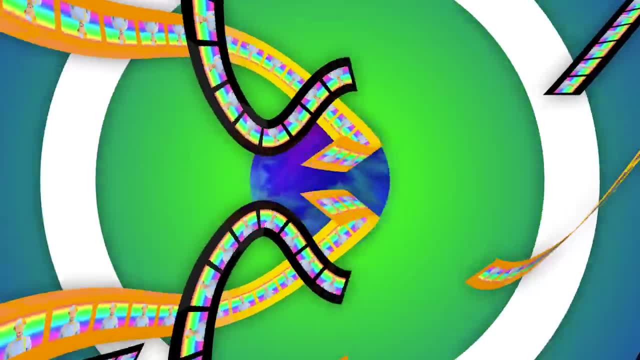 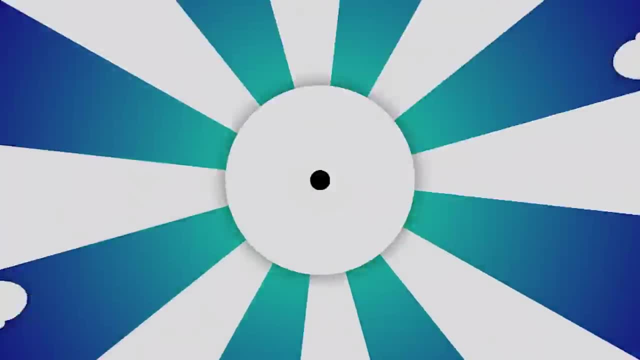 Blippi. Come on everyone, Let's make learning fun. Blippi, Blippi. So much to learn about. It'll make you want to shout Blippi.